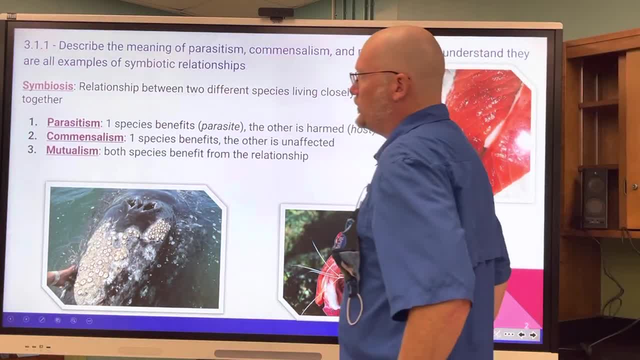 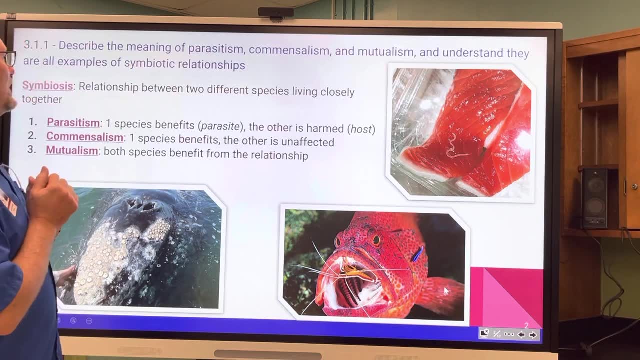 All right. so the first part wants us to describe the meaning of parasitism, commensalism, mutualism, and understand. they are all examples of symbiotic relationships. Now, if you took biology, you already learned about this. I do believe. 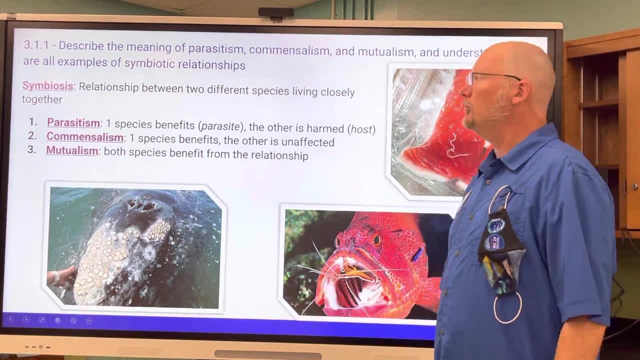 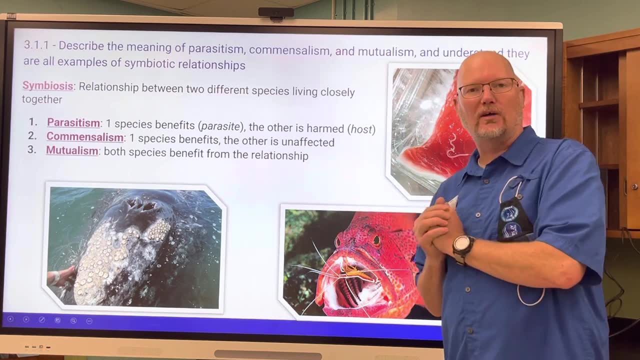 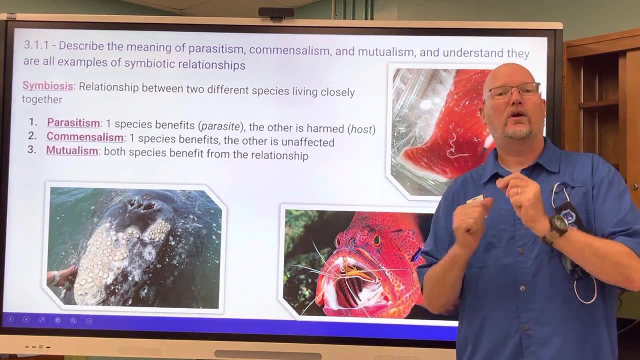 You may have even touched upon it and remember it from middle school, but we're going to relate it now and apply it to these concepts, to marine science. okay, So we know that symbiosis is a relationship, a close relationship, of two organisms. 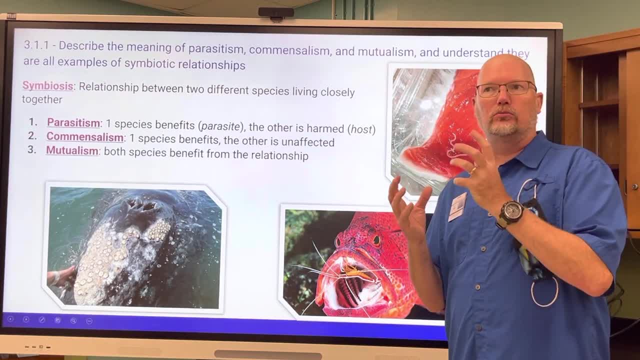 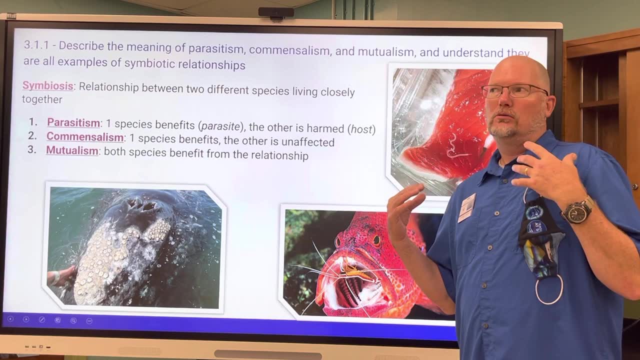 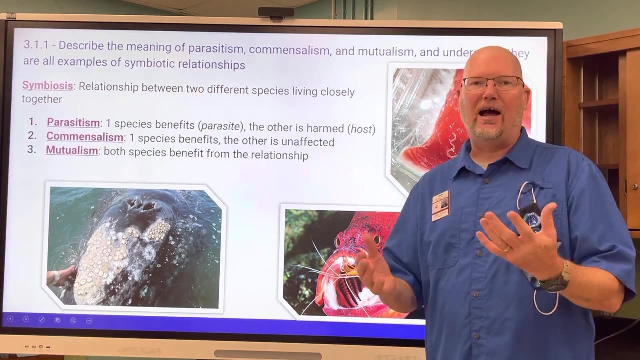 that are living, you know, very either so close to each other that they're on one's, on the other or right next to okay, And so there's examples from all over the and all different kinds all over the world. 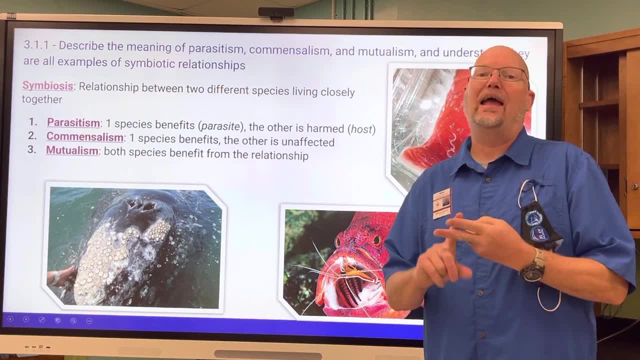 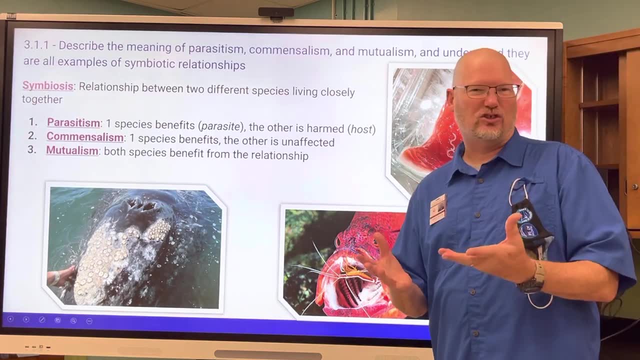 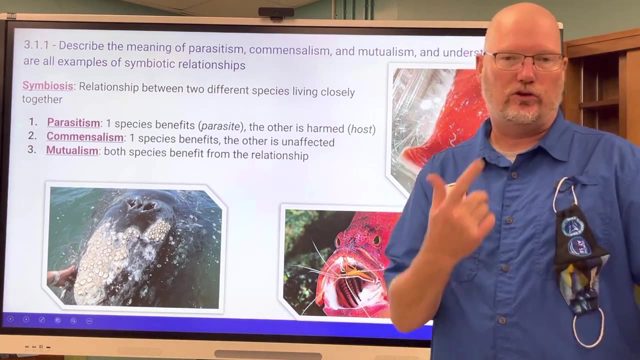 There are bird, there are parasites, there are plant parasites, and then there are these type types of parasites. okay, Or symbiotic relationships. I was specifying one- but, generally speaking, symbiosis, You have a symbiotic relationship with you. You have a bacteria that live in your gut and on your skin. 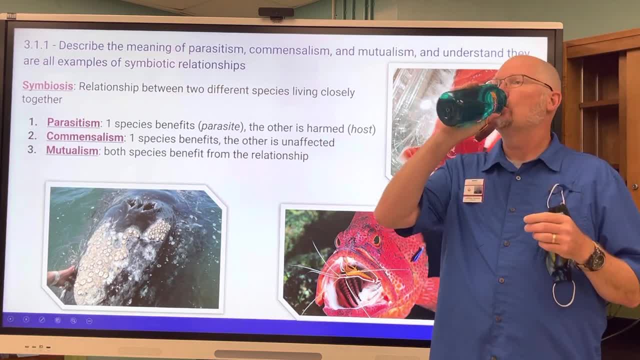 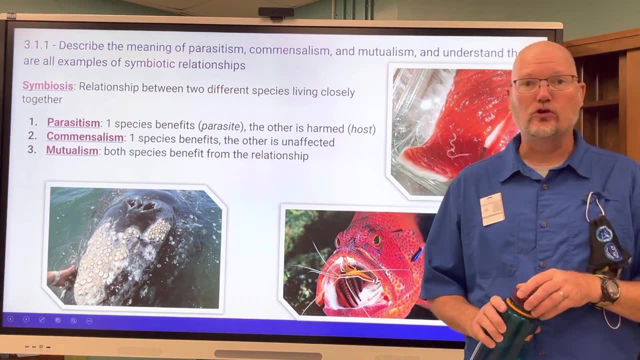 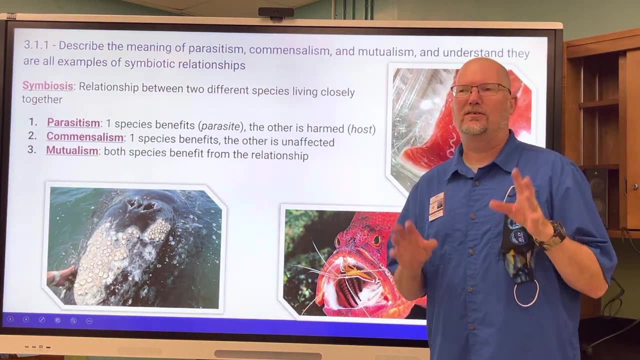 and in your mouth and your nasal passages, under your fingernails. and no, you can't scrub them all away, Nor do you want to. We can talk about that some other time. You have mites that live in your eyelashes and other places. No, you can't scrub them all the way. So parasitism is where one species benefits and the other species is harmed. So an example would be this worm living in the muscle tissue of a fish. That's never good If you have something that's living in your muscle tissue. 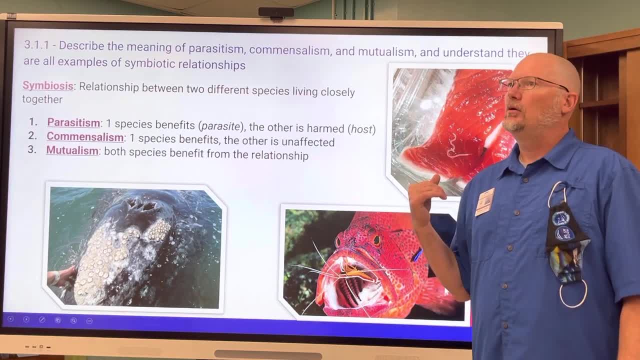 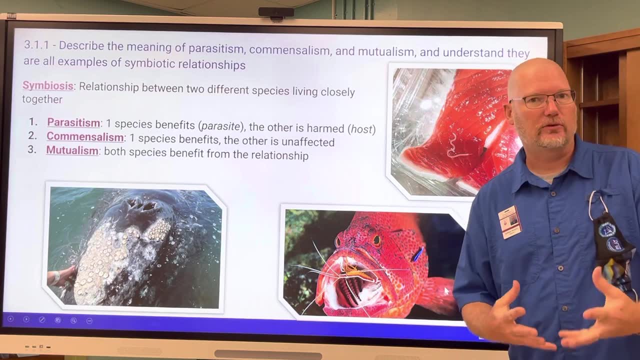 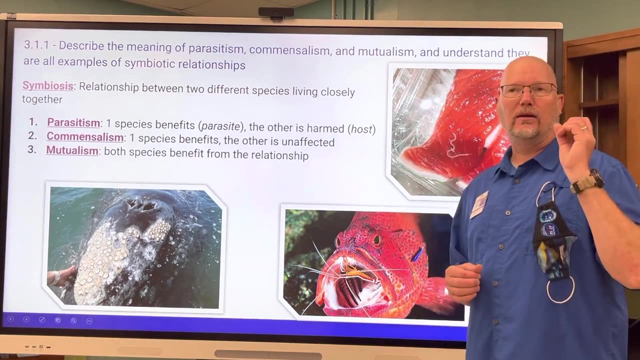 or your intestines, typically other than the bacteria that help us break our food down, We're talking about marine organisms here, like worms. I'm talking about worms. in this case It's typically bad, always okay. Commensalism is when one species is benefited and the other species is neither harmed. 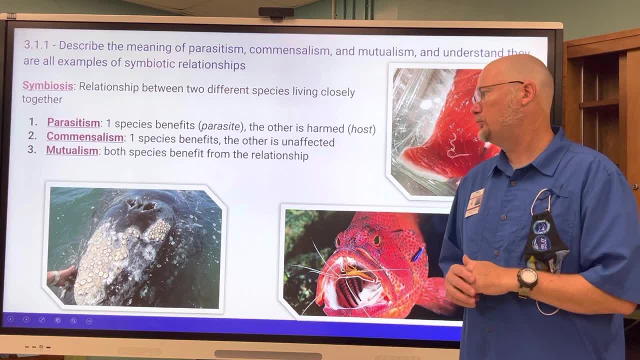 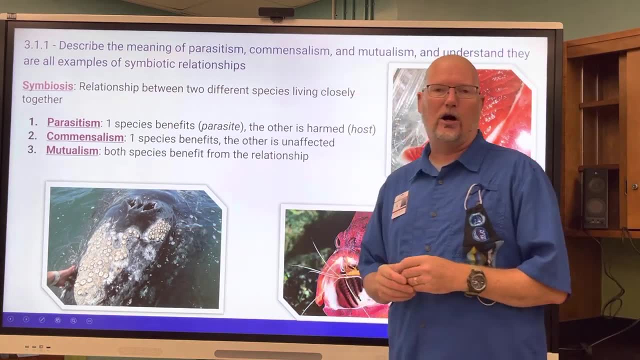 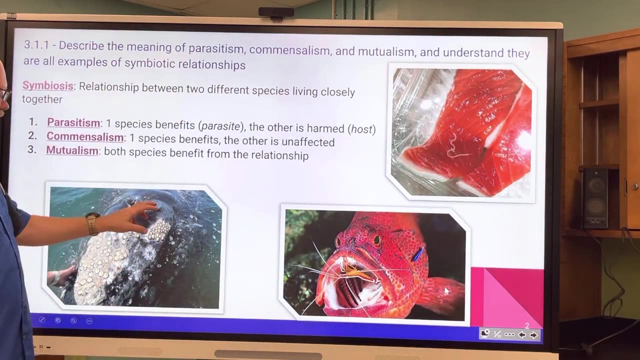 nor benefited. It's just kind of neutral for that, other species unaffected. And so that would be the barnacles on a whale. okay, Now, I guess sometimes if the barnacles can grow maybe too close to the blowhole or to 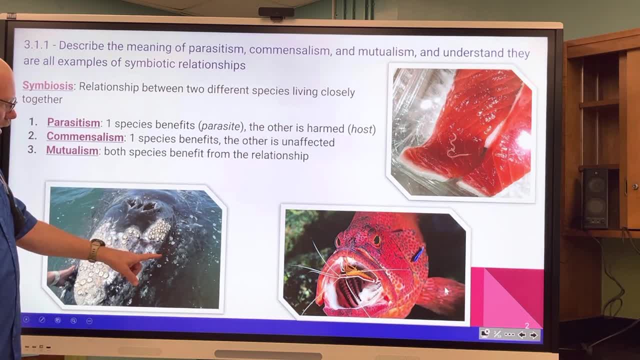 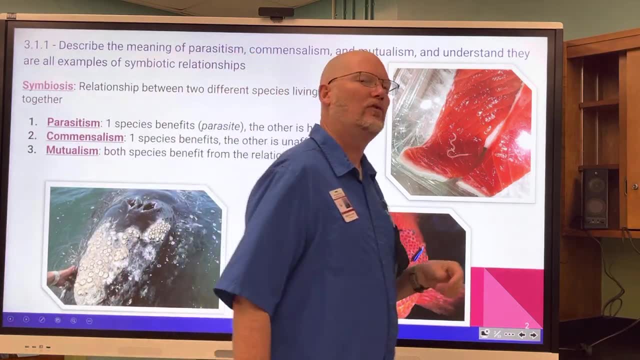 and this is a gray whale. or to the eye or even maybe the mouth, they might become a problem, but whales are smart enough to know how to scrape them off on the bottom. There's videos of that on YouTube. You can see whales doing that. 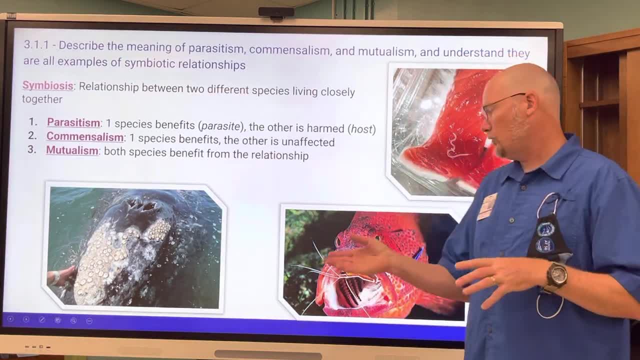 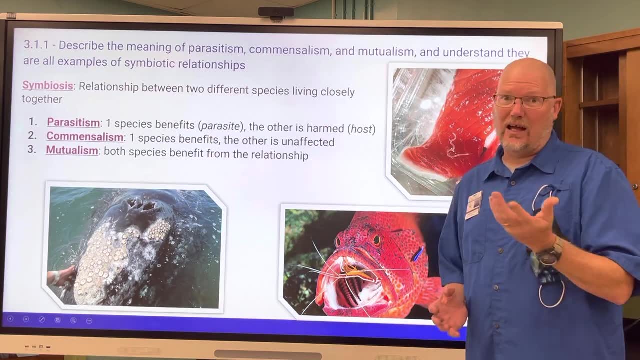 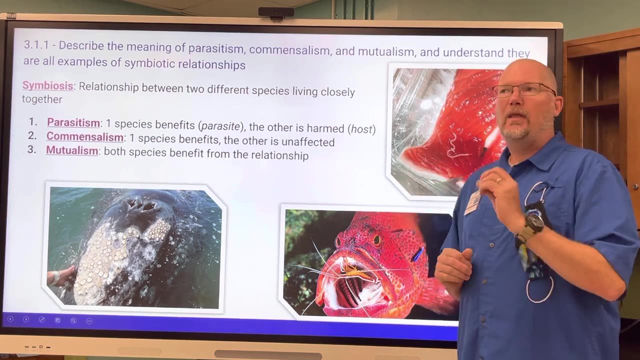 And then mutualism is when they both benefit. So here you have a cleaner shrimp and a fish that is would normally eat that shrimp, but in particular areas- areas on the reef- the fish will line up and it's really quite amazing, And the shrimp and other little fish will come in and they'll go in the mouth. 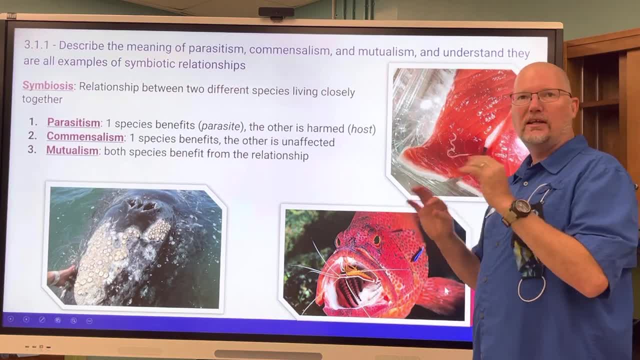 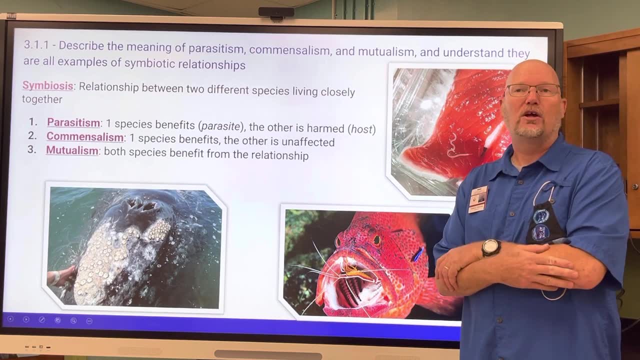 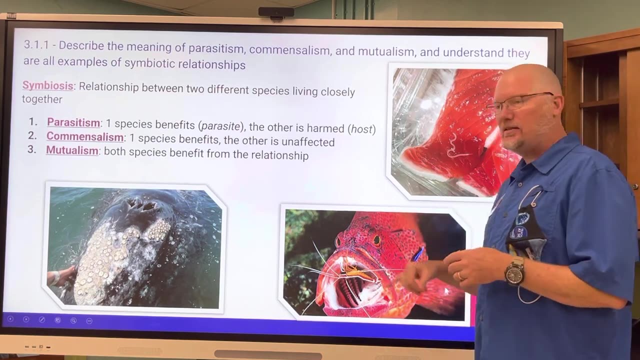 and gills and sharks too, and they'll clean all the parasites and dead pieces of fish or whatever and things like that off of the bigger fish. And the fish just lets it do it because it knows instinctively that it's being benefited, And if it were to eat that shrimp then it would lose that benefit. 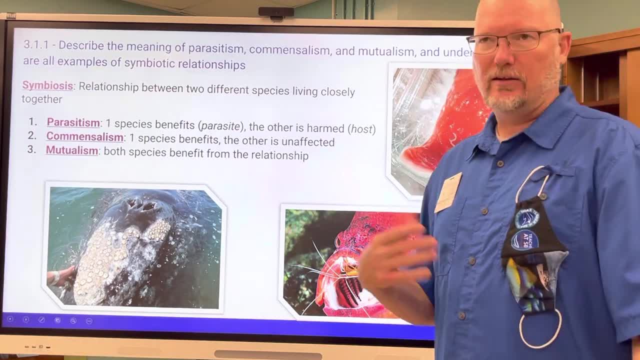 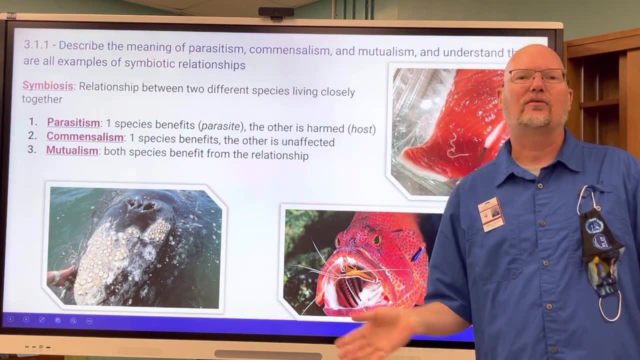 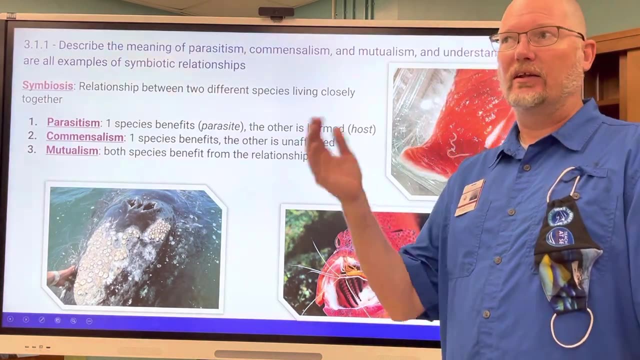 It's rather, quite miraculous. I think that those relationships occur And it occurs on all different levels. you know different ecosystems: on the, on the grasslands of Africa, with the ox picker birds or the birds that go into the mouths of alligators and alligators. let them clean them and it's really, really cool. 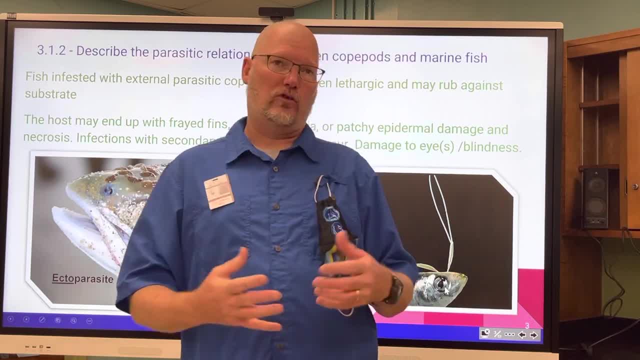 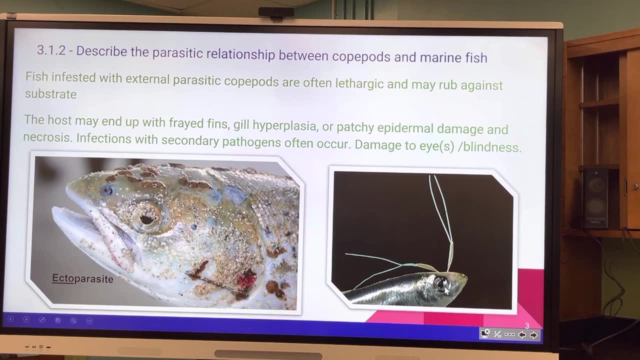 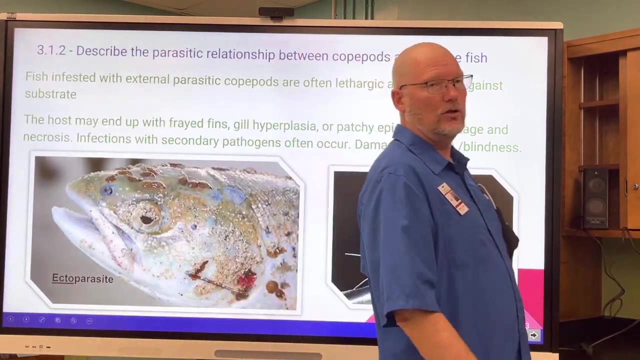 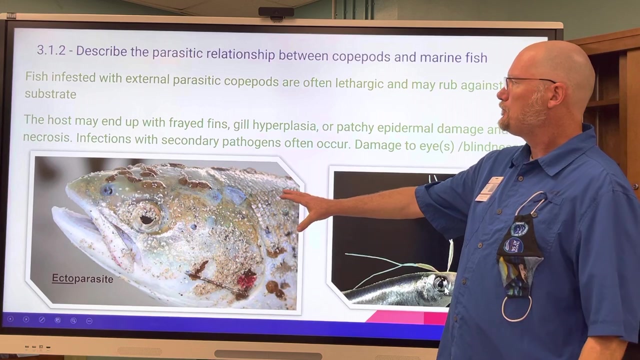 So I'm going to talk specifically about a few of these symbiotic relationships now, The first one being the parasitic relationship between copepods, which are a type of marine invertebrate, and marine fish, Which are vertebrates. obviously, they have bones, right? Okay, An invertebrate doesn't have bones. Now some of them can be. 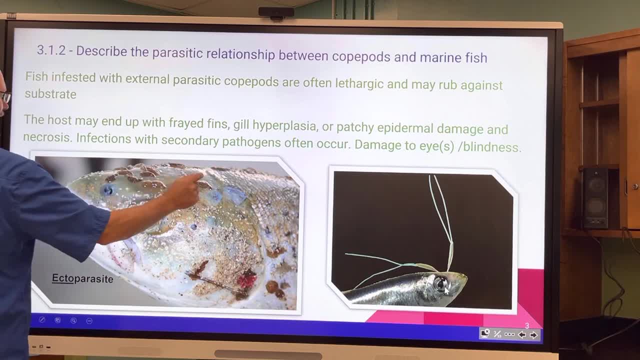 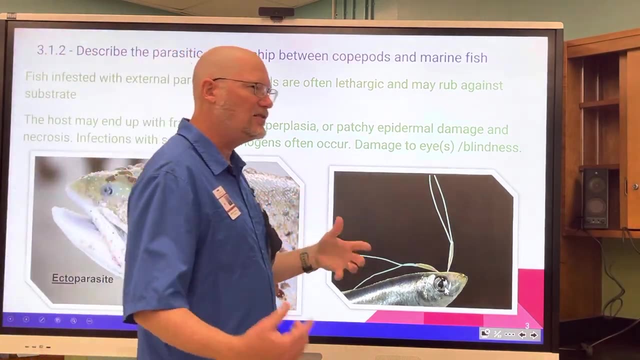 ectoparasites. These copepods are living on the outside of this fish and others can be endo. We'll talk about the endo ones on the next slide. So these, so certain different species of fish can be infested. I guess you could say infected with, but that's more like a disease. 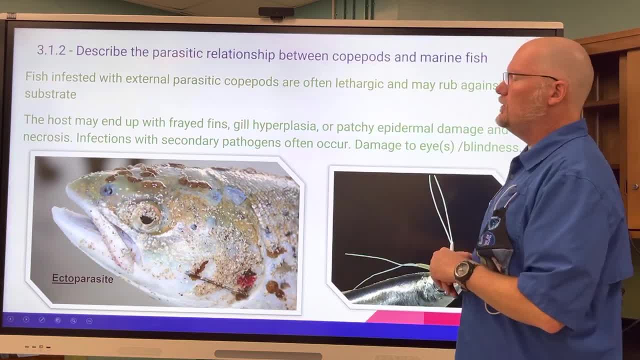 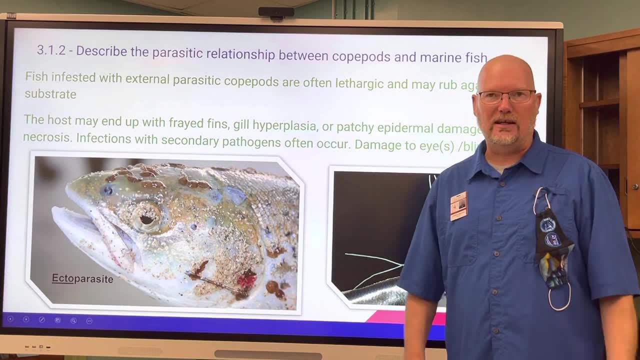 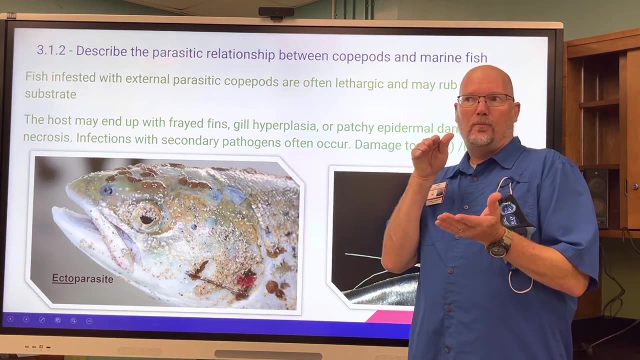 with these parasitic copepods and the fish will become lethargic. that means not a lot of energy, because these are essentially sucking their blood and eating them, weakening their bodies, and then they rub against the substrate. substrate is the bottom of whatever water they're living in. 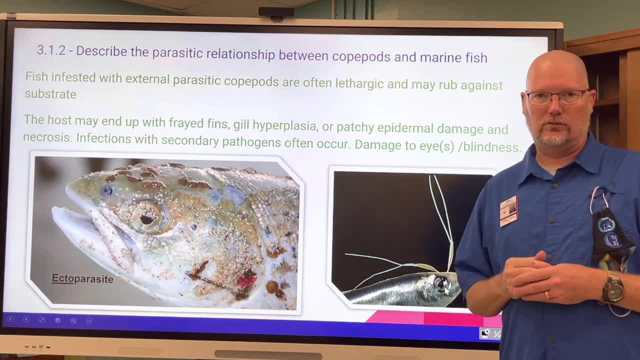 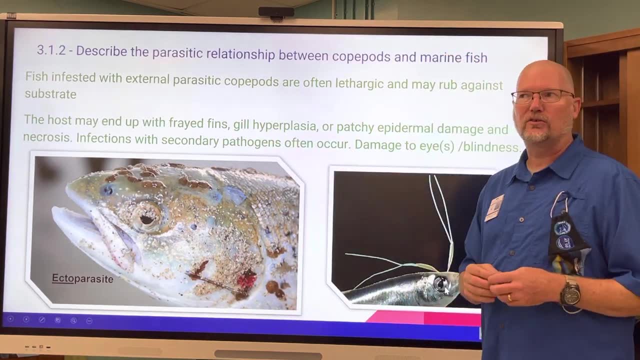 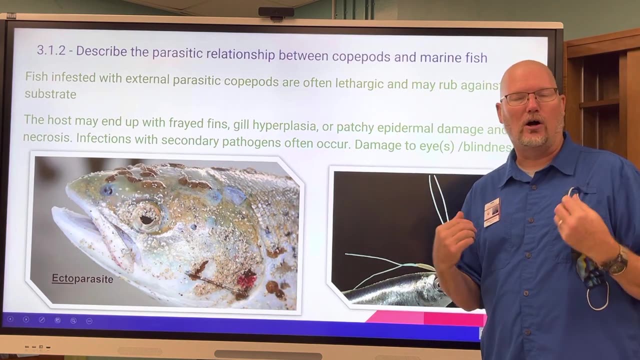 to try to rub off these parasitic clinging on copepods and some of the damage that can occur are frayed fins because of the the detriment or the negative effects of these creatures on their bodies, on their tissue. gill hyperplasia, that's essentially swelling of the tissue. 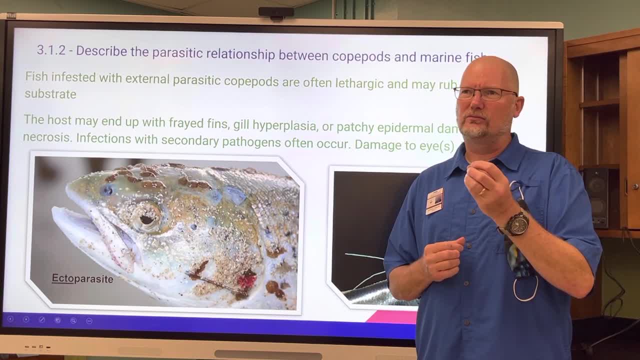 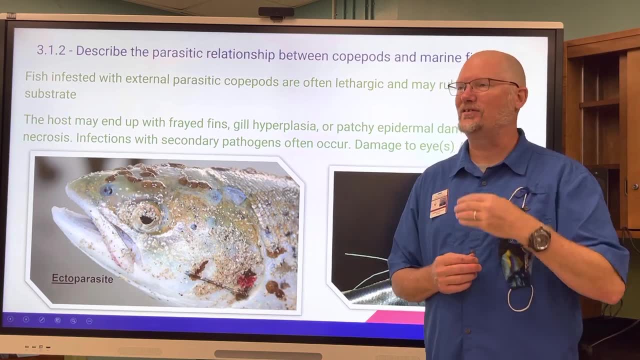 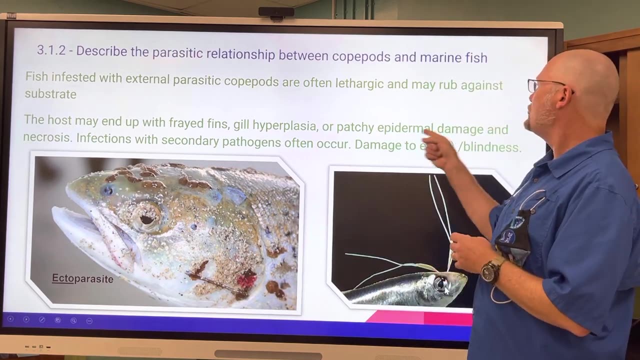 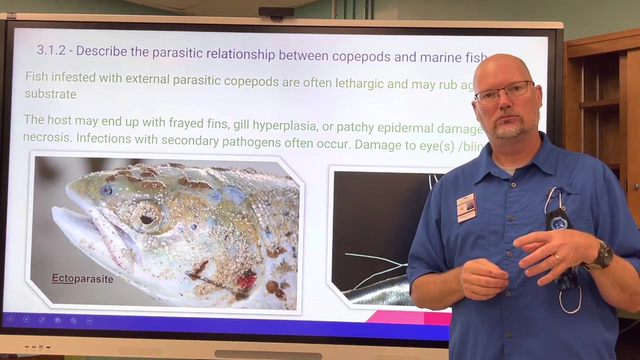 not quite to the point of a tumor, but still from constantly being damaged from the gills. gills are very sensitive. i don't know if you've ever gone fishing before. that's one of the first things that bleeds if you damage a fish or patchy epidermal damage to and necrosis. so necrosis is dead tissue necrotic. 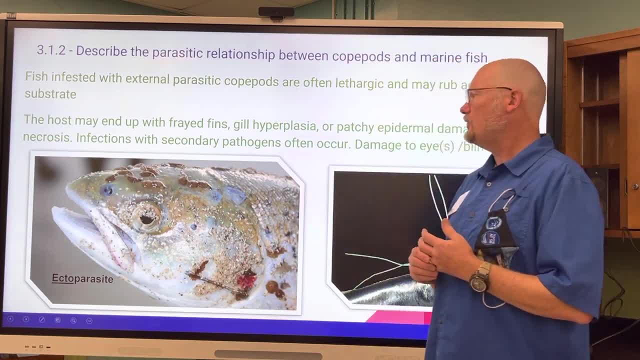 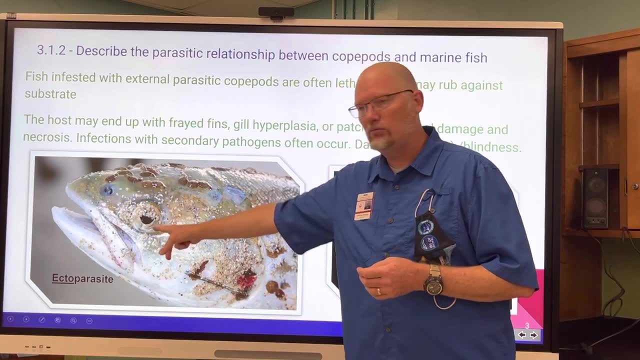 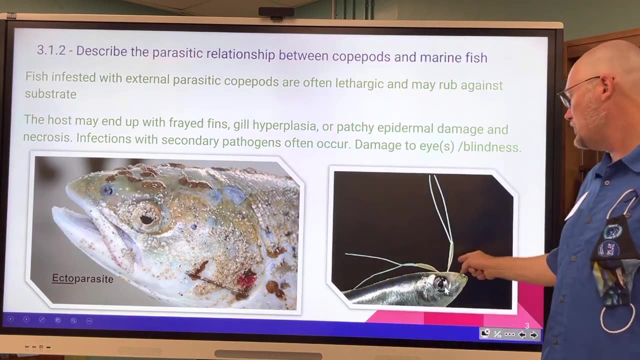 and then secondary infections. infections can occur as well, also damage to the eyes or blindness, if one of these things gets on their eye. this is just sand on the outside here, but these are the ectoparasites. so we're these different species. you can see they're very different. 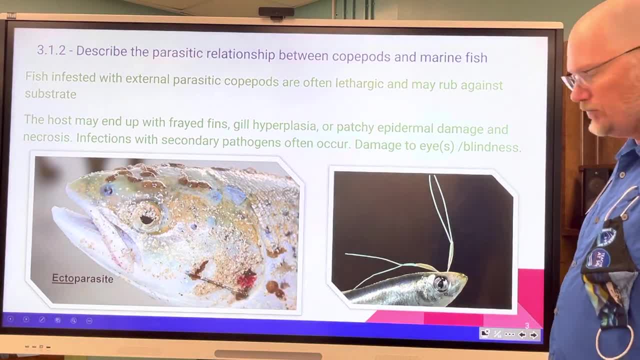 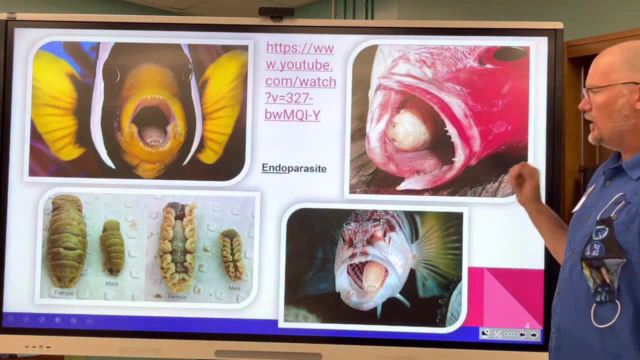 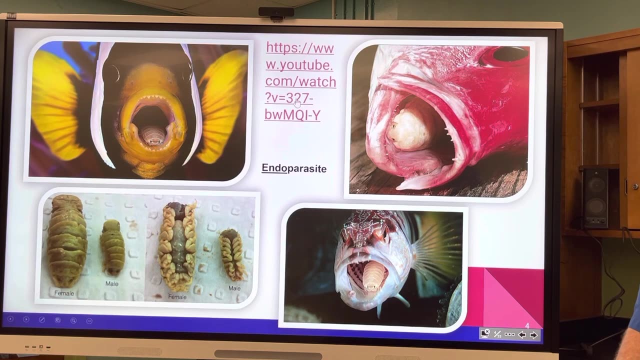 species clinging to these fish. all right, and then here's an endo parasite, so i'm going to watch a little video about this. um, i'm not going to tell you about this yet, so we'll watch the video first. the video tells talks a lot more about these very creepy creatures. okay, 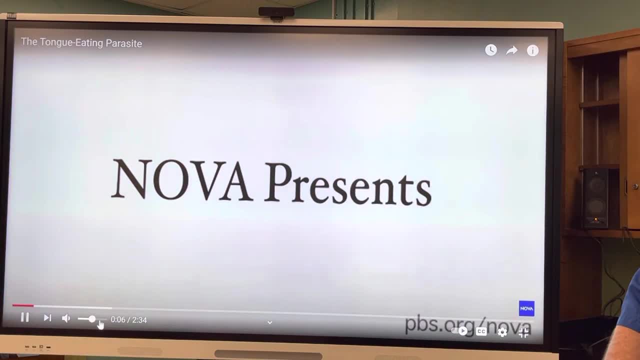 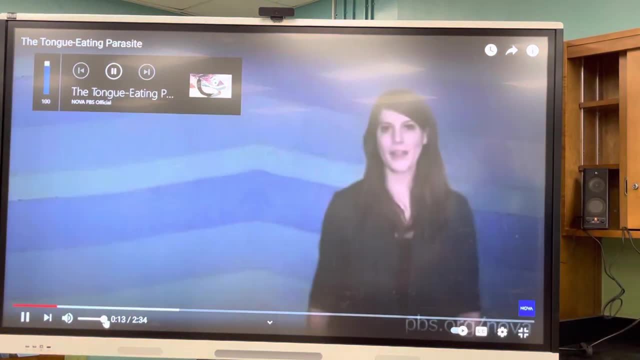 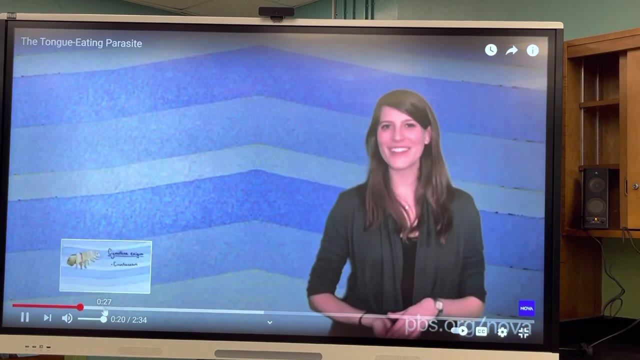 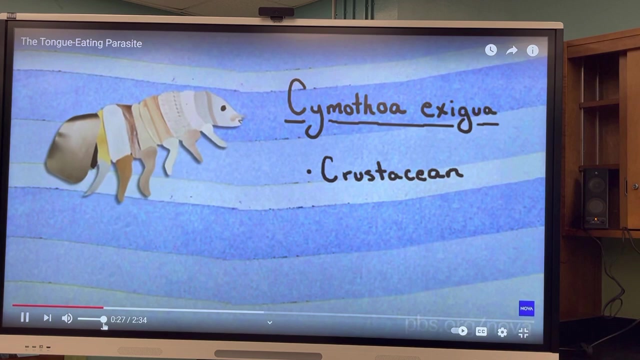 i'm about to introduce you to one of the grossest creatures on earth. it's the tongue-eating isopod simithoa exigua. isopods are crustaceans like lobsters and crabs. this particular isopod happens to live in the ocean and is a parasite. it's a sort of marine lab. 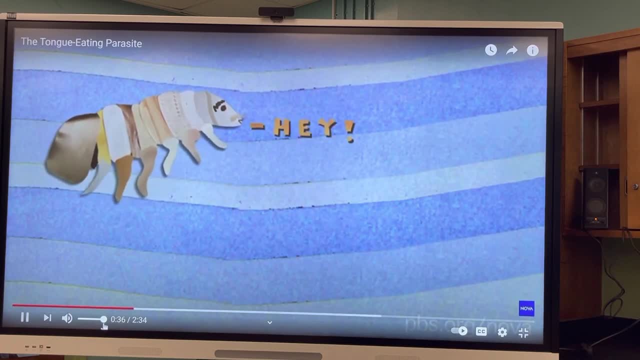 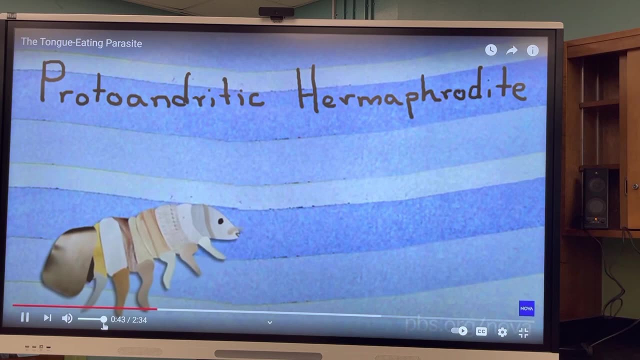 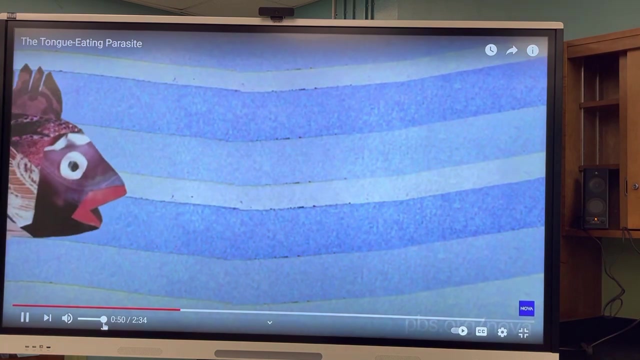 uh, only it's way creepier, hey. anyway, the first crazy thing to know about these guys is that they're what's called protoandritic hermaphrodites. that means that when they're adults, the males can become females. these isopods infest fish, so what happens is that a number of juveniles enter. 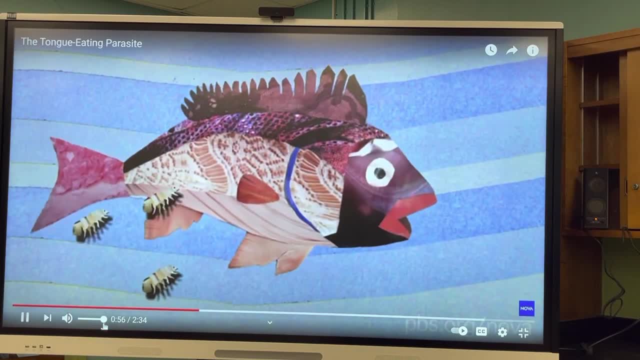 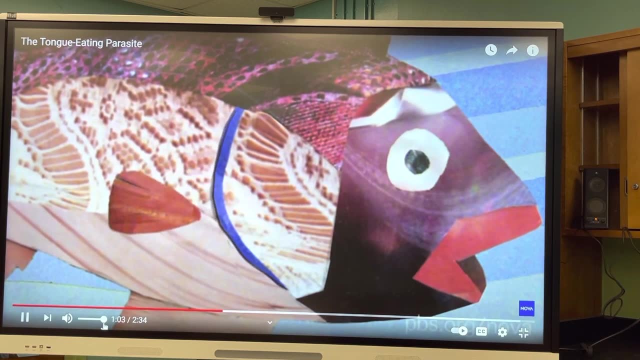 through the fish's gills and all mature into males. then one of the isopods will become a female, and that's when things get really freaky. the female will crawl into the fish's mouth and attach herself to the base of the fish's tongue. 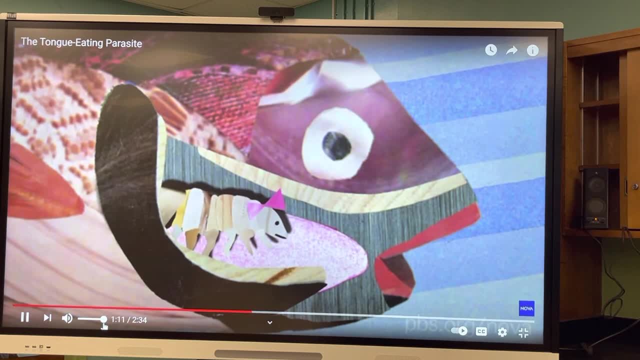 using her back legs. then she'll suck blood from the tongue until it withers and dies. this procedure is quite unpleasant for the fish, but it doesn't kill it. in fact, it starts using the parasite like a prosthetic tongue. meanwhile, the isopod just continues to hang out in the fish's mouth. 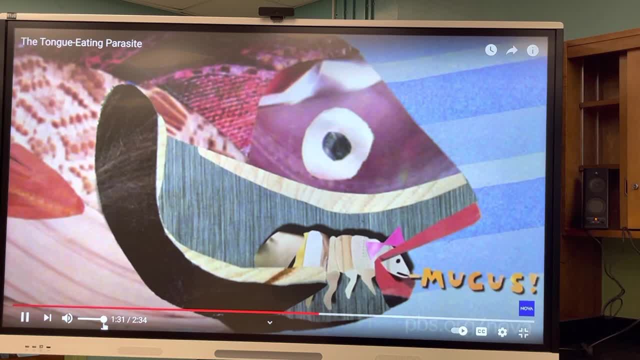 sucking its blood or feeding on fish mucus mucus. We don't know a ton about the parasite's life cycle, but based on other mouth-infesting isopods- and yes there are others- the female may even mate while in the fish's mouth. 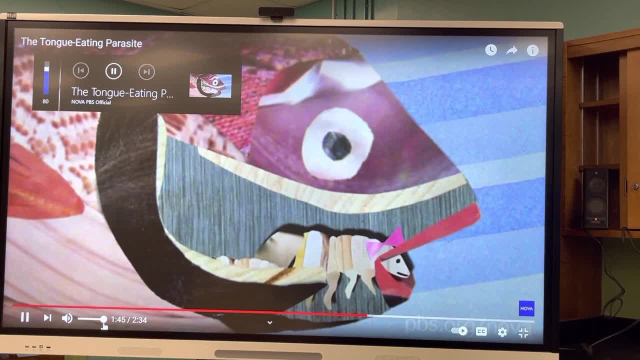 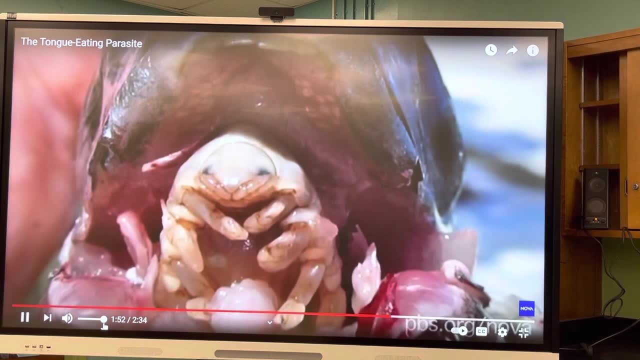 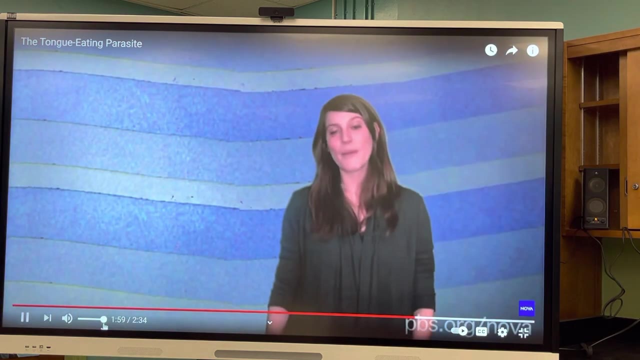 with male isopods living in the fish's gill chamber. I know this doesn't sound real, so here's a photograph of a mouth-infesting isopod to prove it. Thankfully, these guys don't infest humans, but they do infest fish that we eat. 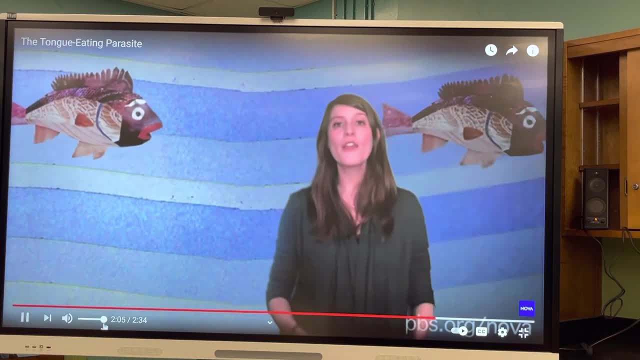 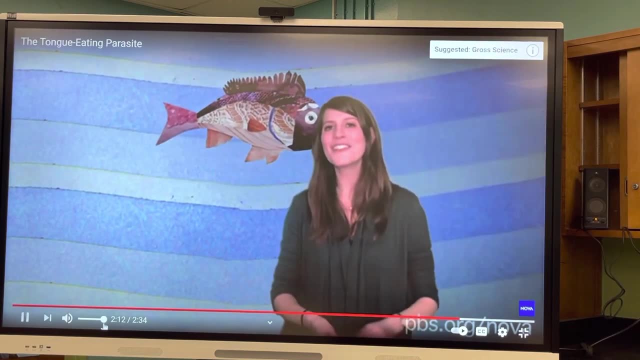 Cymothoa exigua has a preference for snapper, and other mouth-infesting isopods prey upon mahi-mahi or barramundi. So the next time you're at the grocery store, take a look inside that red snapper's mouth. 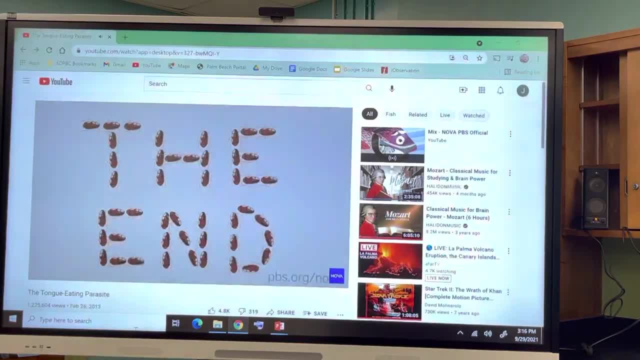 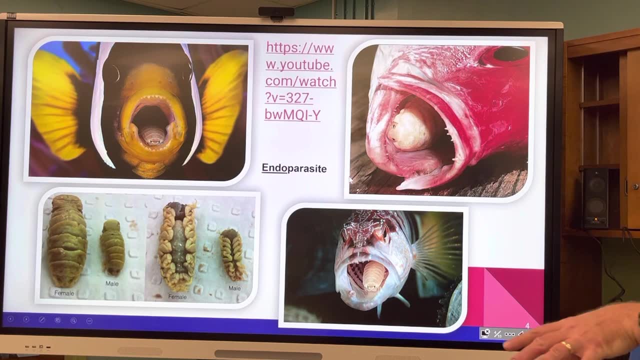 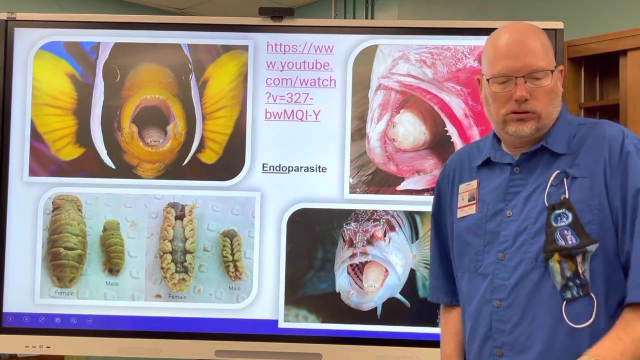 You might find a tasty treat inside Ew. Okay. so, like I said before, these are endo, meaning inside parasites, and these are real pictures of different creatures that have had succumbed to this parasitic infection. Okay, So we have this now. that's parasitic. 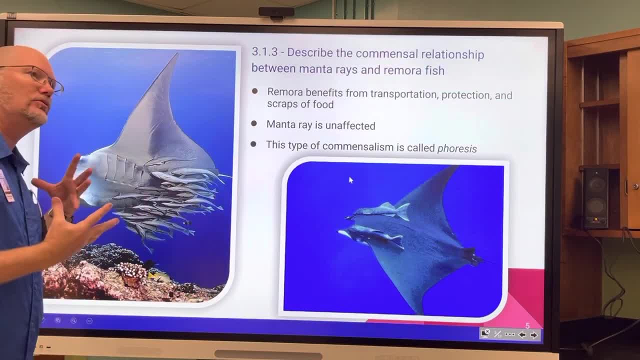 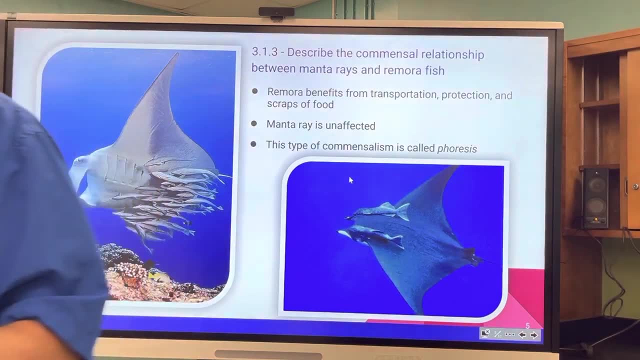 This is commensalism. So remember what commensalism is. Commensalism is when two species interact and help each other, like what you guys are supposed to do with your partners at your tables. You're supposed to help each other. 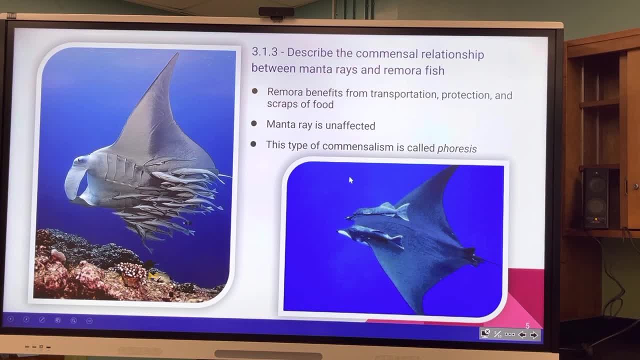 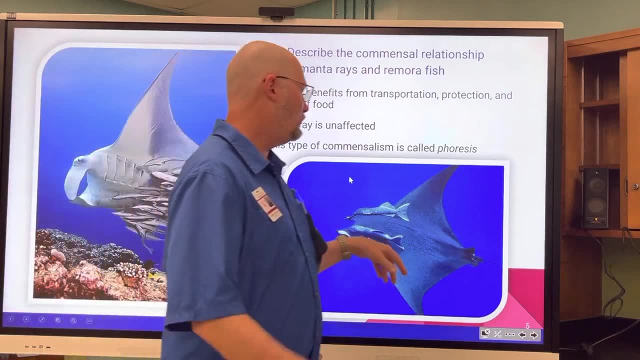 not be so selfish with everything, But you're not a different species. So, manta rays, we have them in the Atlantic Ocean, We have them here out, just right off the Gulf. They'll sometimes come really close to the shore. 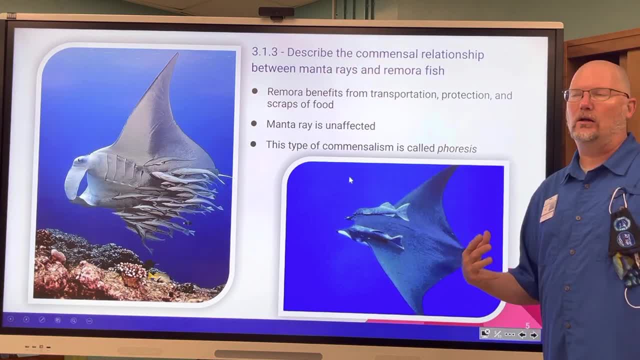 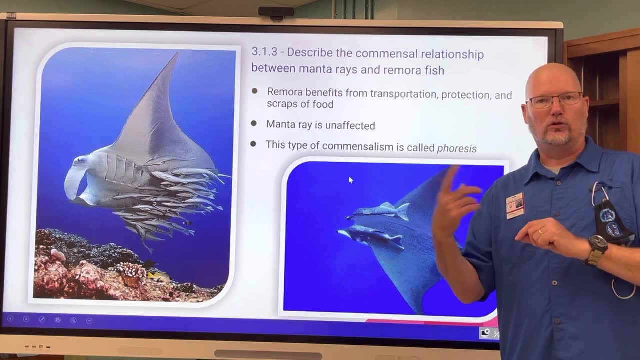 And they are typically found as well- sharks as well- with these fish attached to them. Now, manta rays are cartilaginous. They don't have any bones. We're gonna learn about those in the future. Where mora are bony fish. 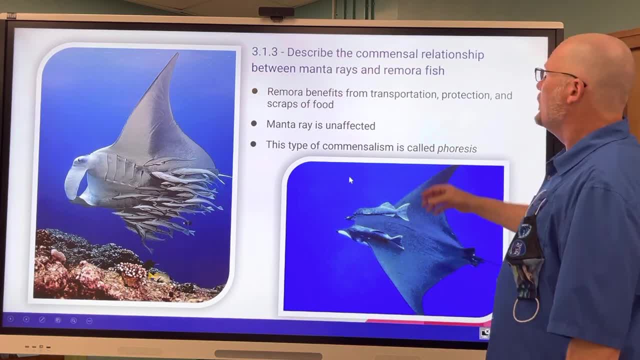 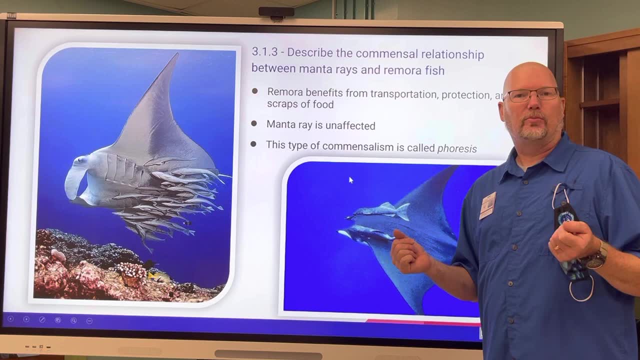 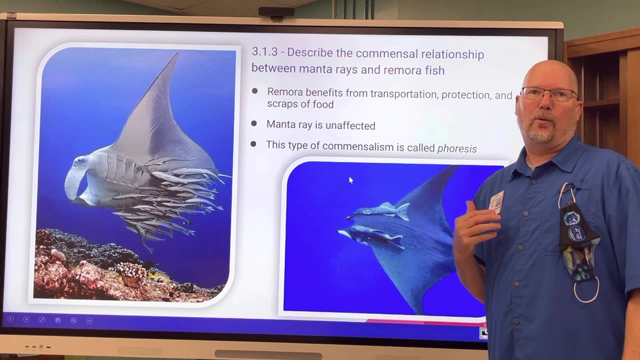 So just some extra information there. So the remora benefits because it gets a free ride on the manta. It's like sitting on the wing of an airplane Protection because they're relatively small And if you hang out with somebody big. 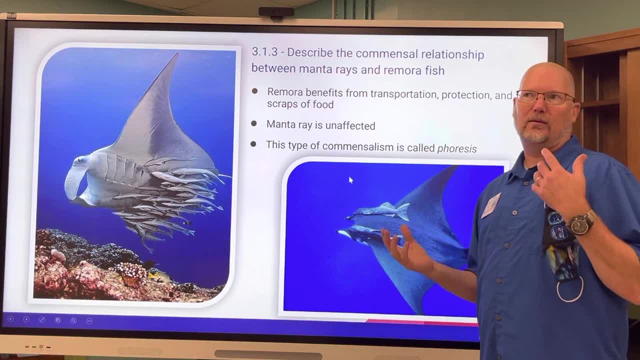 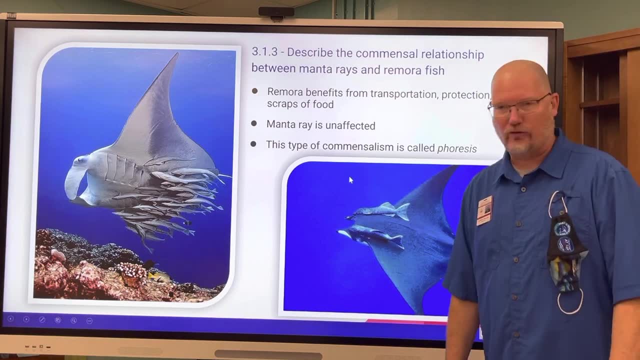 they're gonna protect you right, And scraps of food that may get left over from the manta ray finding its own food. okay, Manta rays are really kind of filter feeders, But if the remora are hanging out around sharks, definitely there's gonna be lots of scraps of food. 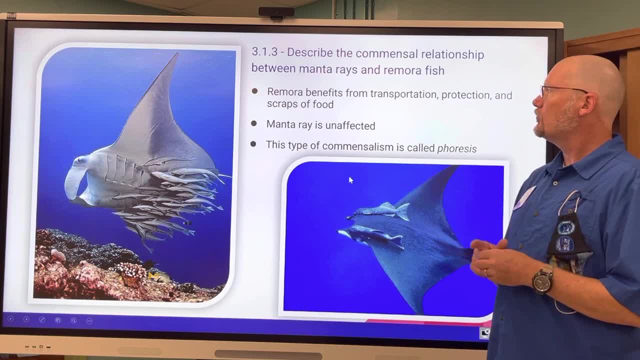 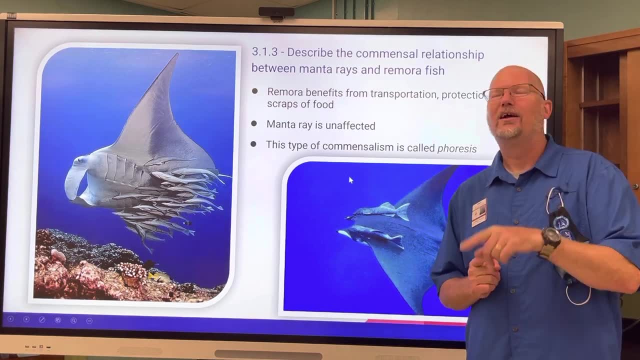 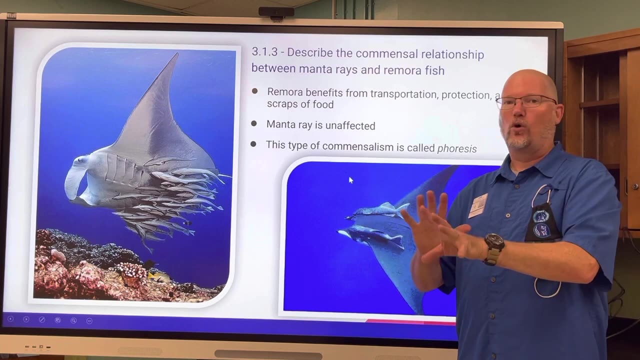 I'll show you a picture of that next. And of course, the manta ray is unaffected, Right. I think I described mutualism before, where they both benefit. This one is: one is benefited, the other is not benefited or harmed. 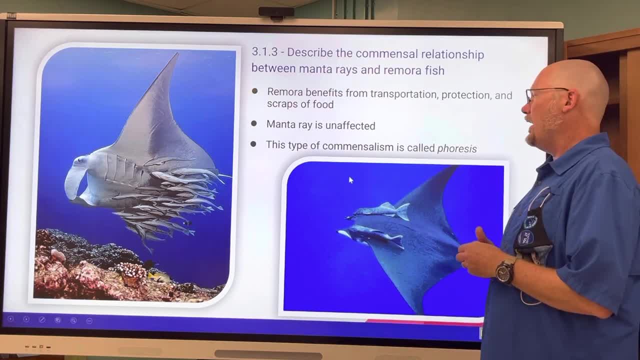 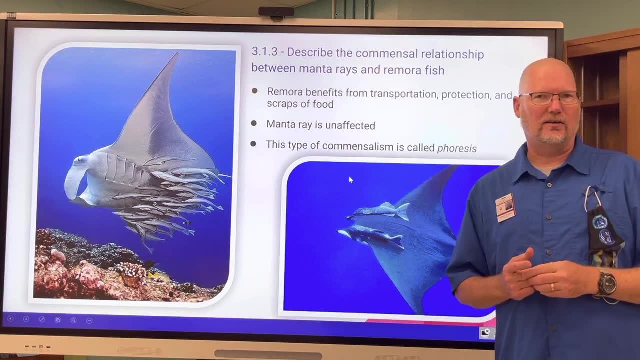 It's just unaffected, right, That's commensalism. sorry, And then, but this special type of commensalism between these two- and this is one of those words I believe that you defined in your assignment yesterday- was phoresis. 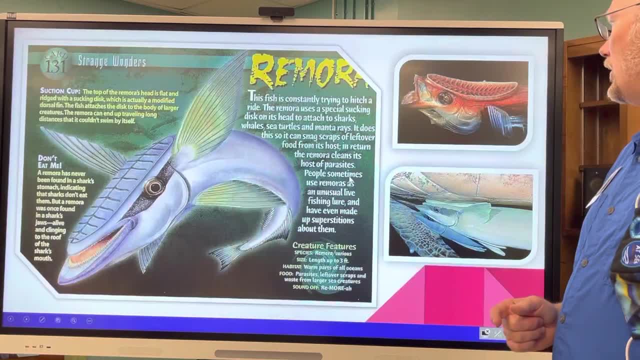 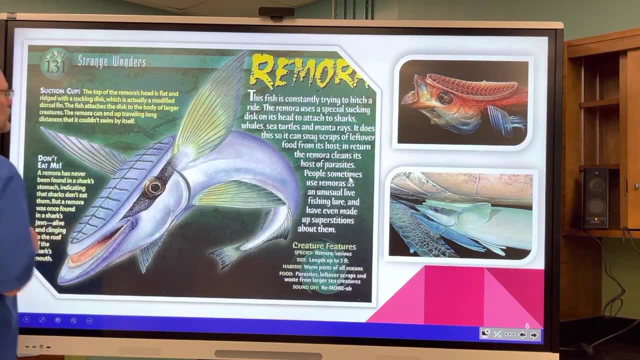 That's how you pronounce it, phoresis. So here's the closeup of the remora's suction cup. okay, And there's a question about this in your notes? Your notes are filled with all kinds of questions and extra things you have to put in. 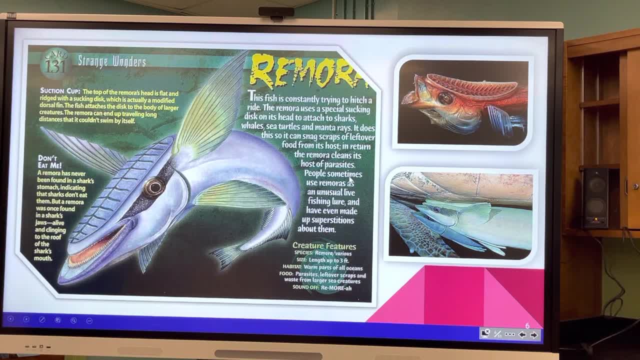 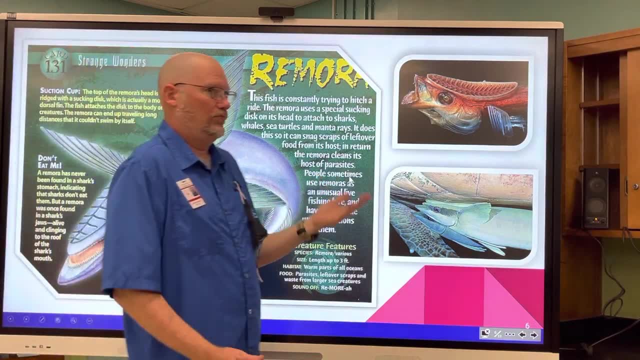 so just be aware of that while you're going down. It's a modified dorsal fin. So how many fish have you know? So how many fish have you know? So how many fish have you know? So how many fish have an actual fin you know? 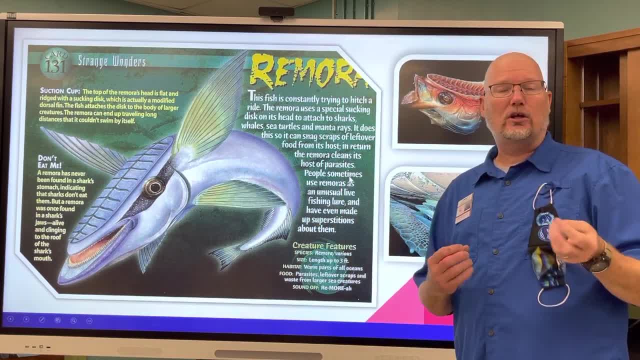 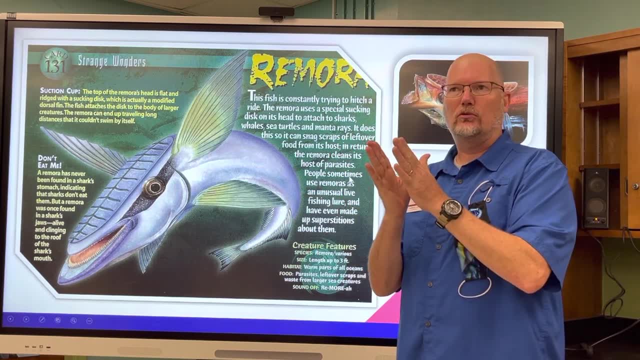 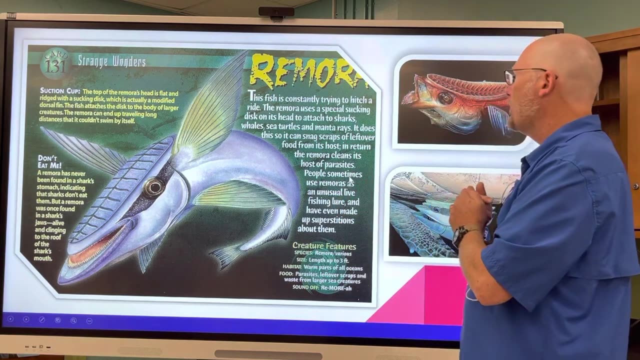 back here on their back. Evolution has developed that fin into kind of like a sucker, which it can grasp on and hold on while the larger organism is swimming. so they can hold on, okay, And they always try to hitch rides. And this is what they look like. 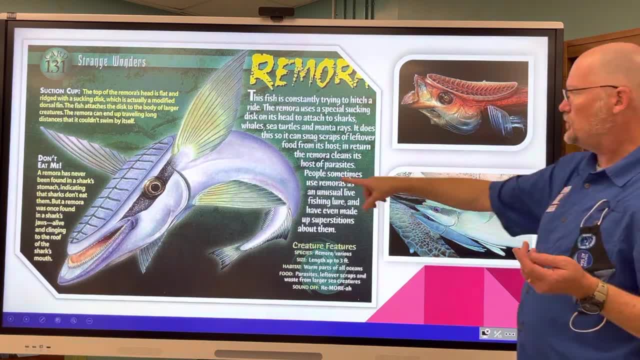 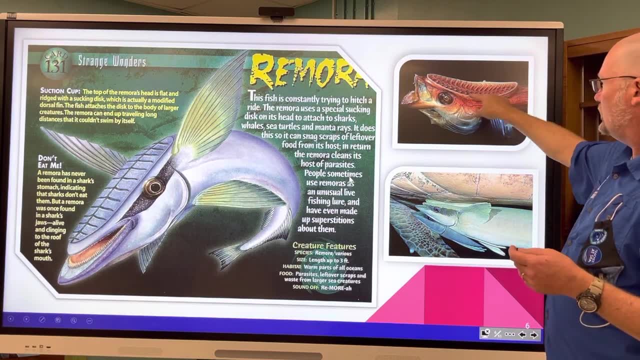 There's different species. This is the same species as that. This is the same species as that. This is the same species as that. This one's a little bit different, as you can see, And it's definitely a suction cup okay. 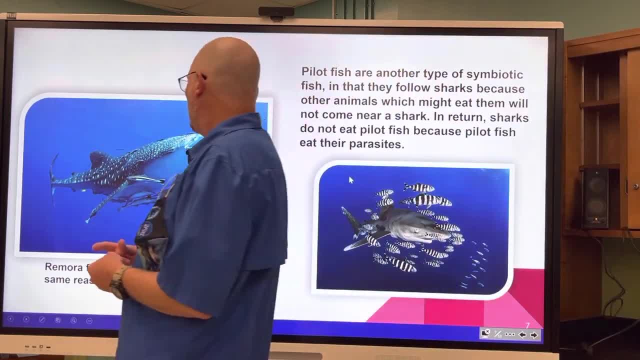 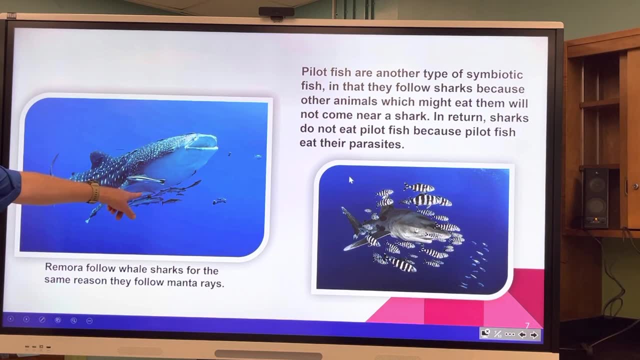 And then pilot fish is another example. So here you have a whale shark with remora. So here you have a whale shark with remora definitely swimming around. These are the striped remora, but there's also a pilot fish here. So, and for the same reason that they have the commensalistic 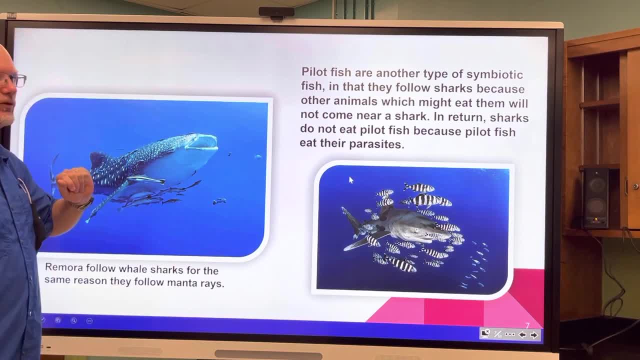 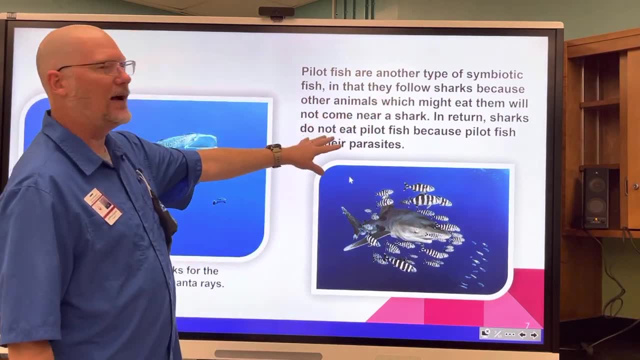 So, and for the same reason that they have the commensalistic relationship with manta as they do with the whale shark. And then these are pilot fish and they follow sharks because other animals might eat them, but they won't come near the shark, right. 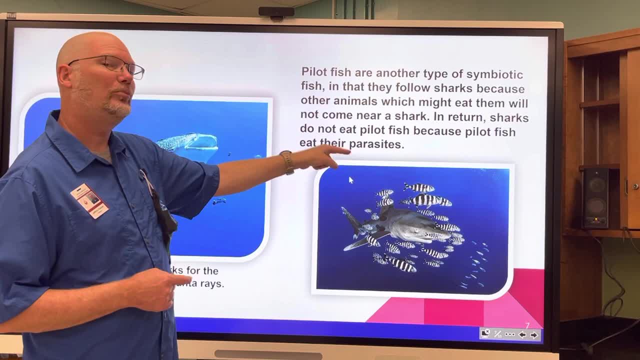 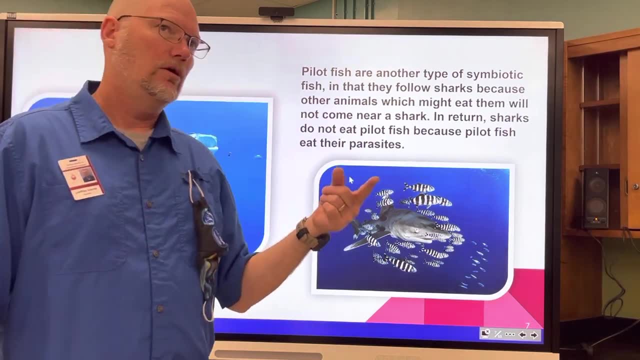 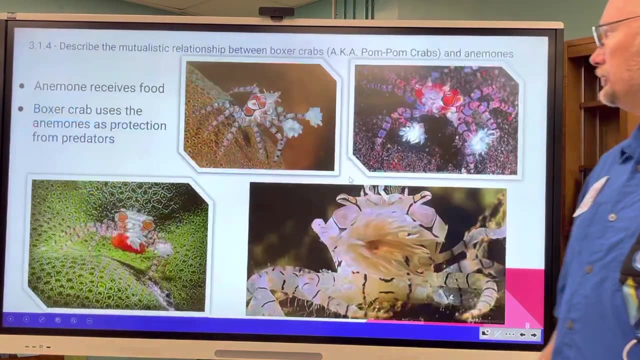 Like Zoe said before, And in return, the sharks don't eat the pilot fish, because the pilot fish eat parasites off of the shark, like we've mentioned with the cleaner shrimp before. okay, So these types of relationships are happening all the time out there. 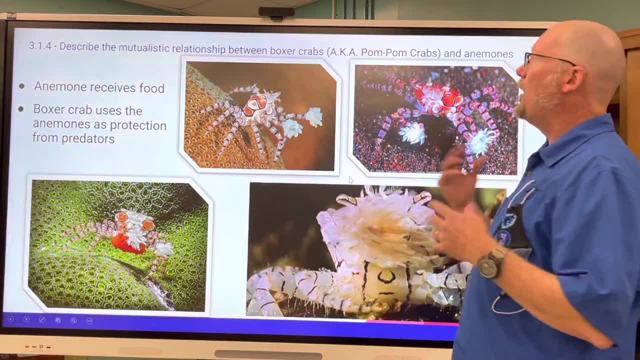 So these types of relationships are happening all the time out there. So these types of relationships are happening all the time out there. So the last one we're going to talk about is the pom-pom crab or the boxer crab. okay, And anemones. 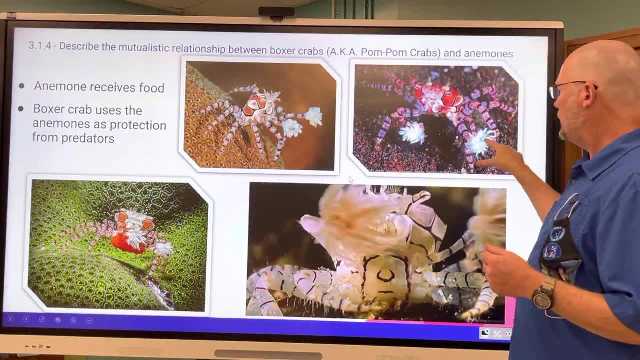 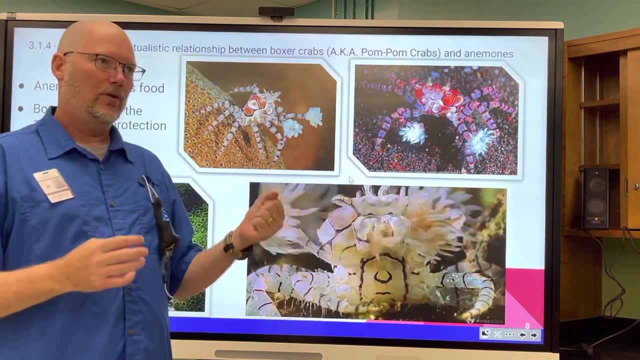 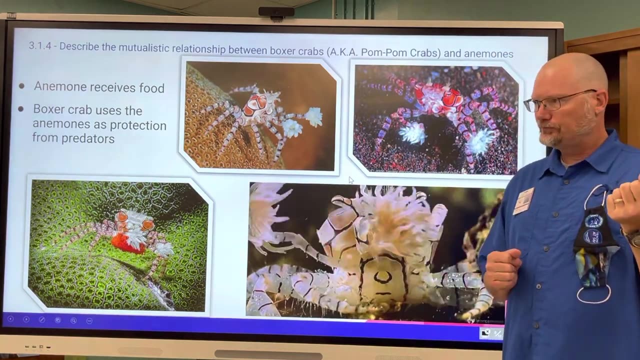 So this is not part of the crab, These things that the crab is waving back and forth. These are actually anemones, which are invertebrates that have stinging cells. They're related more to, I guess, corals and jellyfish and those types of organisms. 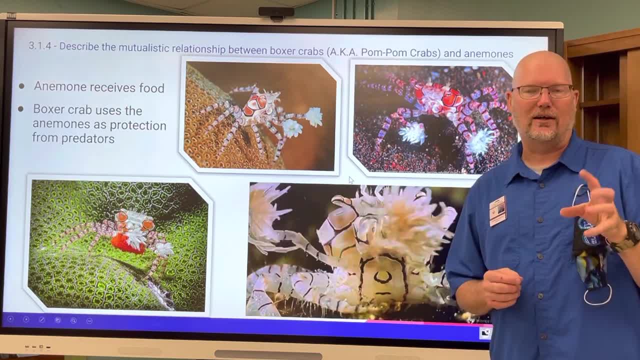 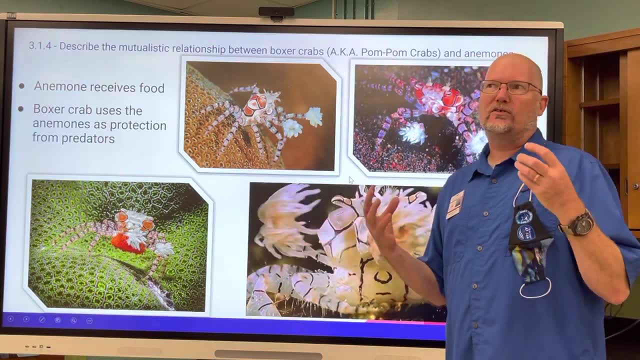 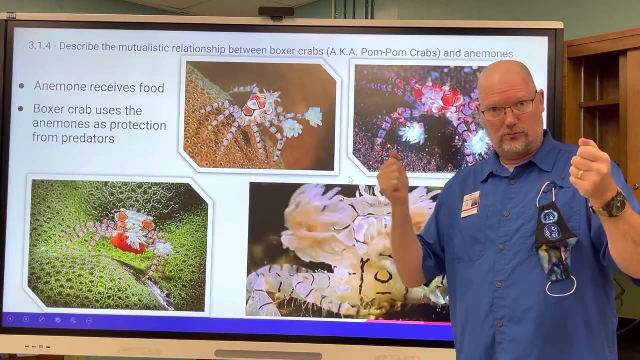 with organisms with stinging cells. They're called cnidarians, but we'll get to that later. They're animals, They're not plants. And through its development, through its growth and development to maturity, these boxer crabs will pick up two boxing gloves. C anemones. 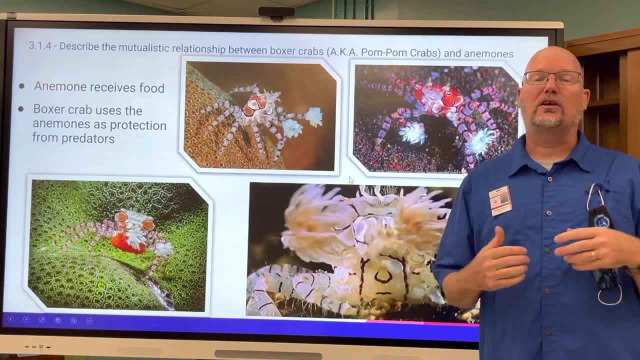 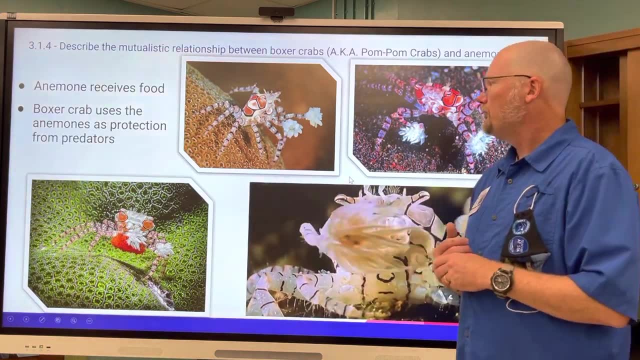 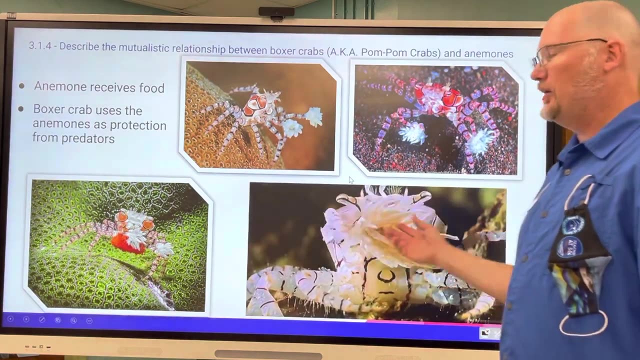 And they will use them as protection against something that's going to come and attack it, which is quite amazing. Okay, so now the anemone also gets protection from being eaten because of the crab right. It's keeping a fish from eating the anemone, moving around taking it. 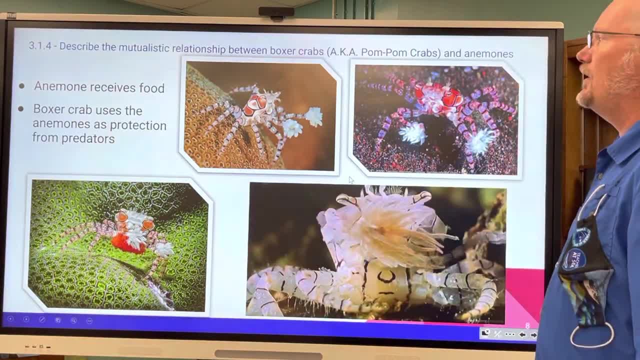 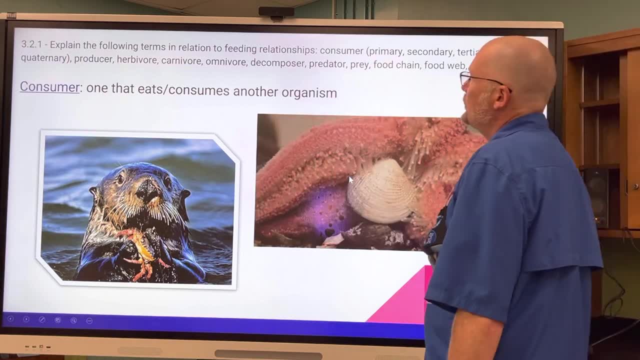 Otherwise the anemone would be stuck in one spot. So the anemone gets to travel around as well. So it receives foods, crabs, leftovers, Okay, so now we're moving on to the next topic, which is relationships. 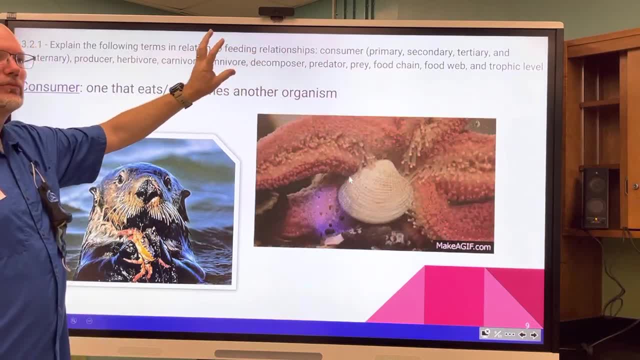 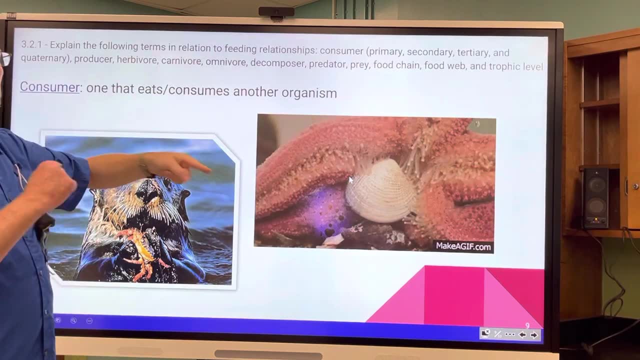 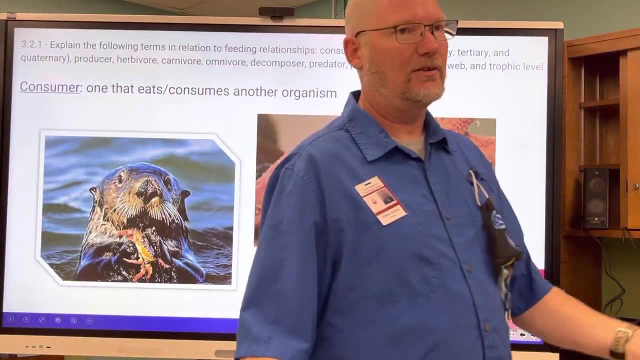 In feeding, among consumers, producers, omnivores, carnivores, herbivores, decomposers, the predator-prey relationship, food chain, food webs and trophic levels. That's a lot of words, That's a lot of vocab. 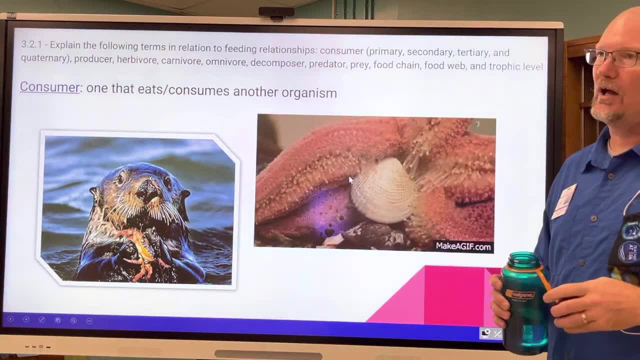 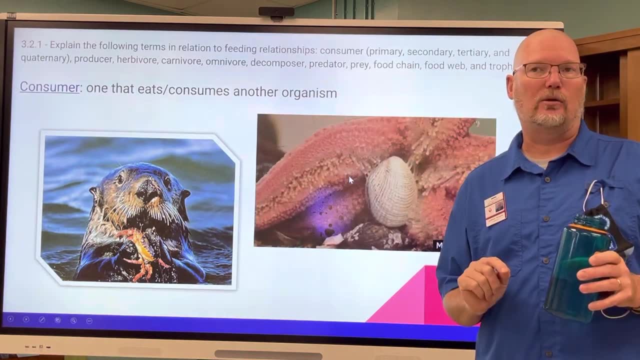 So I broke them up into each having its own slide and with examples. So in your notes you'll see that there's room for you to include the examples that I talk about the marine. There's some marine examples on each of these slides, okay, 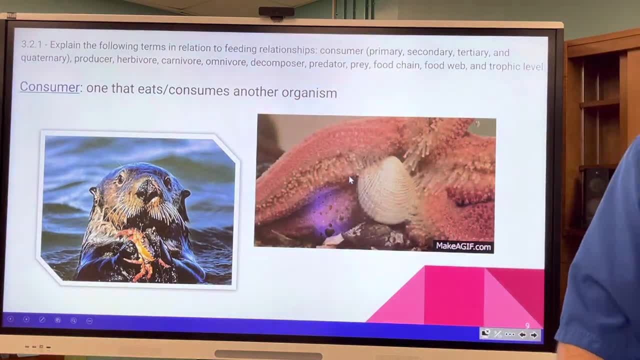 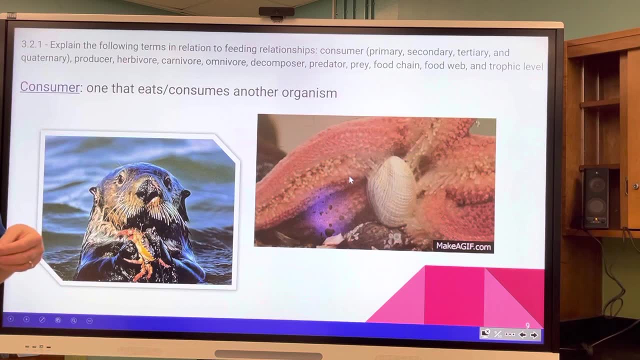 Okay, so we're going to talk about consumers first. Consumer- well, we're consumers, so we kind of know what that means. Something that consumes something, uses it for, typically for energy. okay, In this case, we're talking about consuming food, right? 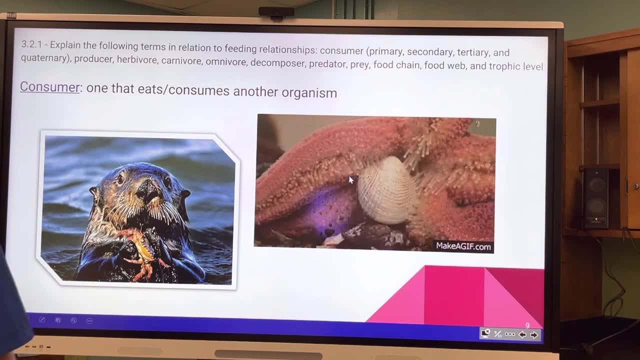 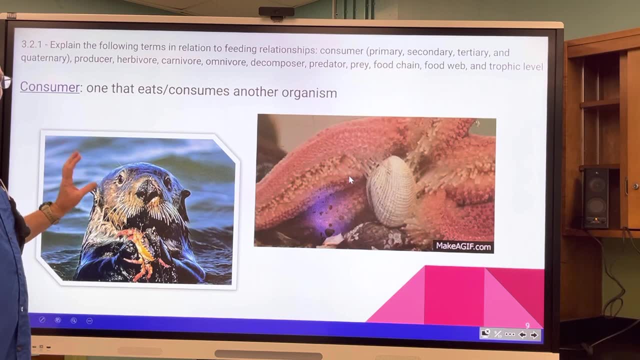 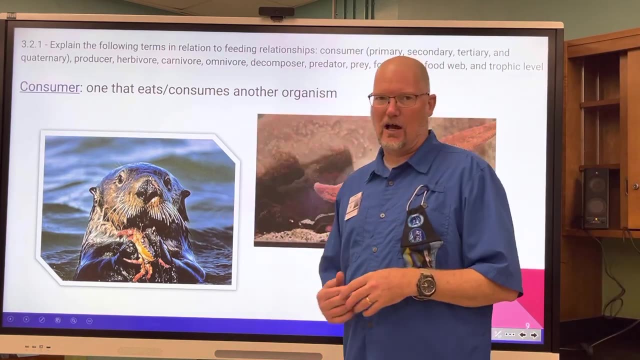 So when one organism eats another organism, so here you have, in the Pacific Northwest you have the mammal, the marine mammal with the thickest coat of fur in all the world is the sea otter, and obviously he's eating a crab. 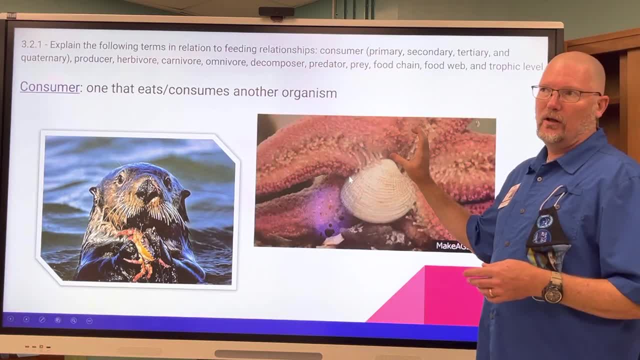 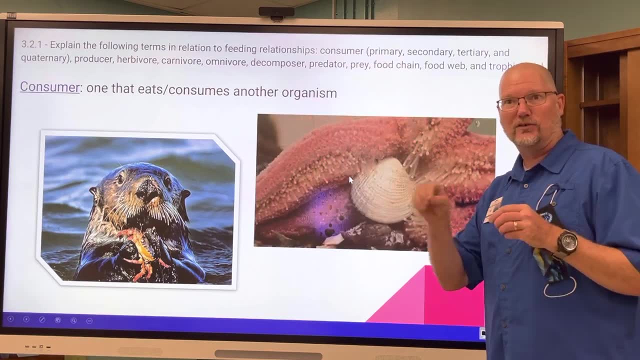 And then you have this invertebrate, this Echinodermata. This is a sea star. We don't say starfish because they're not fish, That's an old term. We say sea stars And they use their tube feet. 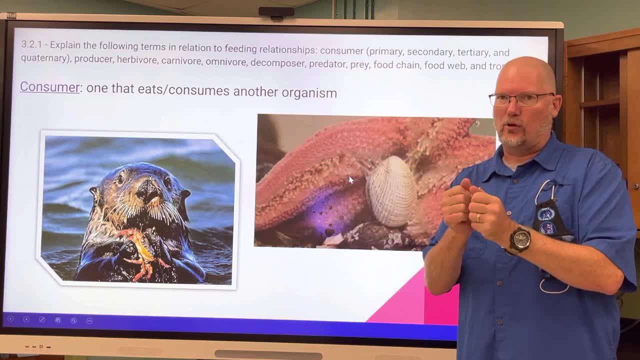 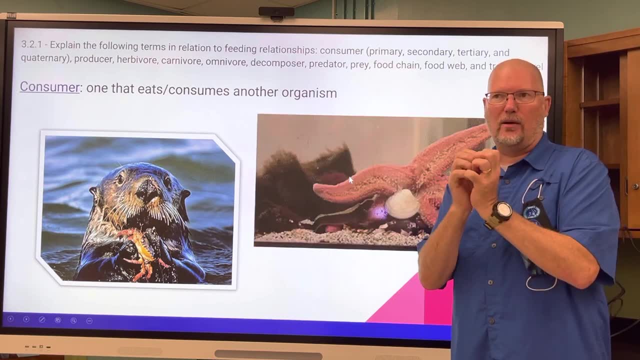 When they get enough tube feet on a clam. I don't know if you've ever tried to open up a clam or a mussel, but you can't do it with your bare hands. Nobody can. You have to have a tool. Their tool is these tube feet that grab on and just inch the clam open a little bit. 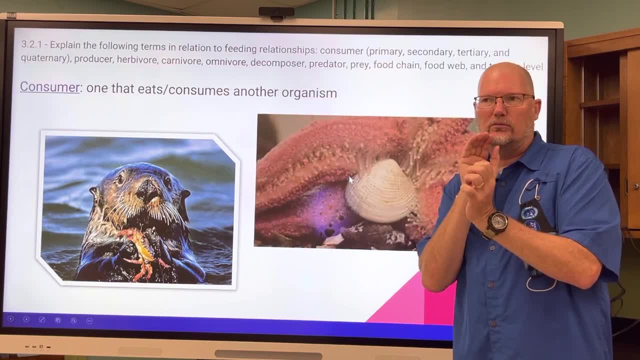 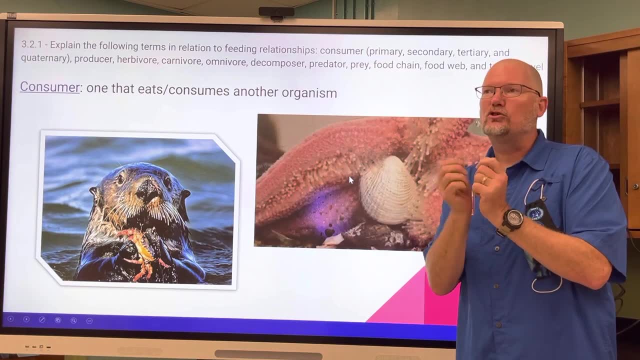 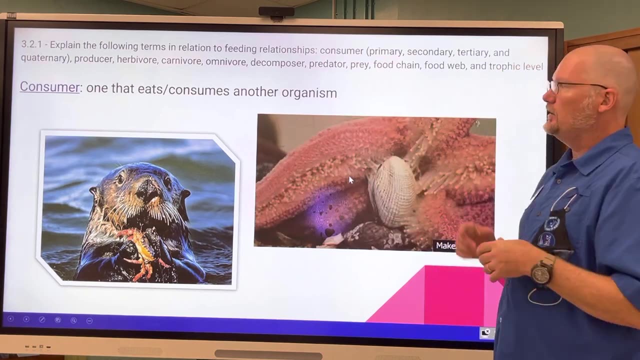 and then they eviscerate, in other words throw up their stomach into the clam through the tiny space that they open up, and then they digest the clam from inside the clam shells. That's pretty wild. So definitely a consumer. 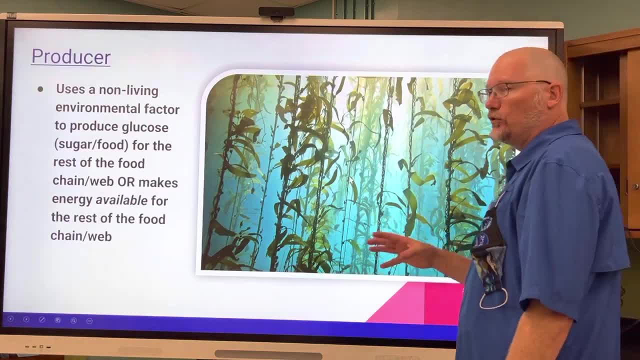 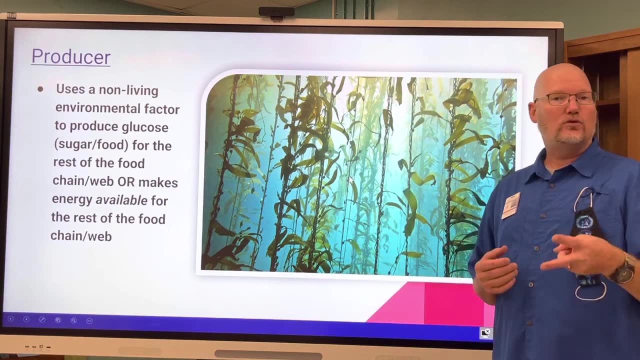 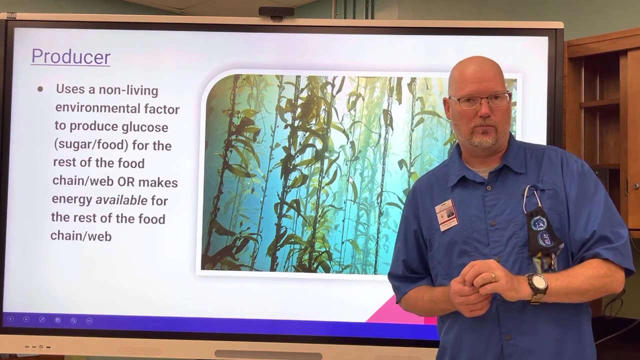 an organism that eats another organism. Producers, on the other hand, don't eat anything. They make the food, They produce the food, And there's two types. There's the photosynthetic producer and then there's the chemosynthetic producer. 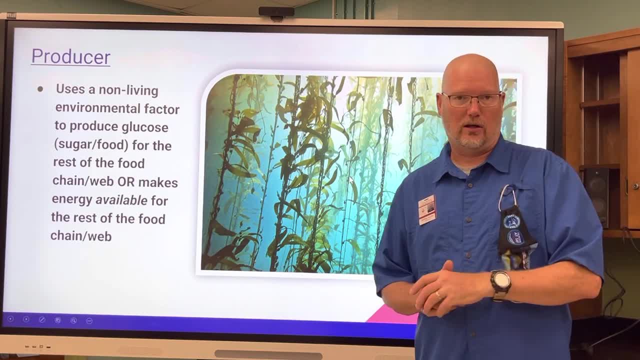 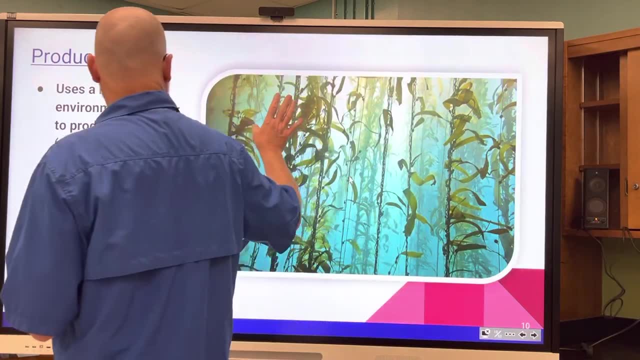 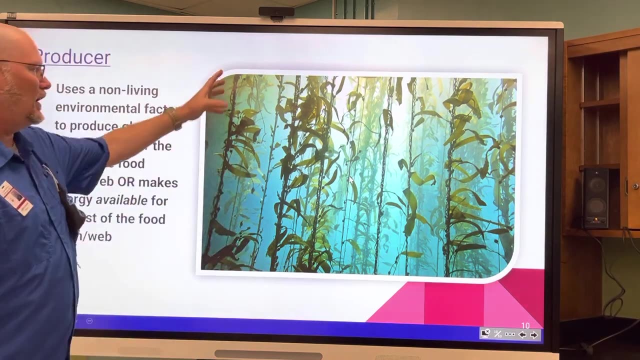 the ones that live down deep in the hydrothermal vent environment. Okay so we'll talk about the photic zone first. Okay, So they are using a non-living environmental factor, meaning the sun. In this case, this is a kelp forest. 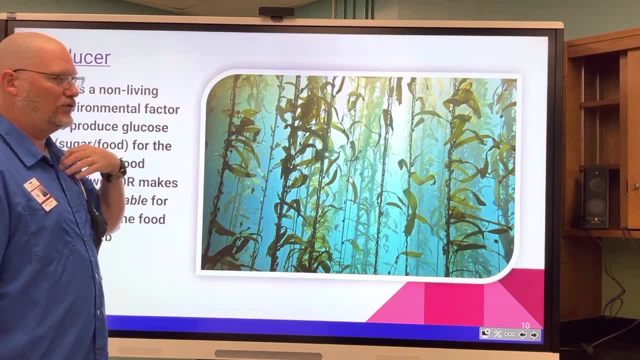 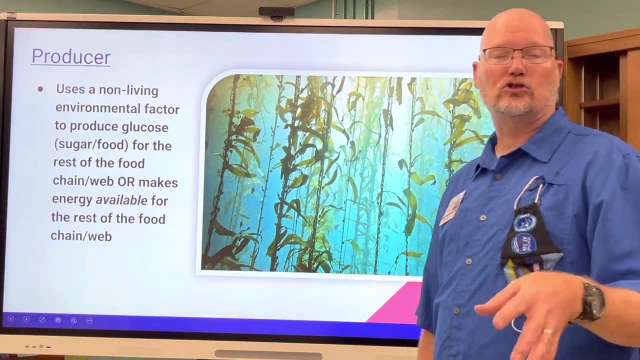 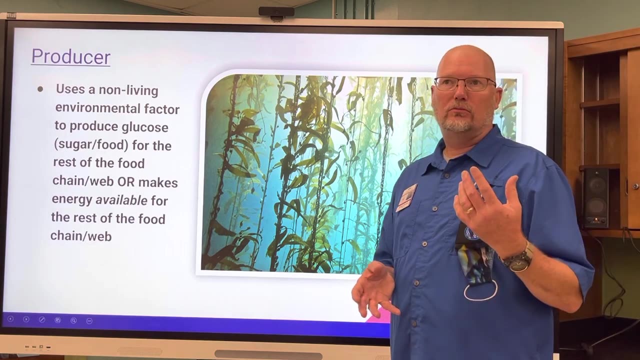 They occur in different parts of the world, but particularly as far as we're concerned in America. they grow in the Pacific Northwest- okay, off the coast of California and Washington and Oregon- And they make sugar. They make glucose, right, If you took biology. 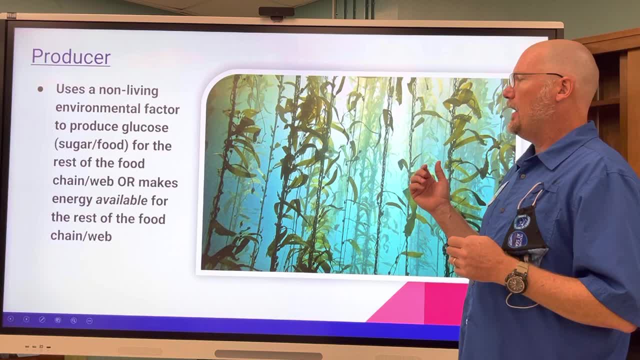 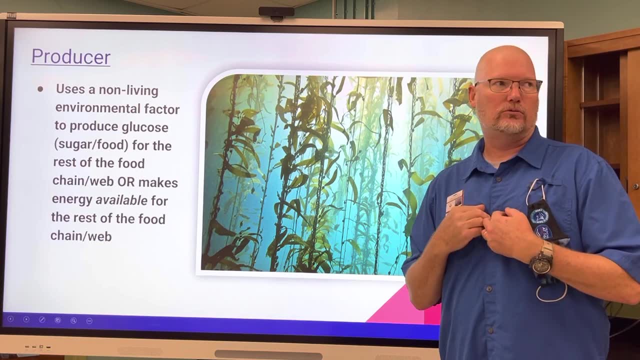 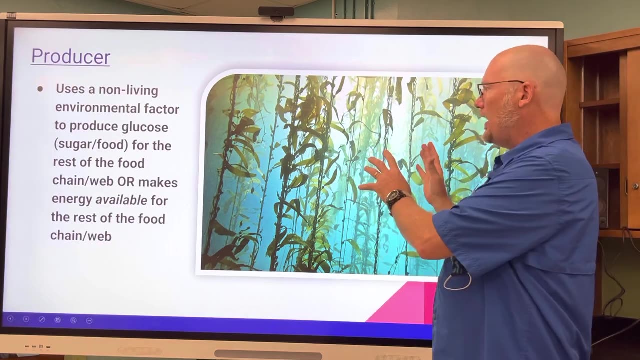 you learn this? If not, you're learning it now, And that glucose is used for the rest of the food chain, going down the line all the way to us. I guess When you eat a fish, you are getting energy that was made originally by plants or algae. 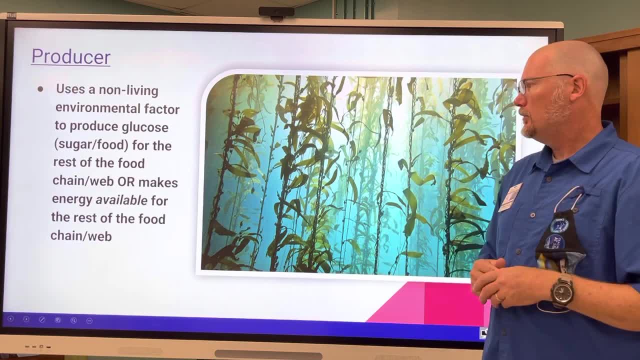 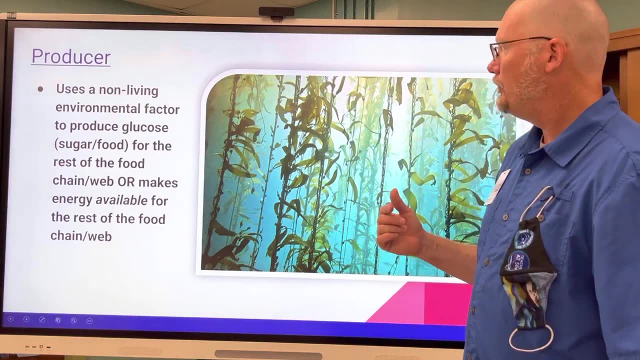 They're not quite plants. This is algae, A very big algae, very long algae, growing very fast, but it's algae And then. so that was a photosynthetic example. This is a chemosynthetic example. Remember the hydrothermal vents? 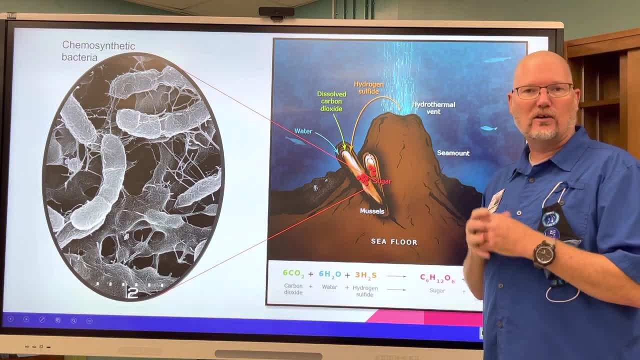 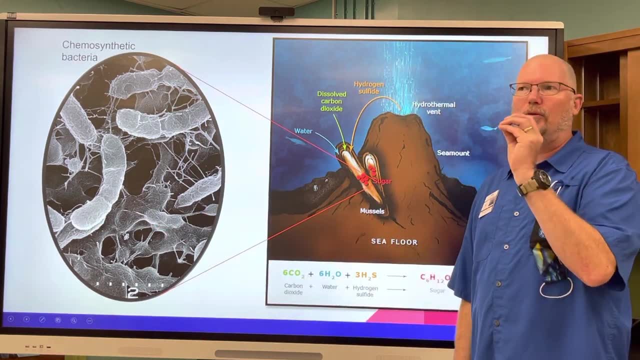 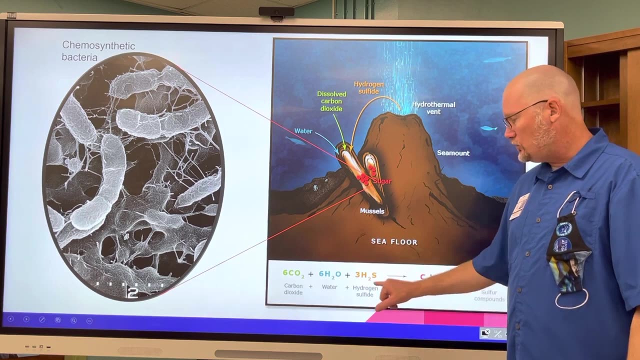 okay, These are muscles living at the hydrothermal vent and inside the muscle. are these chemosynthetic bacteria that virtually do the same thing that the plants do, or the photosynthetic producers do, except instead of using sunlight, they're using hydrogen sulfide. that's coming out of here. 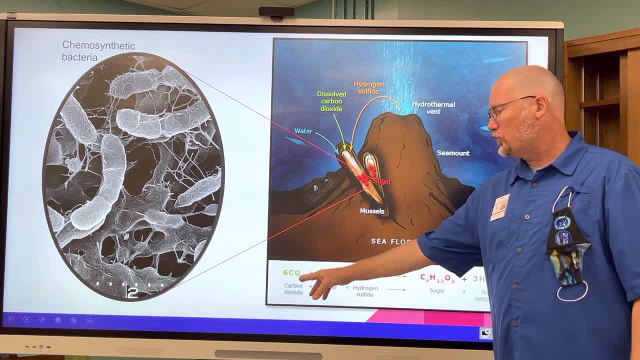 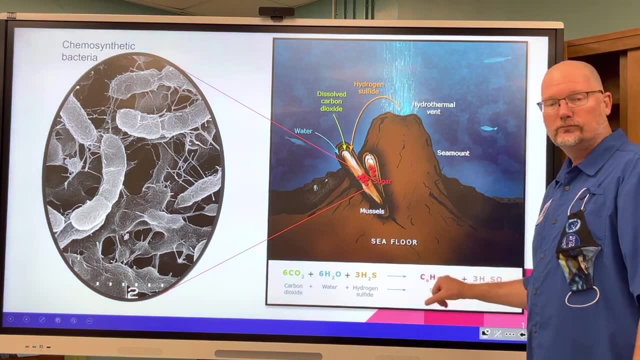 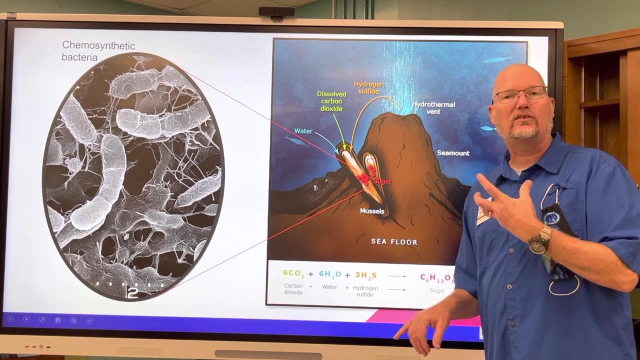 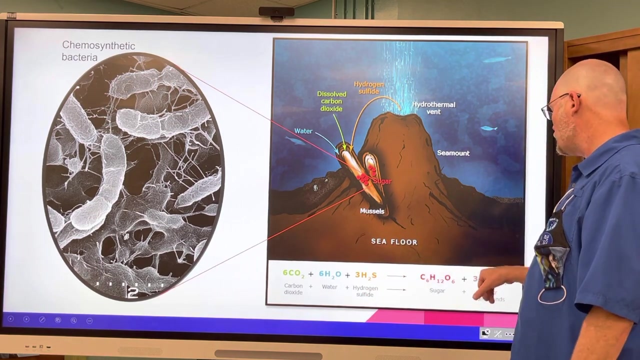 And it's their energy source. and then they combine it with carbon dioxide and water, just like a plant does, and they would, and they end up with the same product: sugar, glucose- and well, in our case, in plants case, it would be oxygen. but down here they're producing other compounds because they have to do something with that sulfur, so this is hydrogen sulfate actually. 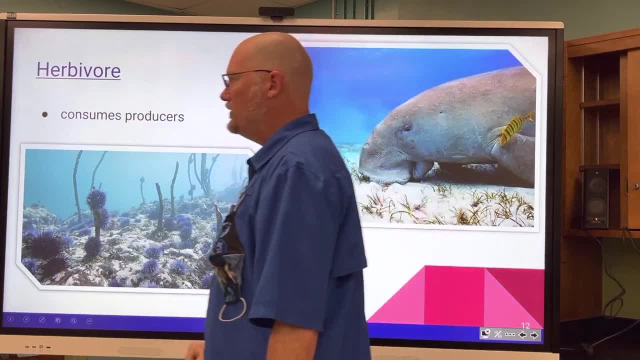 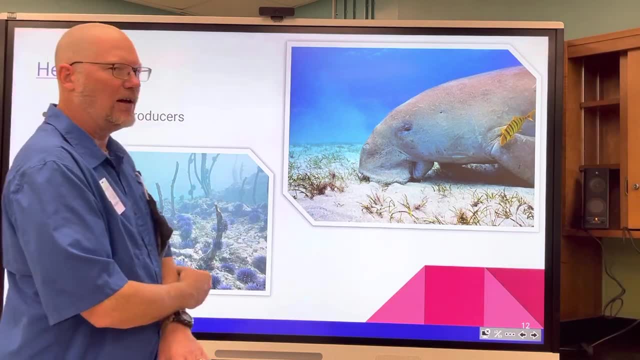 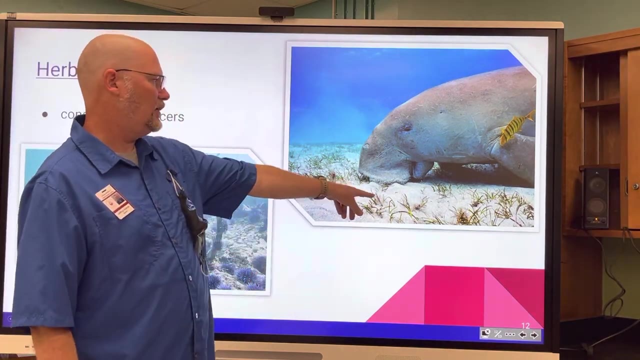 Herbivores. Here's our famous manatee that we're familiar with. If you've been, actually, that might be a dugong, which is a relative of the manatee, and they love both organisms. They're similar family, same family. They love to eat sea grasses. 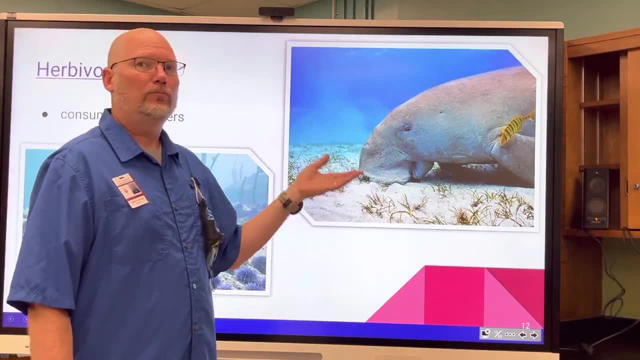 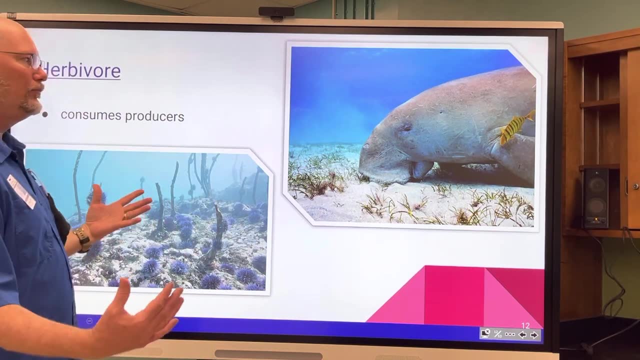 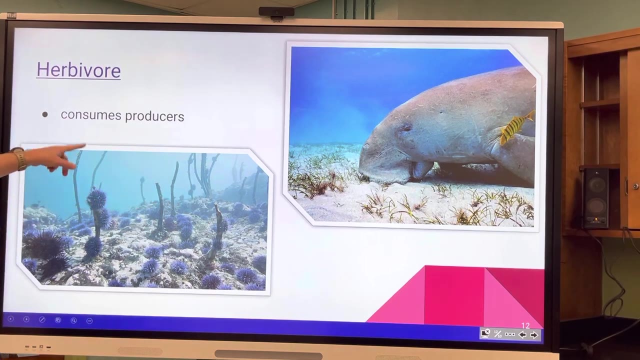 Okay, so they're like- that's why they call them sea cows, because they graze along the bottom, just like- and they're gentle and you know, but big Um, just like land cows, All right, And these are sea urchins that are eating kelp in a kelp forest and you can see that they've eaten a lot and they've grown a lot. 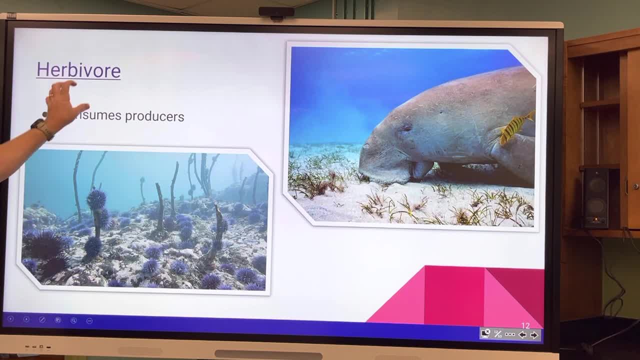 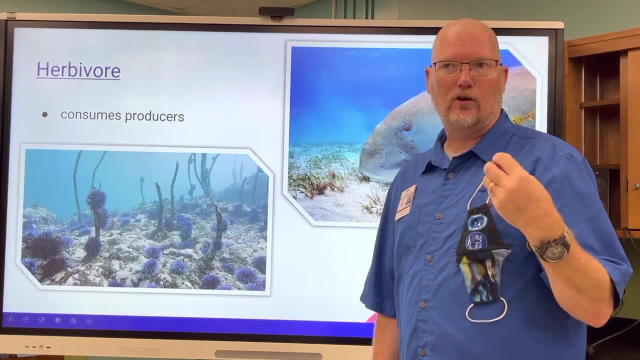 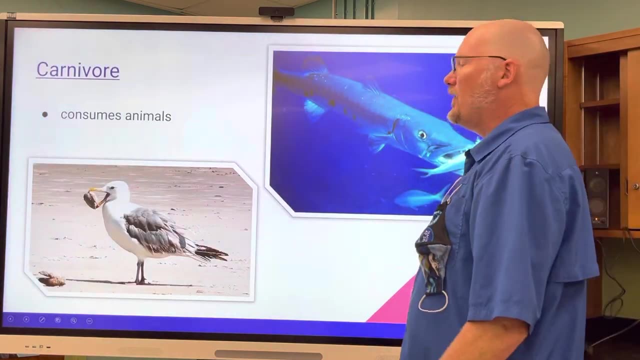 So the these guys consume producers. They are consumers, but they're not carnivores, They're herbivores, right, Eating like a vegans, I guess- of the animal world. And then here's the carnivores, And they consume animals. 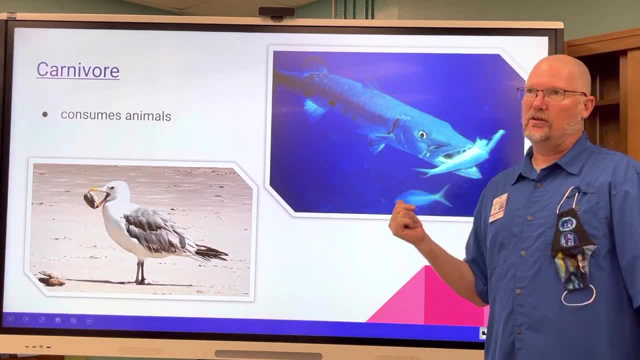 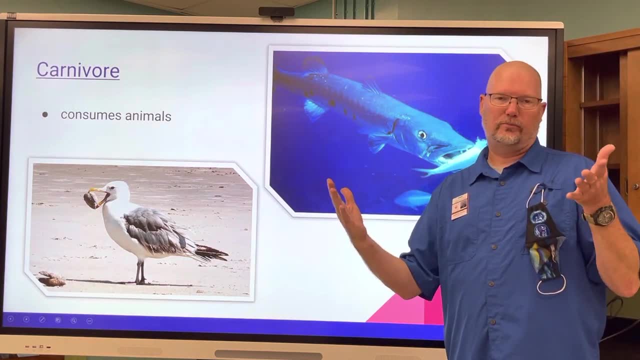 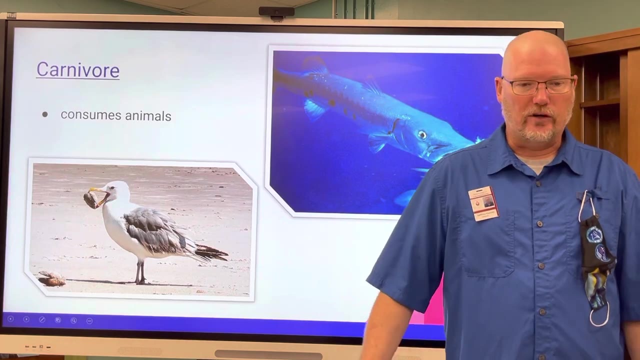 Obviously, here's your barracuda. I saw some of these snorkeling last weekend. They're about this big. I was chasing them. They weren't big enough to hurt you, So and then seagulls, obviously eating a clam, Carnivore eating meat. 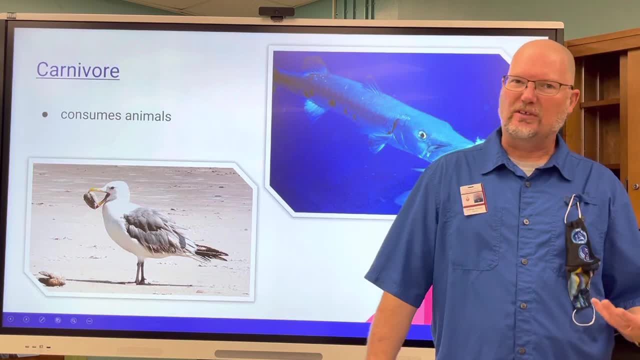 but seagulls are seagulls hunt, but they're also scavengers too. They'll eat, you know, dead stuff. And then we've got omnivores, Omnivores, Omnivores, Omnivores, Omnivores. 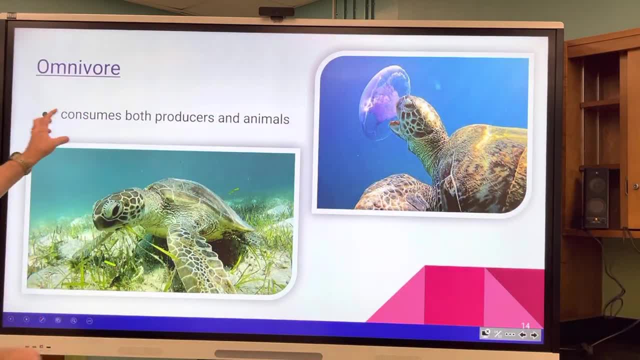 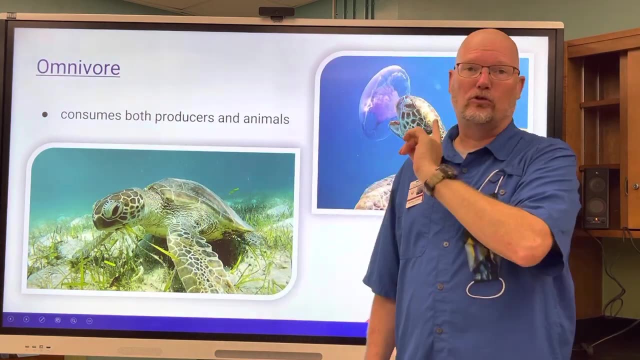 We're omnivores. They eat both producers, which are plants and animals. So here you've got a sea turtle. Sea turtles eat both animals. He's eating a jellyfish. You could see how a plastic bag floating in the water could look like a jellyfish to a sea turtle. 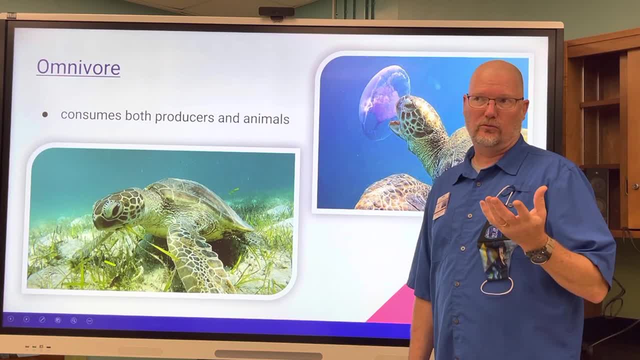 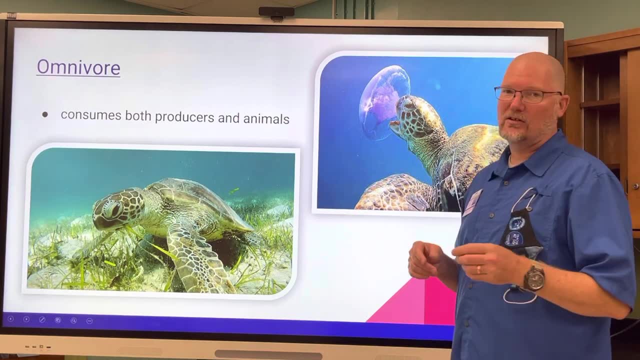 And that's why sea turtle populations are not doing too well because of all the plastic waste. But they love jellyfish And the stinging tentacles don't bother them. It's pretty amazing. And then, of course, they're eating this grass. 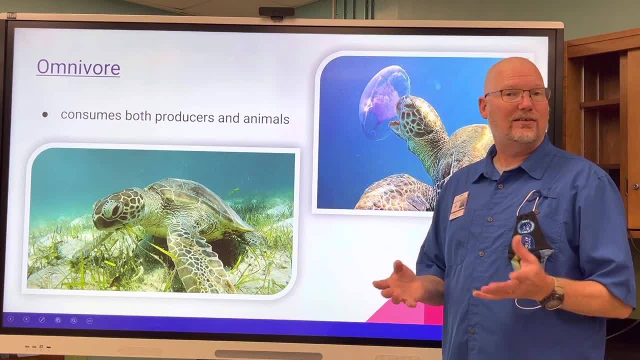 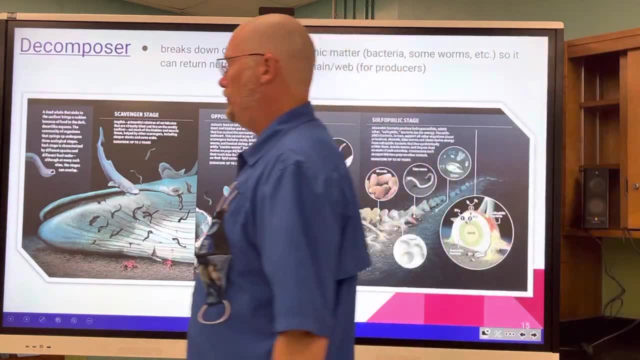 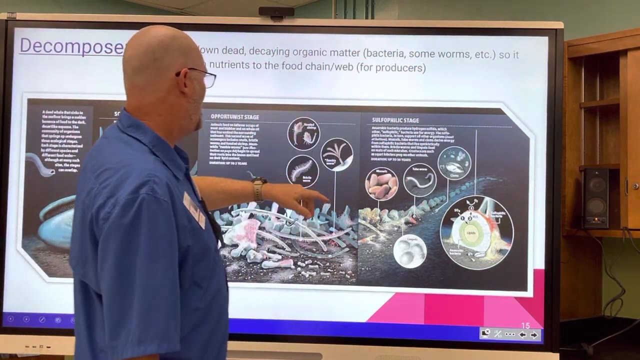 the seagrass the same food that manatees eat, So they're omnivores. They eat both animals and plants. Then you have decomposers. Decomposers are typically bacteria for the most part, but you also have some worms, and here's a bristle worm. 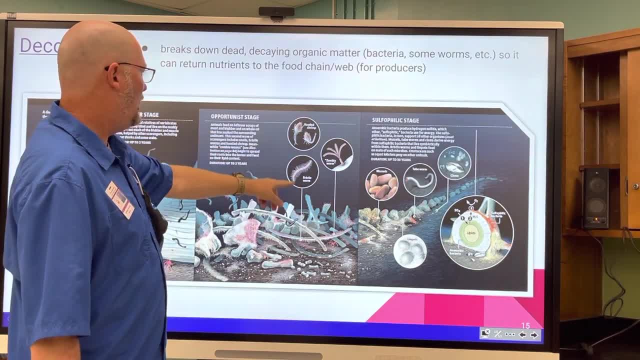 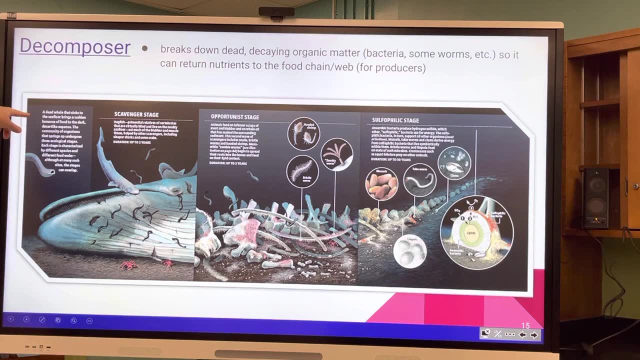 a zombie worm, some shrimp- Okay, Hooded shrimp they're called- And here is a whale carcass. It's at the bottom of the ocean. A dead whale sinks to the sea floor And then you've got these cookie cutter sharks and these other scavengers that come in. 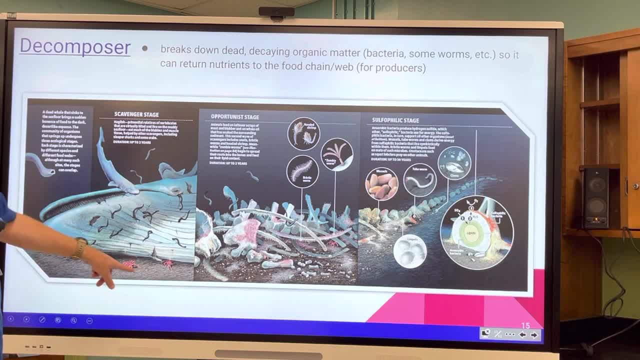 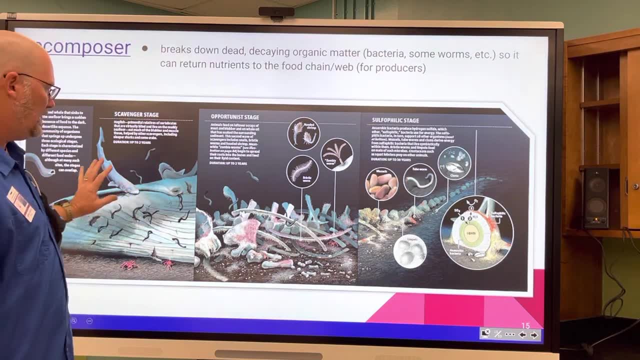 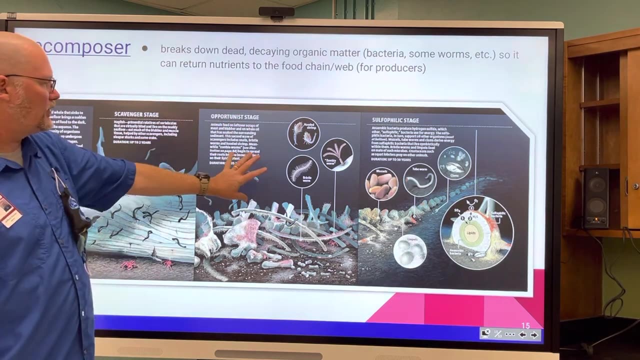 These are hagfish and they come in and they just rip it apart and get crabs, Okay, And then, once the main part is eaten away, then the other parts are broken down as well by these opportunists, And these are your decomposers. 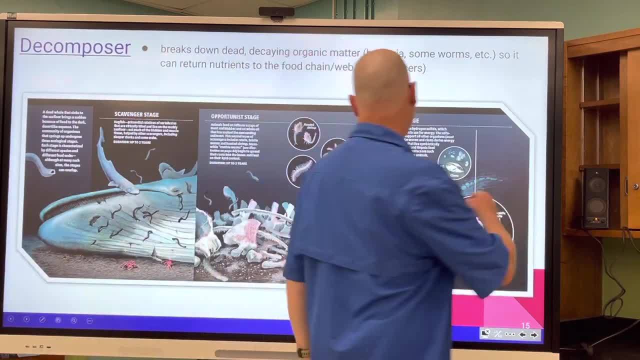 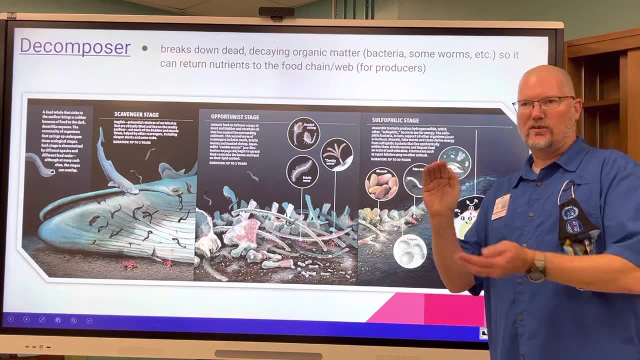 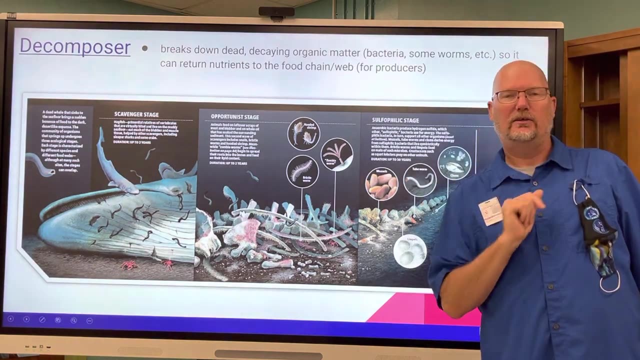 These are the things that are returned. So you've got mussels, two worms, clams, limpets, which are little single shelled organisms that like suck on to something. Okay, You can see them if you go to blowing rocks in Jupiter. 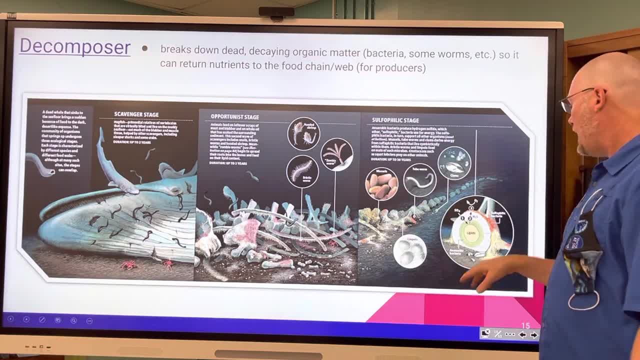 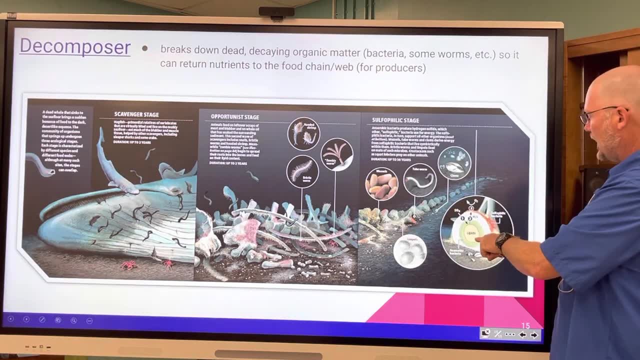 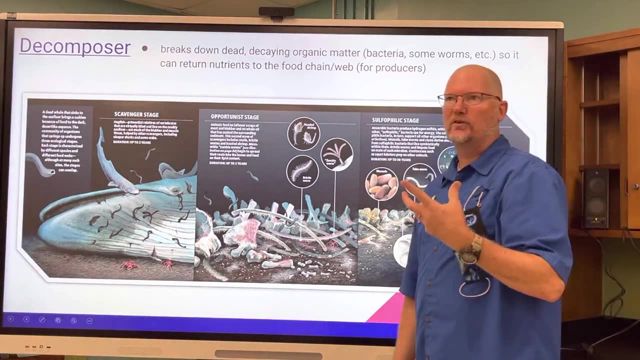 you know, just off of Jupiter beach- We talked about that before- And then you've got bacteria converting everything, not just the meat and the organs, but the bones. now, Now they're inside the bones And they're converting. the bacteria are converting it to new substances that start the whole cycle over again. 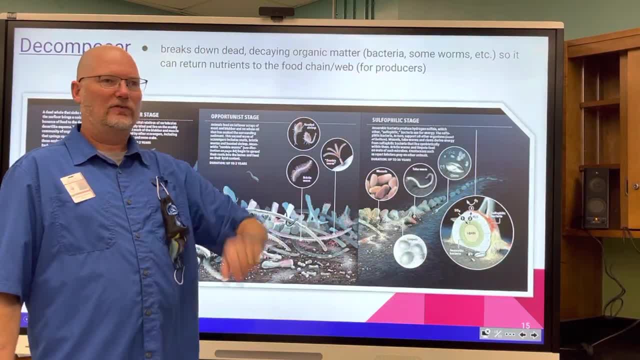 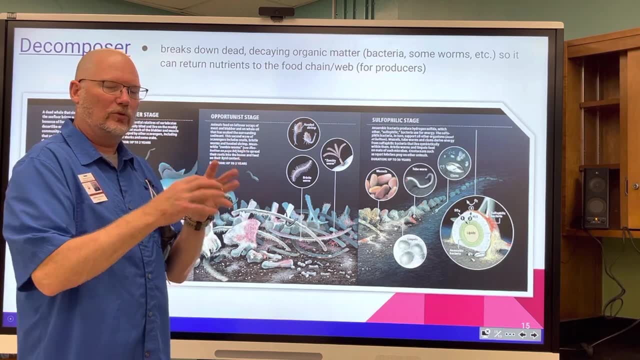 Just like if you put a sandwich outside on the grass and then you came back, you know five days later there'd be no sandwich there, right? Because all the animals would come in and eat it and break it down into nothing. It would be recycled back into the environment again. 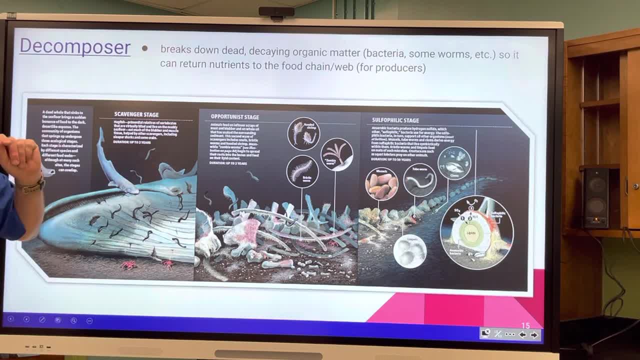 which is returning the nutrients to the food chain. Okay, Um, there are videos. there are videos of these whale carcasses down in the ocean. Um, I think they did a study actually too, because it's, you know, obviously very hard to find a random whale carcass at the bottom of the sea. 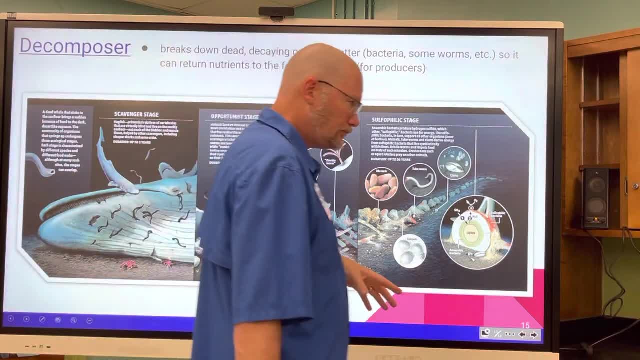 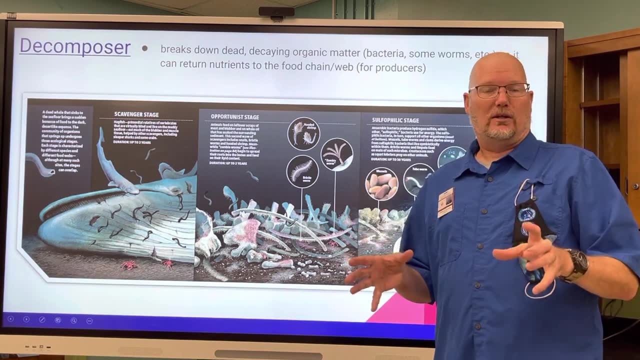 So they found one washed up on the shore once, at least once. they may have done it more than once- And they purposely sunk it where they knew it was going to be, And then they videoed it and they watched it and they they. 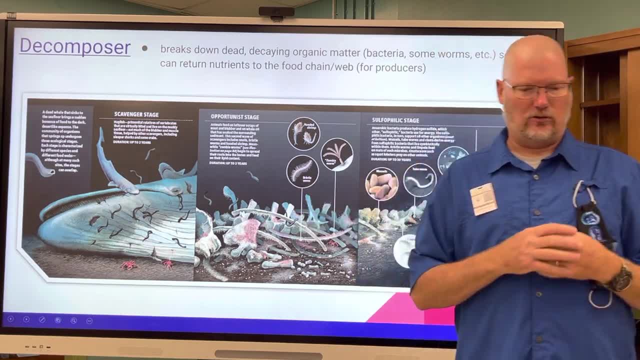 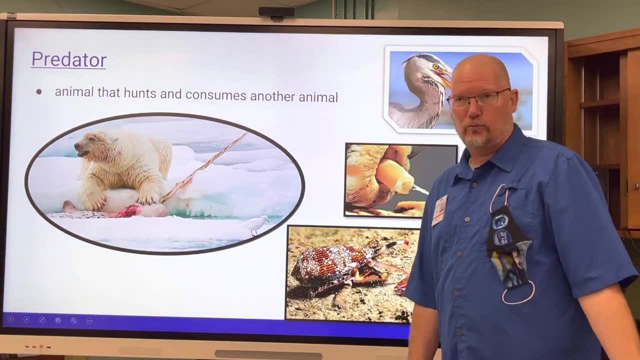 um just recorded and they discovered new organisms and and a whole new process of of recycling nutrients back into the environment. It's really kind of cool. And then we've got the predators, which obviously are carnivores, but um 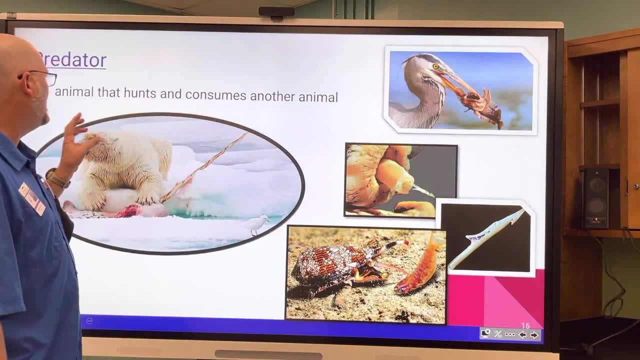 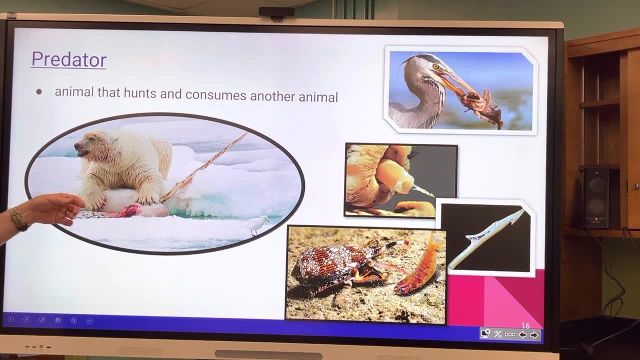 particularly hunting other animals. So to be a predator is one animal hunting another and eating another animal. Okay, So I found some pretty interesting pictures here. Not all of them relate to Florida. I just thought this one was cool because of the um. 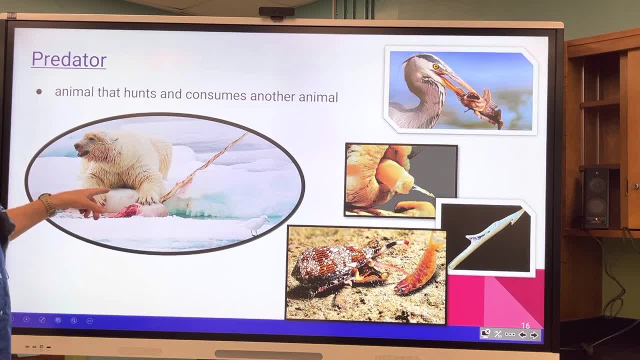 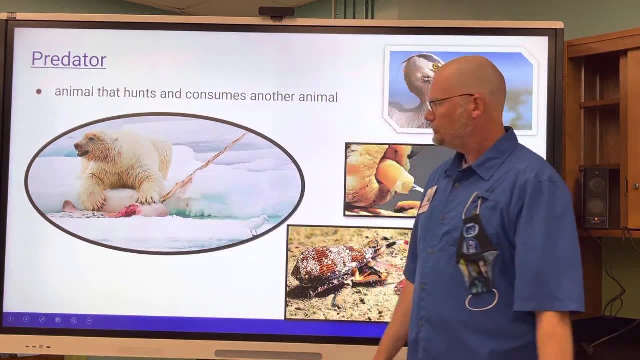 it's like a narwhal being eaten by a polar bear. How did that even happen? But anyway, polar bears happy. um, narwhal is not happy. but do you know the narwhal? This is not a horn. 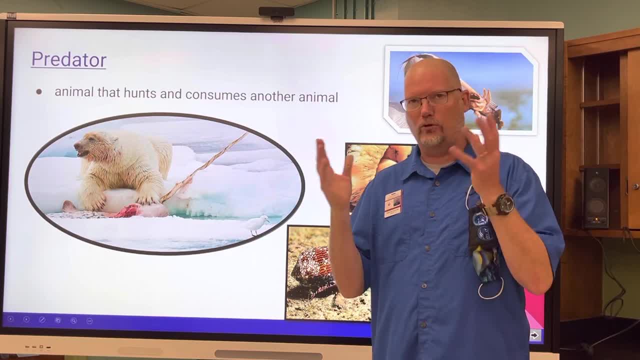 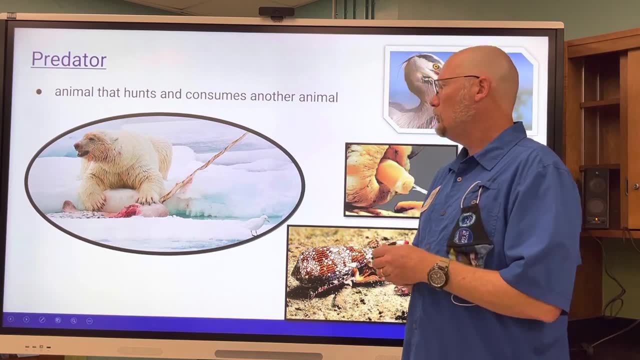 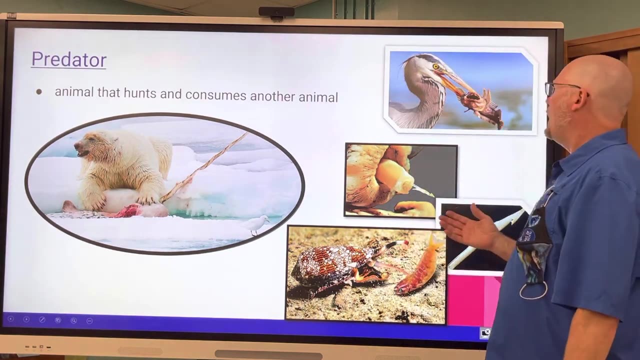 It's always depicted as a horn in cartoons and everywhere commercials- It's actually a tooth. It's a tooth that it's a tusk, really Okay. So don't be one of those people fooled thinking it's a horn. Okay, Like on a rhinoceros or something. 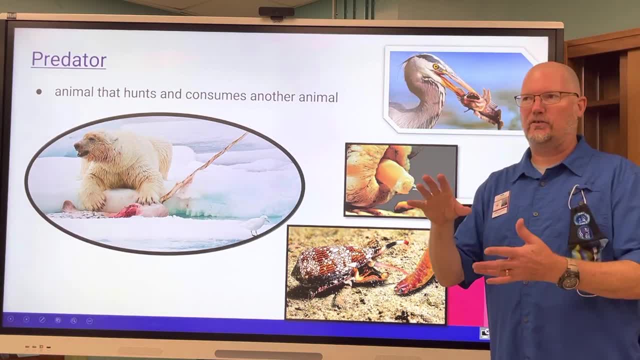 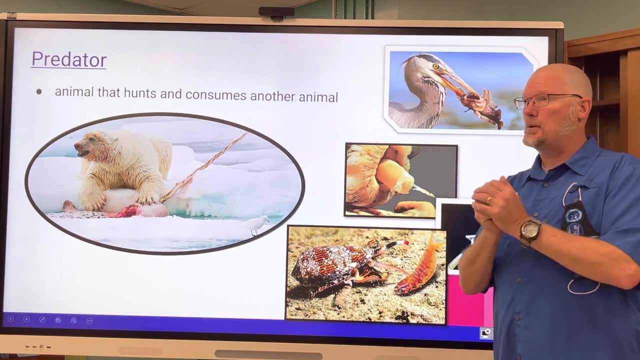 Um, Hey, you have great blue hair. Heron, very famous bird, biggest heron type bird in Florida, possibly the world. I think we've got them all over the place here in Florida. I'm eating a fish, getting ready to eat a fish head first. 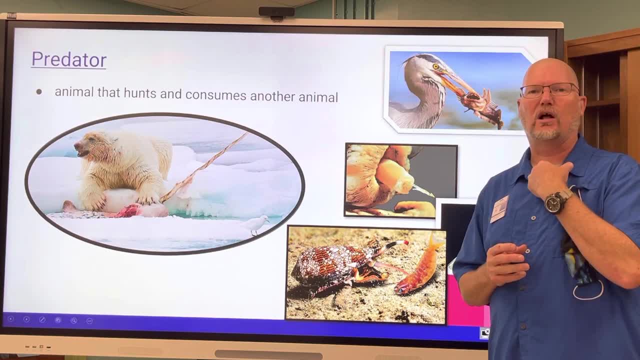 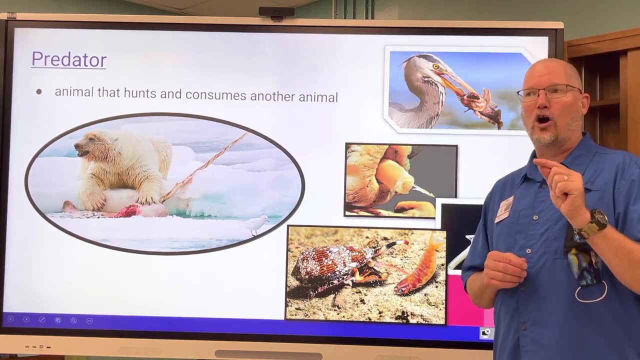 Otherwise the spines would get stuck in his throat. So what he says: to swallow it head first. And then this creature is called a cone snail and it's- it's got a toxic bar, a harpoon that comes out of this. 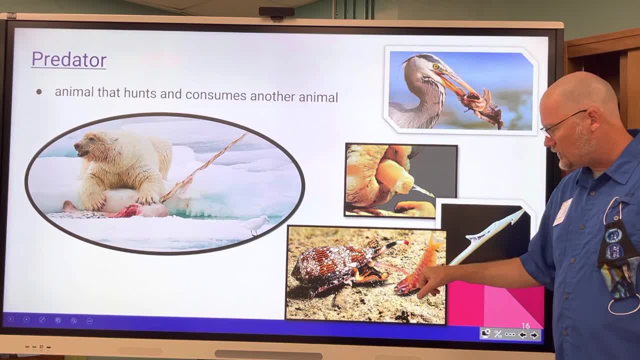 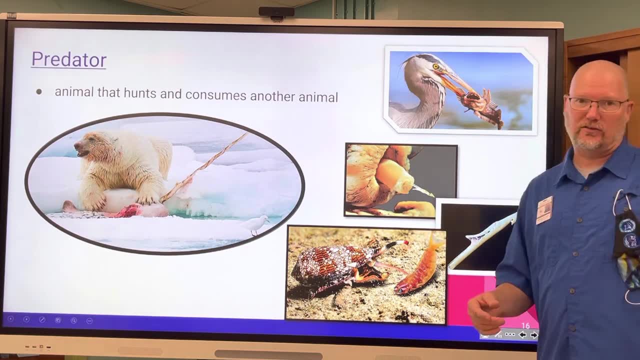 this, this projection of this thing, And it's: it'll stab a fish and inject it with a toxin which makes the fish obviously stop moving, And then the snail has its way with the fish. Okay, It eats, it consumes it. 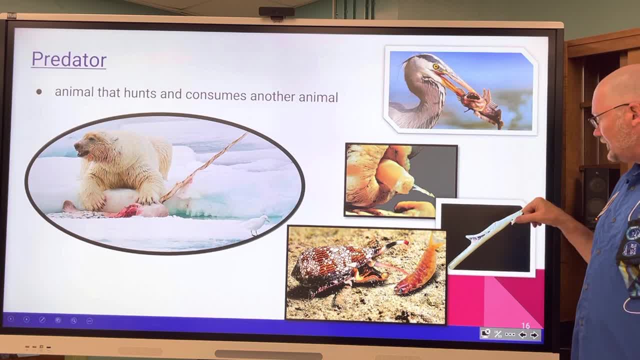 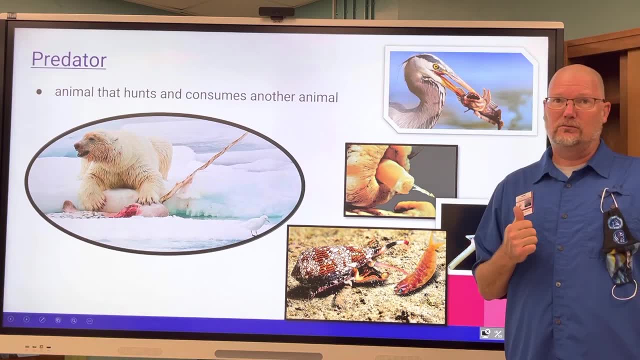 And this is what the harpoon looks like up close. It's literally like a harpoon like for, like hunting whales back in the day. Okay, I wonder if that's where people got the idea from. Maybe, I don't know. 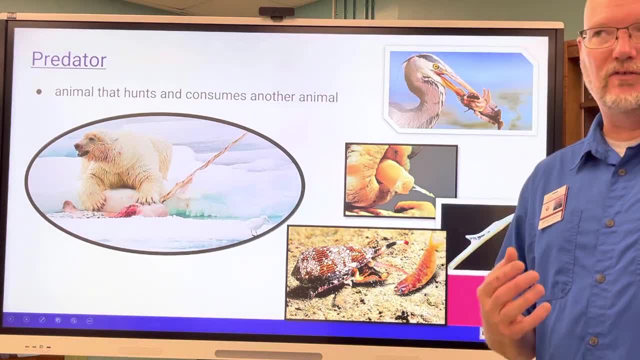 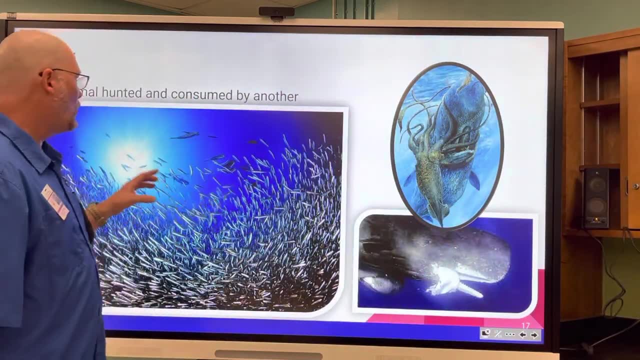 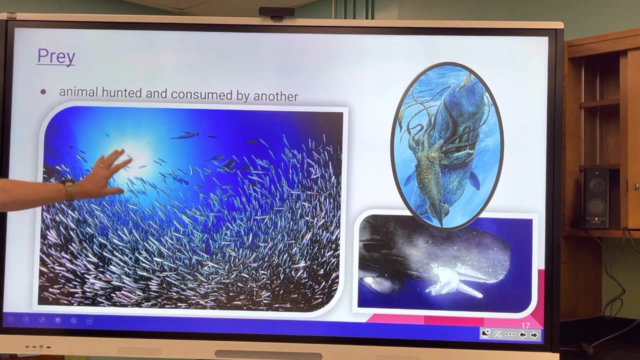 but it's just incredible. It's just incredible To be a naturally formed thing like that. Okay, And obviously the opposite of a predator is a prey organism. And so you've got these fish balls, or, you know, bait balls they're called. 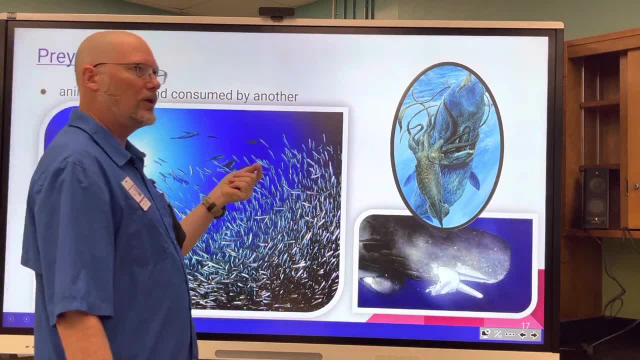 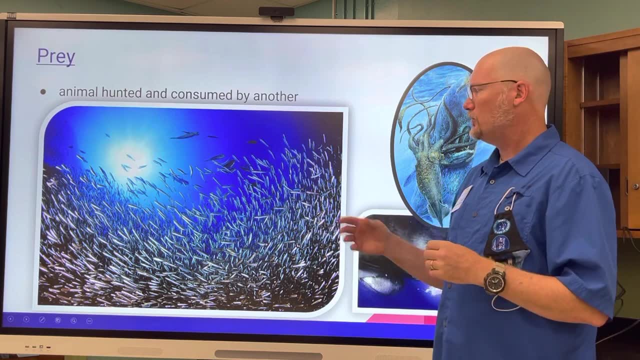 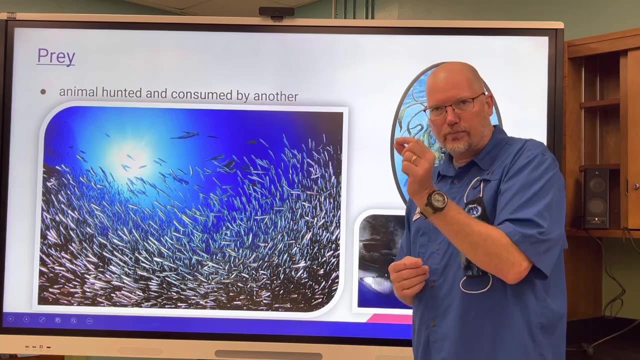 We watched them. when we, when we were watching the underwater live feed from the Deerfield beach pier, We watched these guys swimming around. These are herring, Okay, And they are prey fish. They still don't eat their own prey- teeny, tiny things in the water. 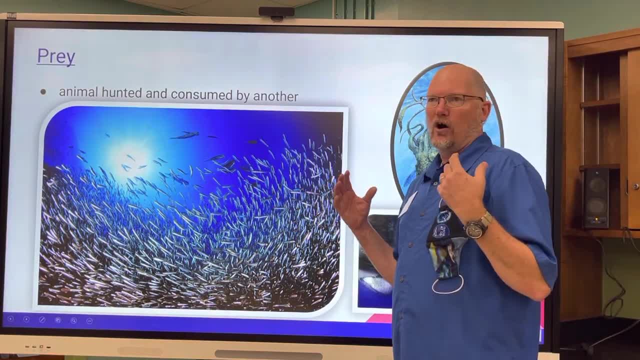 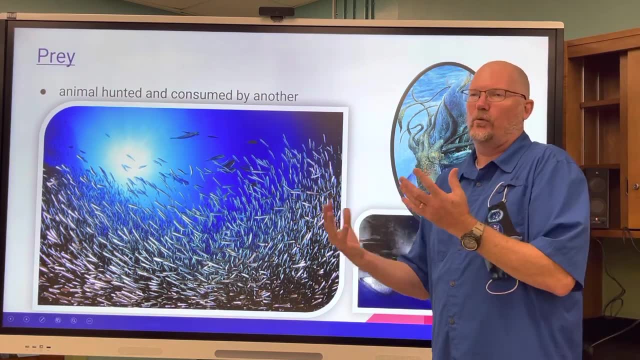 plankton and stuff, but they are they pretty much everywhere. Anything eaten by something else is prey. So even a shark could be prey, even though it's also a predator. And then I chose this one because no one's ever actually seen this before. 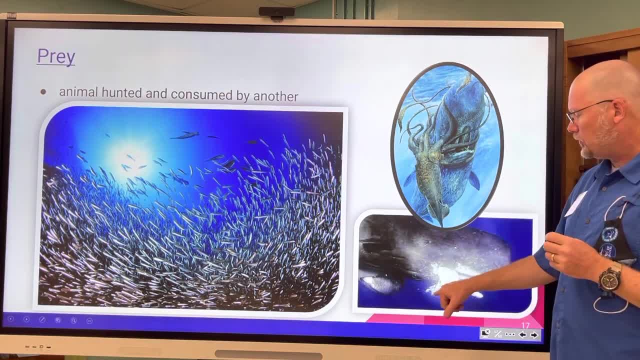 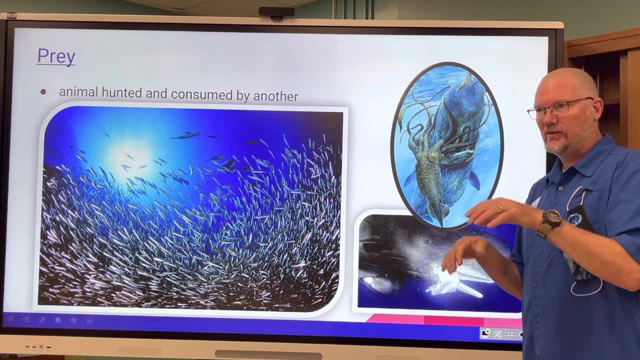 but we know what happens because we have- this is probably the closest picture we have- to a sperm whale. Okay, Having just won a battle with its prey deep on like a mile deep in the ocean, That's where they find these giant squid. 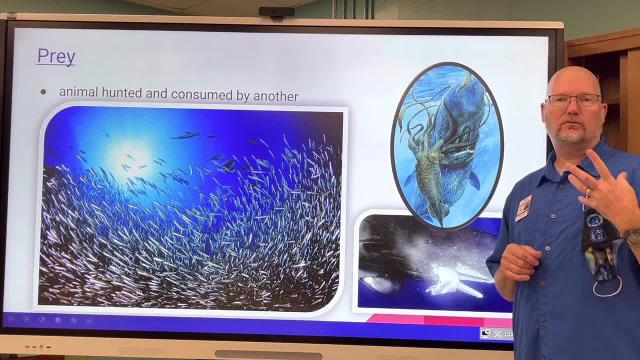 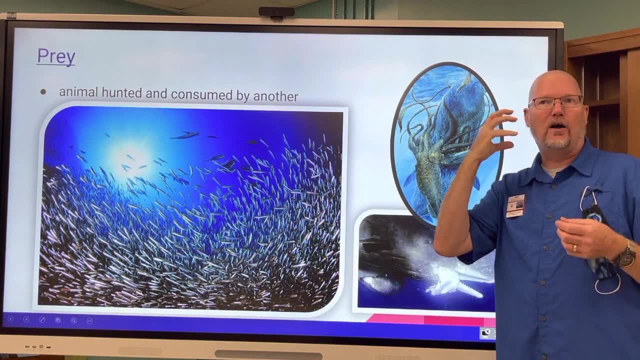 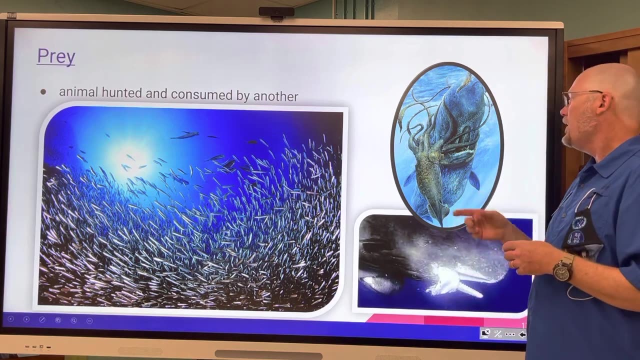 And we know that they have these battles to the death down there because most sperm whales- adult sperm whales- have sucker scars on their bodies, from where this, this squid is trying to. you know, get out, get get away. And then whales that were harpooned back in the day. 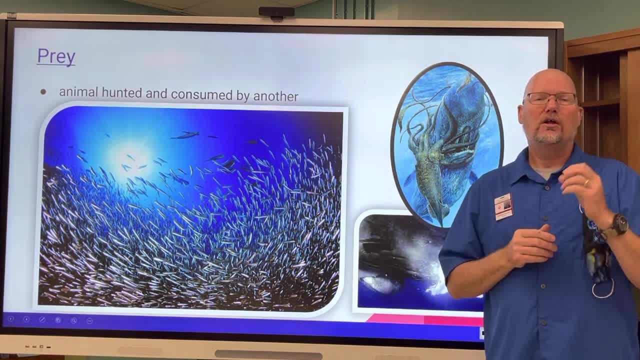 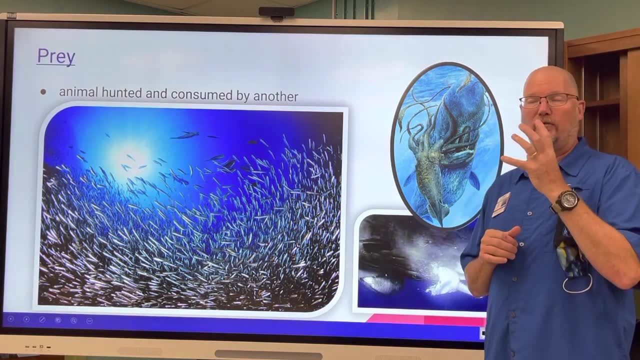 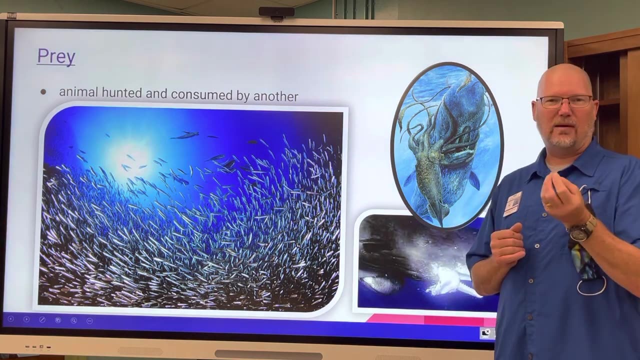 or washed up on the shore. when they do a dissection, they find the beaks- undigestible beak of the whale, sorry, of the squid in the whale's stomach, And it's like made it of a very strong. 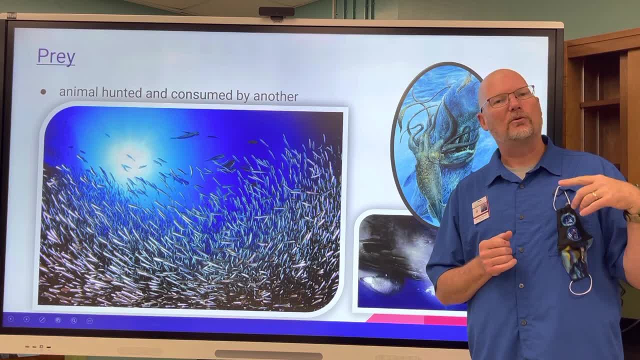 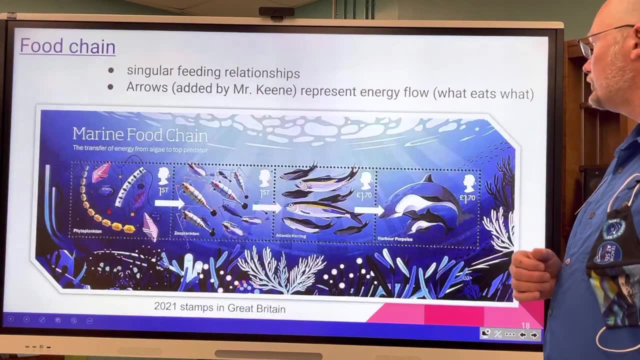 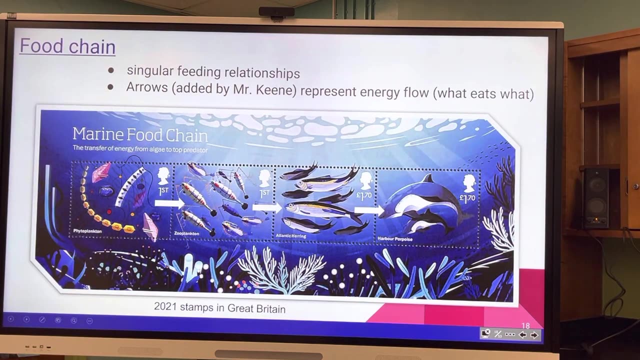 it's made it of kind of what a shell of a crab is made out of. So it's, it's hard to digest. Hmm, Food chain. now, moving on to the food chain, So we're on slide 18,. just for reference sake. 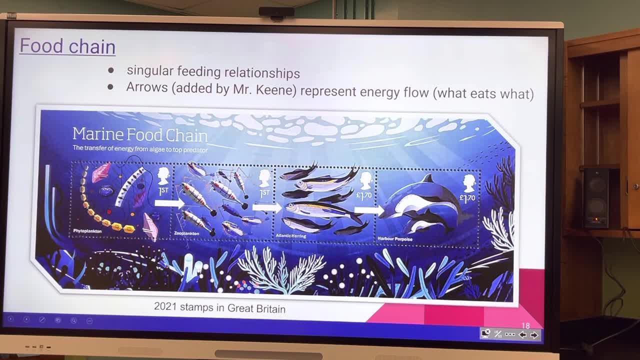 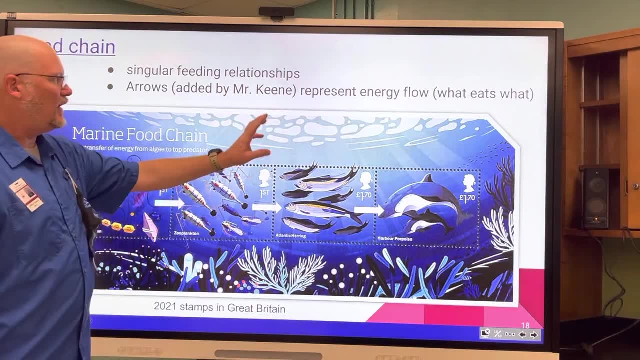 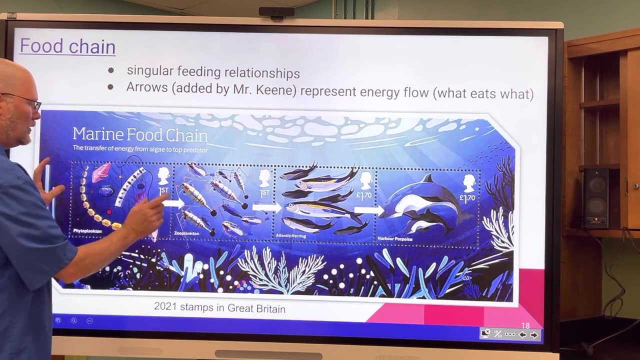 So the food chain shows a singular feeding relationship And the arrows here on this picture I added those. they represent the energy flow and what eats what. So the energy is going from this level to this level, to this level, to this level. 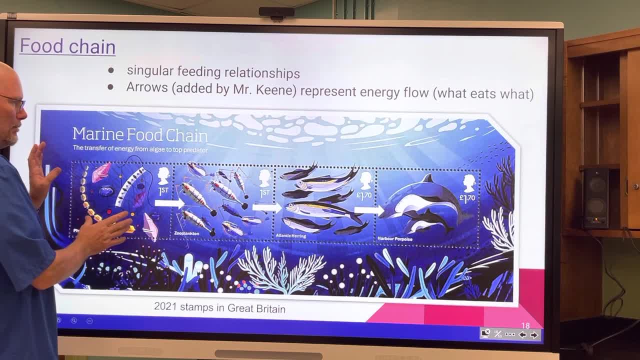 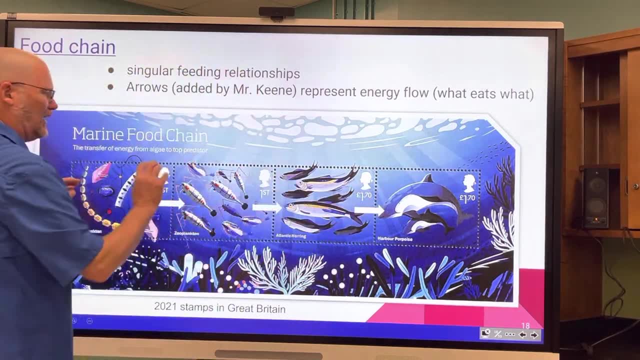 It's a chain right And uh, we're going to learn that there's a lot more of these and then there's less of these, and less of these and less of those, And the picture kind of depicts that. What I thought was neat about this is that it's from Great Britain. 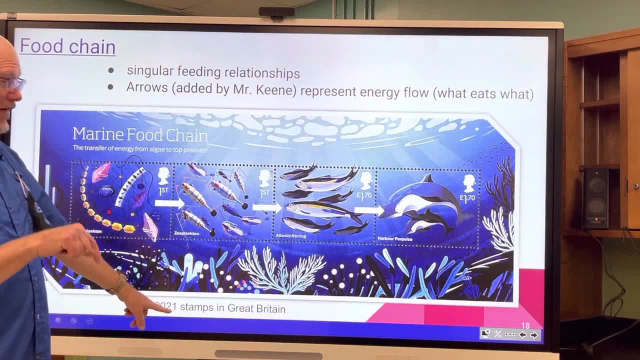 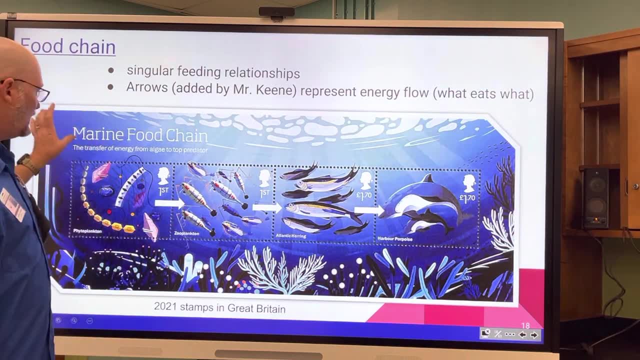 and that there were stamps that are coming out this year or came out this year. You can probably order them from somewhere, I don't know, but these are stamps for postage And they chose a marine food chain for their, for their stamps. 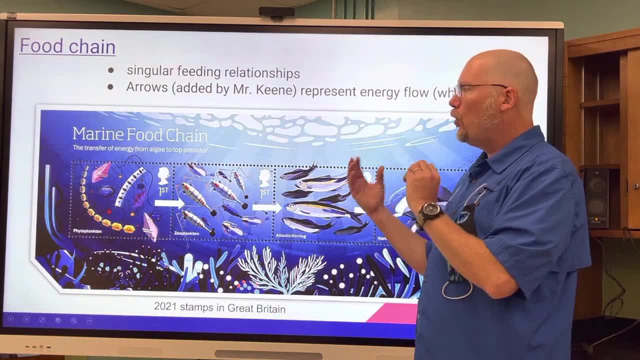 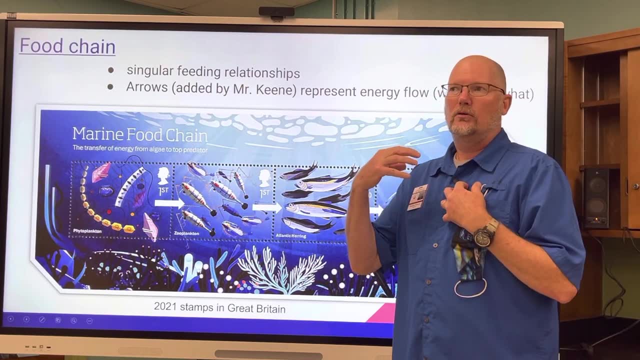 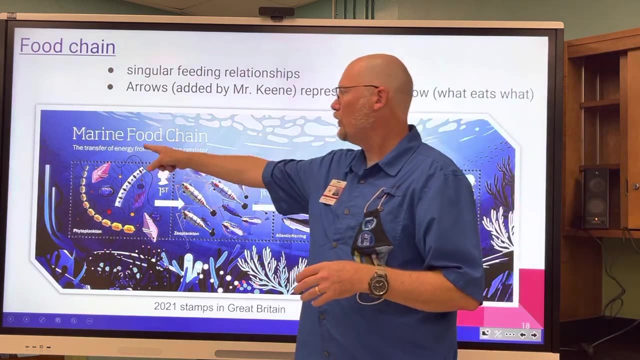 That's I think that I just thought that was really cool. That's how important this concept is to understand because of the way humans treat the environment. That's important to know all the relationships. Okay, And so it's a transfer of energy from algae to a top predator. 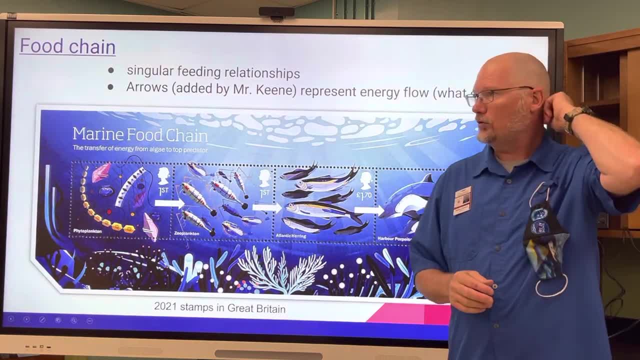 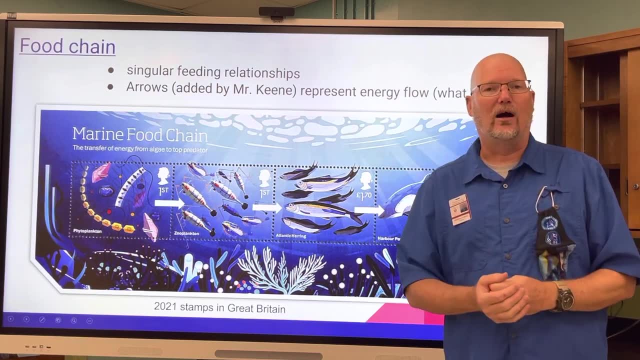 That's really what a food chain is. It's simple. You can make them from virtually any animal that you choose And you choose in the sea. It's going to be involved in some kind of food chain- Not virtually every animal. 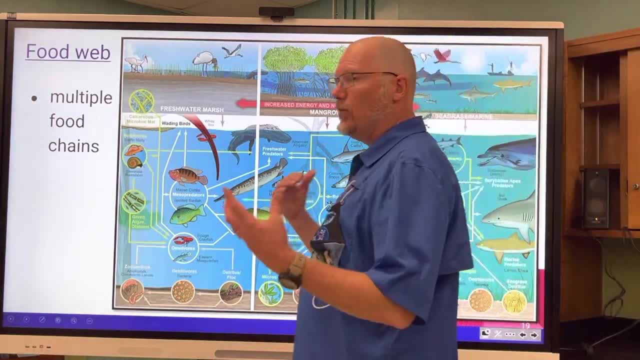 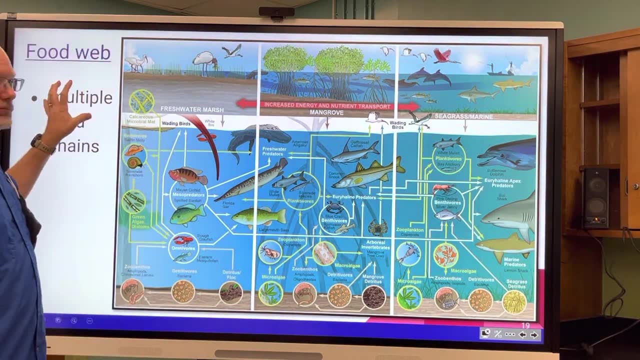 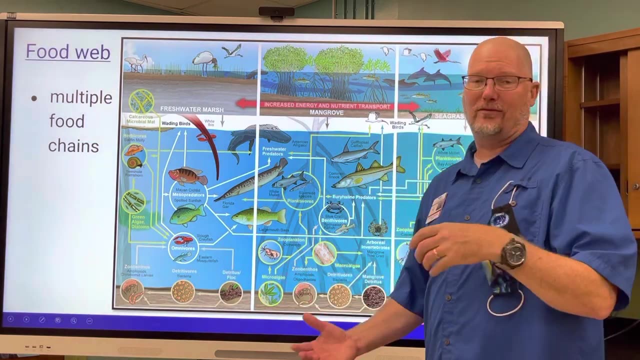 Okay, Here's the. and then, if you take multiple food chains and you put them together, you are going to get something called a food web. Okay, And here is a very complex one. I chose this one to show you, and this is by far not even close to everything that's involved here. 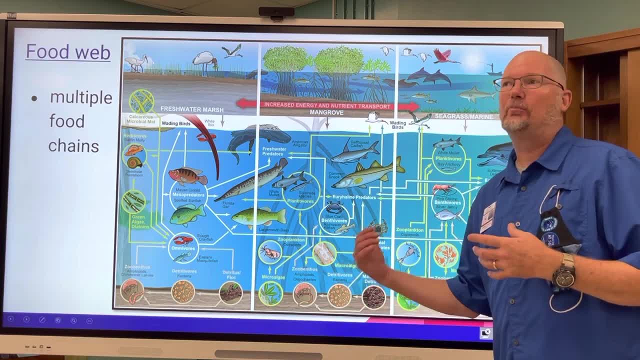 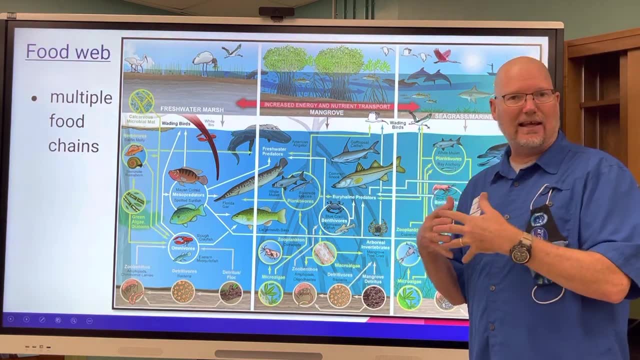 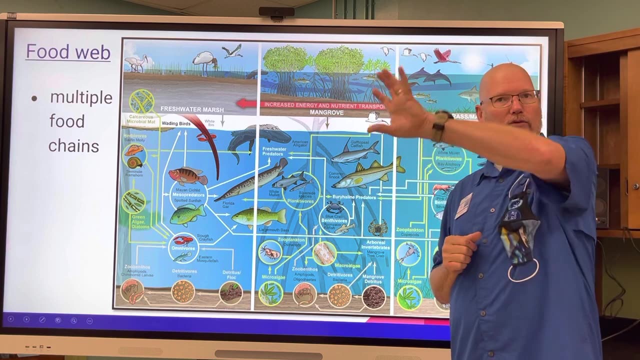 This is just showing a smattering, a sampling of the organisms that can take place in these and how everything is related. So here you've got mangrove swamp, Okay, Or mangrove. We have mangroves all along the Intracoastal, right here. 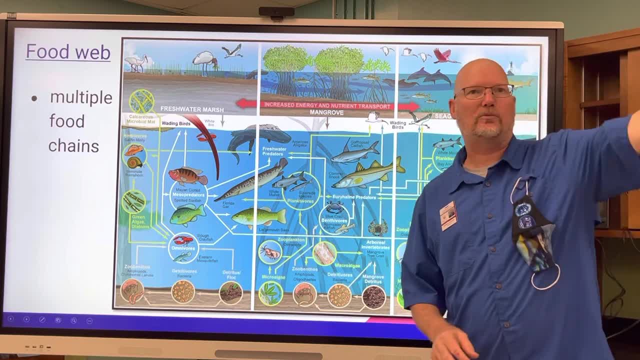 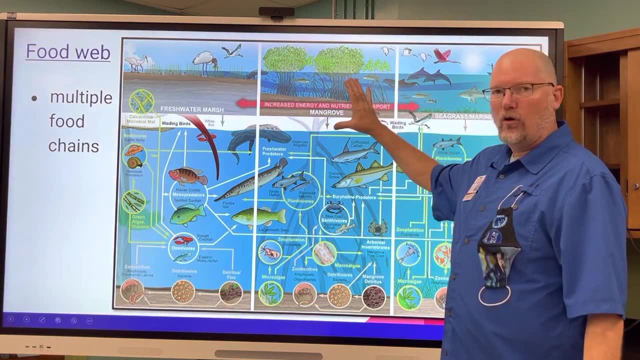 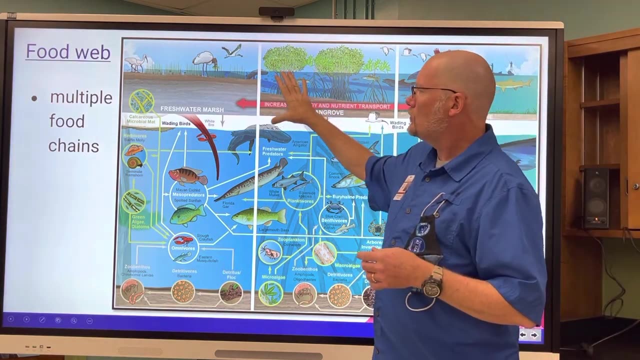 Boca Raton, and North and South, all the way down to the Keys and all the way up to North Florida. Okay, Mangroves are in estuaries- Remember that mixture of fresh and salt water. And so on one side of them, 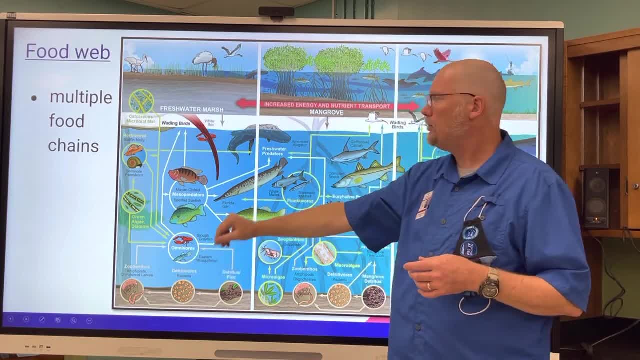 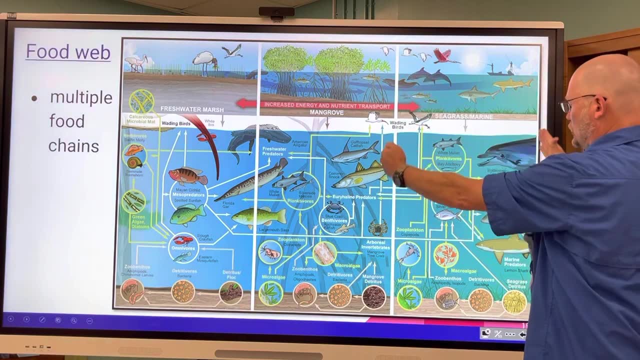 you're going to get fresh water species, which we're not going to talk about, And on the other side, you're going to get the salt water species which we are going to talk about. That's why, on your notes, This section is: 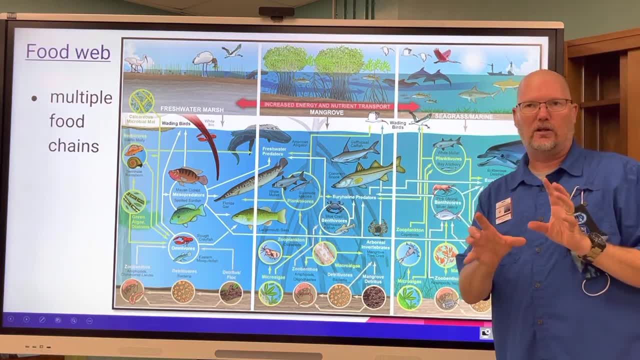 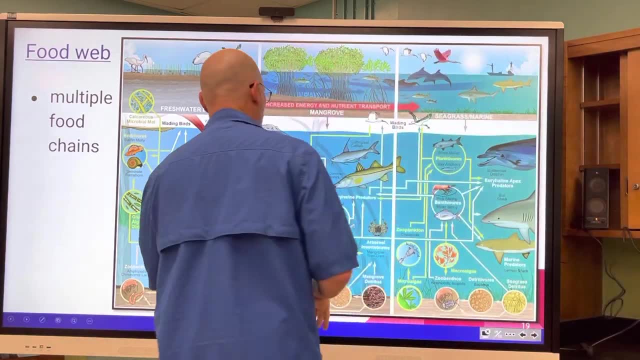 is has been separated and included and you have to label parts of it. So there are three parts on here that you have to label and but but really it's to show you how complex if you take all the food chains or just some of them. 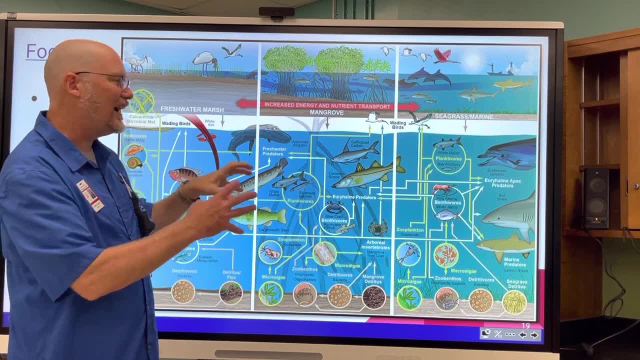 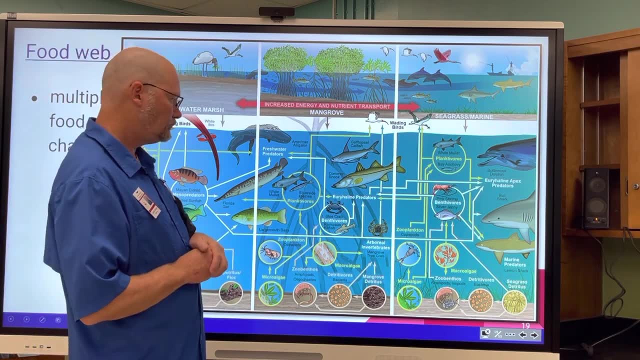 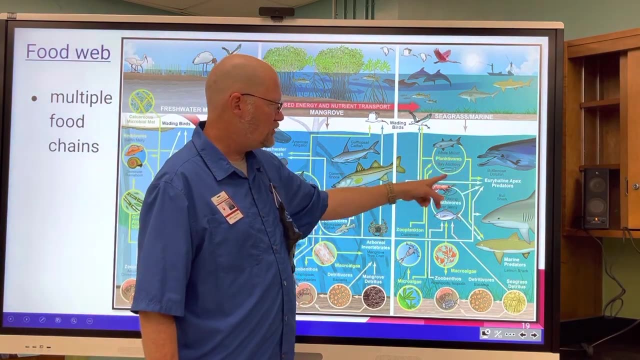 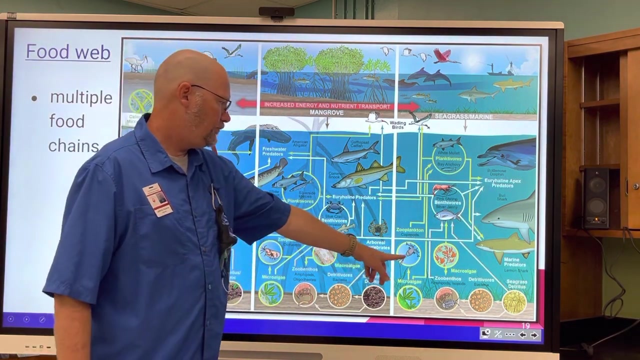 and you superimpose them on top of each other. how quite amazing it all is, Okay. invertebrates, vertebrates, bony fish, bony mammals, cartilaginous, no bone fish, tiny zooplankton and algae. 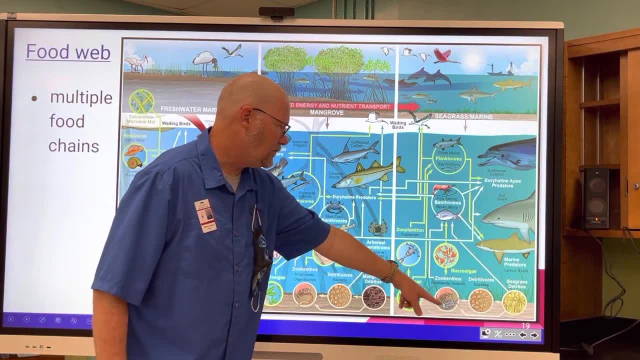 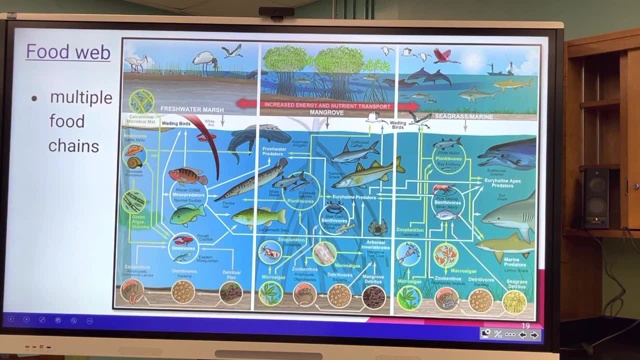 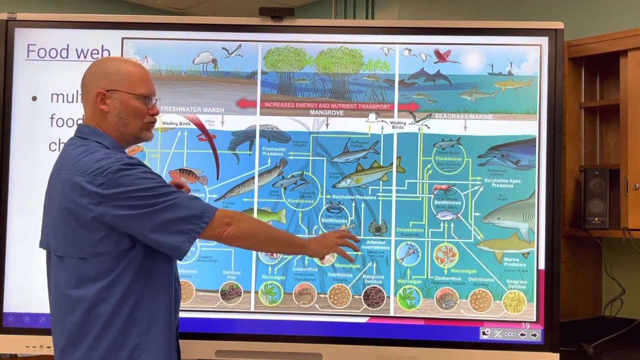 and all these Arthur amphipods and bacteria and seagrass And just all of it's. just they're all involved together. So if you pulled one out, you would affect everything else in the chain which really is connected to other chains. 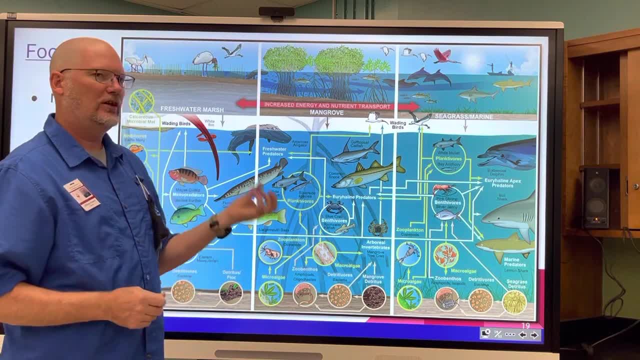 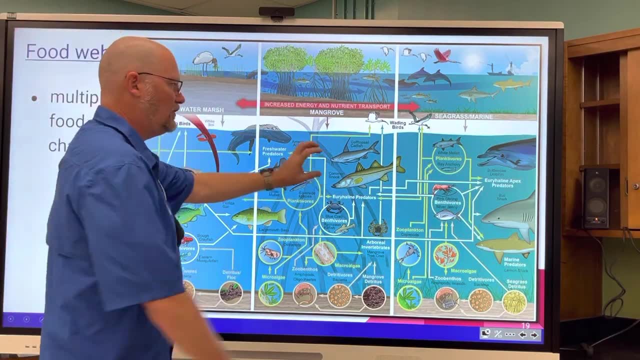 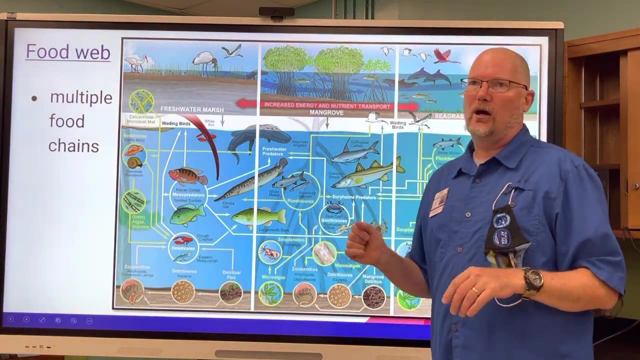 So it's a really complex system that people don't really understand. That's why why invasive species are problems And and when you introduce a new species, it just offsets the whole thing, Like lionfish, for example. lionfish escaped in a hurricane. 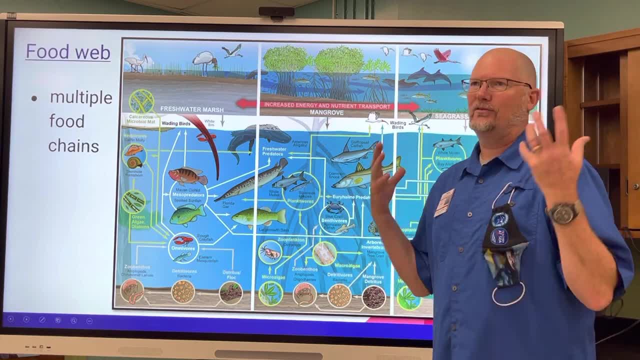 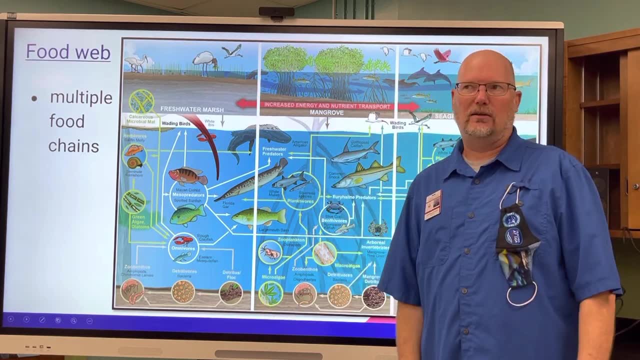 so many years ago- not too many years ago, but in the last 20 years or something like that- from down in Miami a big tank overflowed and all the lionfish escaped and they're eating like everything. So that's an invasive species. 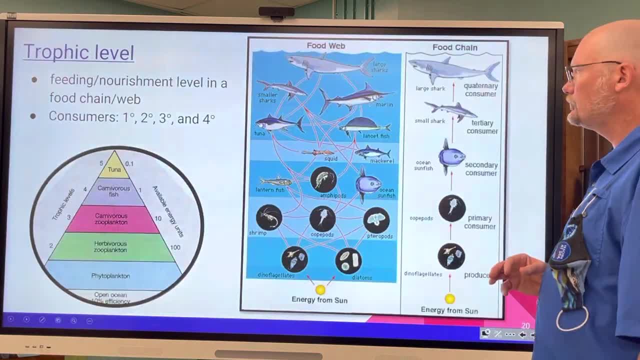 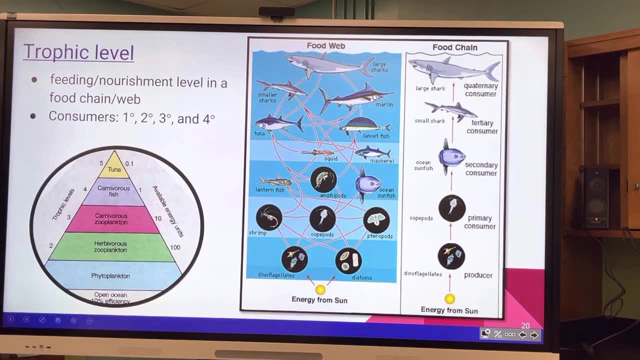 That's affecting the food web here in Florida, And then trophic levels. So you've got some filling out to do here. Okay, on your notes, This is the feeding or nourishment level in a food chain or web. So here's the food web. 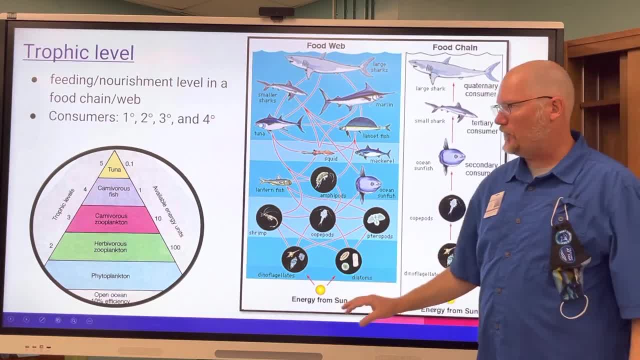 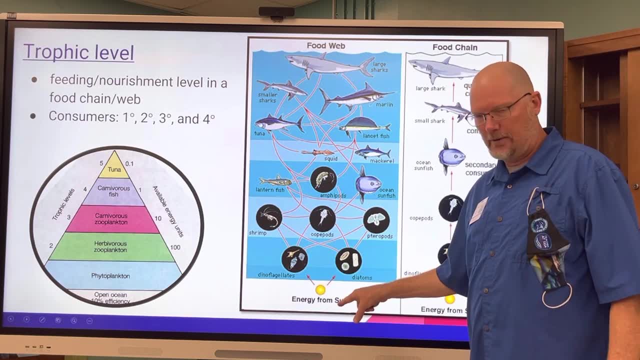 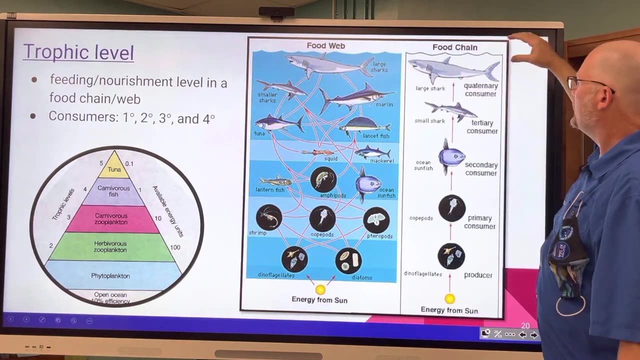 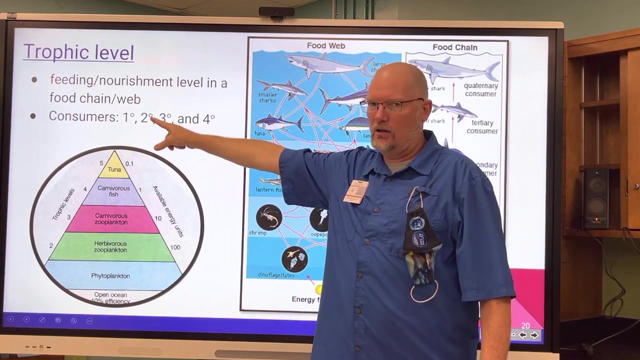 Okay, another example of a marine food web, with the producers on the bottom making food from the sun right And you go up the different levels to the top predator. Okay, And so these levels are called primary, secondary, tertiary and quaternary. 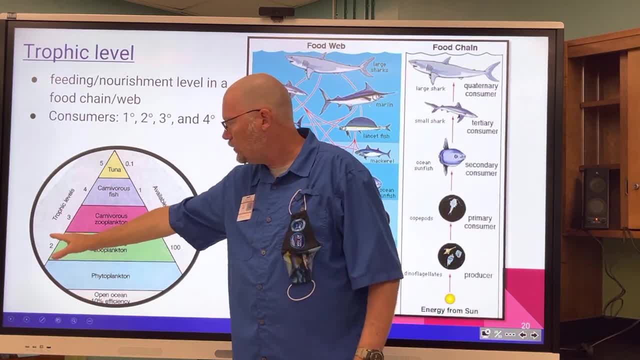 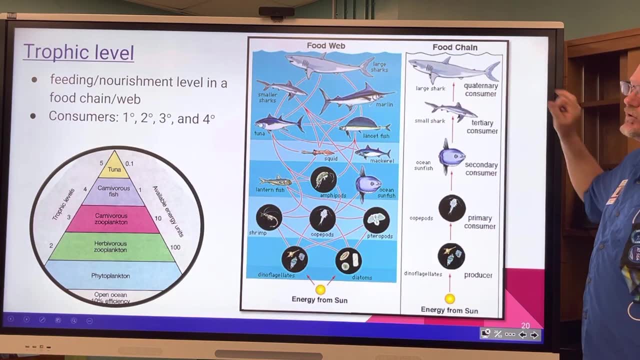 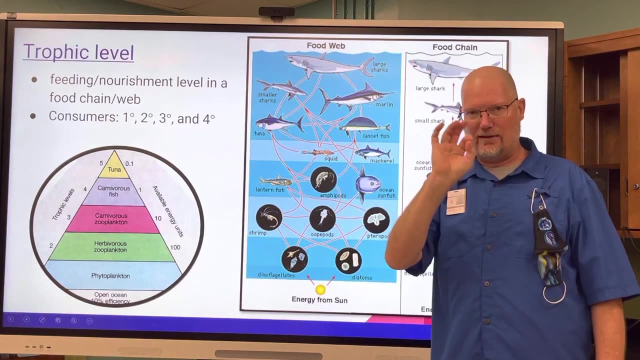 Okay, and they're here as well. So these are the trophic levels and you've got primary, secondary, tertiary and quaternary, Quaternary consumers And this is just an abbreviation for them. So please notate that on your paper. 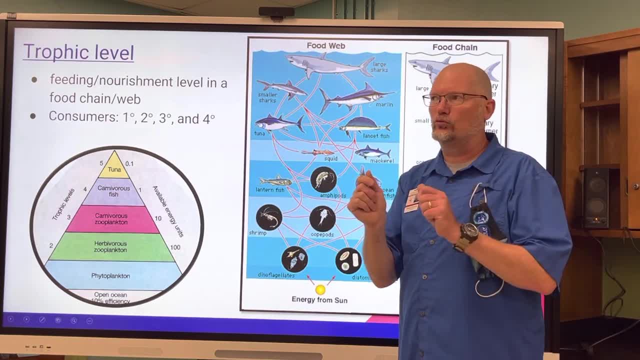 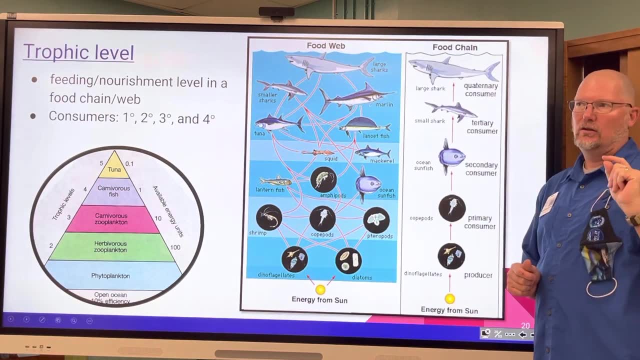 What those are, because you have to fill them in on the blank. But if you don't know what you're writing, if you don't know that that means primary, secondary, tertiary, quaternary, then perhaps on a future test you might be rather confused why you don't know the answer. 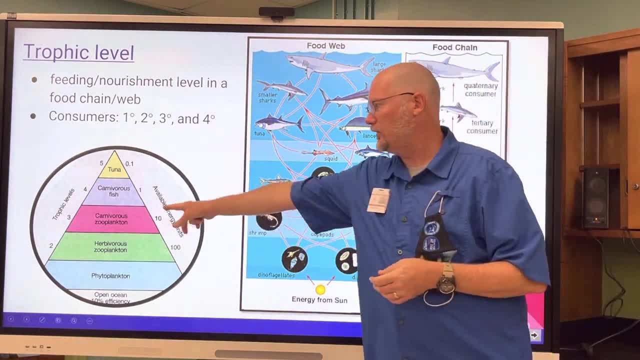 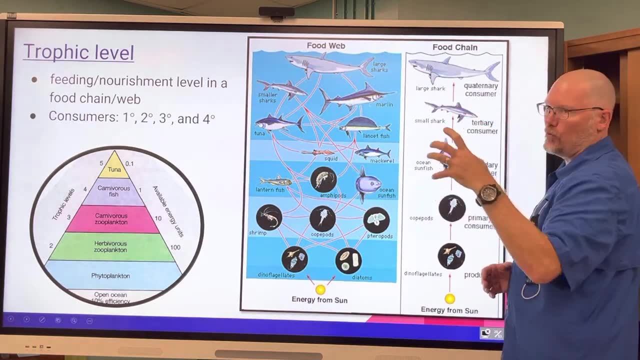 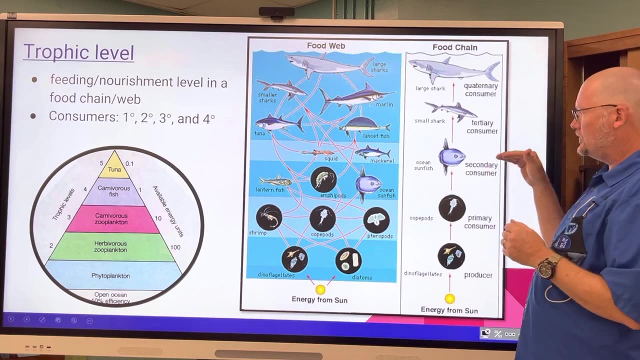 Okay, so please notate that as well. It's filling in this information here that's missing, So anyway. so this is a chain pulled out from the web, and then you can analyze it by telling what the successive levels are in this energy pyramid. 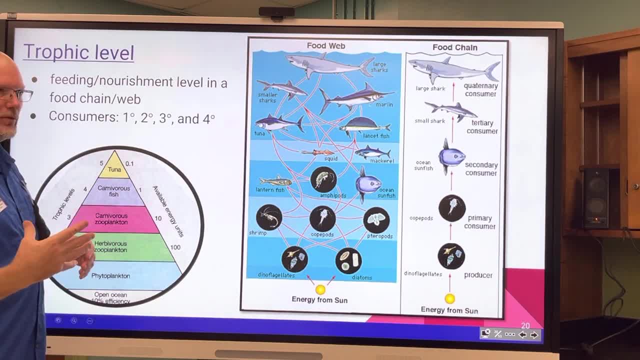 Okay, and if you- I don't know if you remember from maybe your environmental class or biology- that this 10% rule. So if I have a thousand units, this is supposed to be a thousand year of energy. I'm only going to get 10% of that energy in the next trophic level. 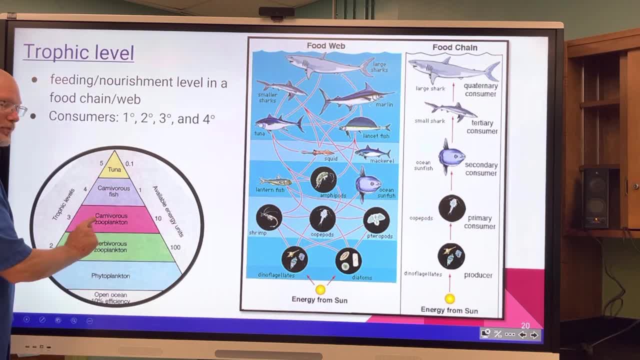 and then 10% of that energy is available to the zooplankton in that level and only 10% for the fish and 10% of that for a bigger fish. Okay, so that's what energy trophic levels are referring to. 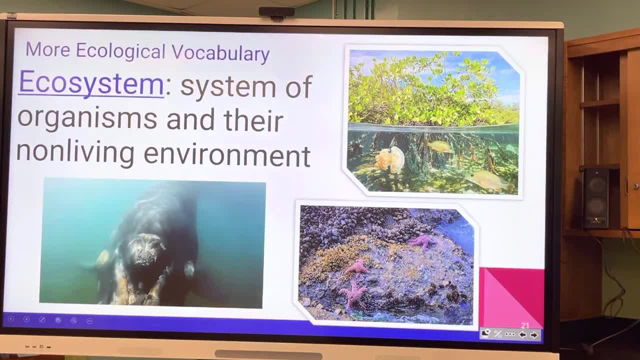 Okay, All right, Here's some more Your vocabulary: Holy cow, All right. So an ecosystem, What is an ecosystem? And we're going to be talking about all of these separate ecosystems in the future, in the next, I believe in the very next unit. 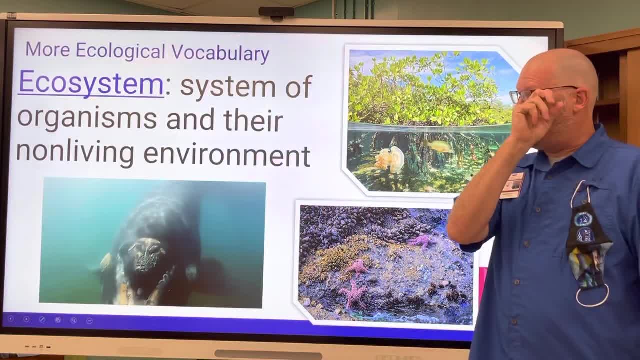 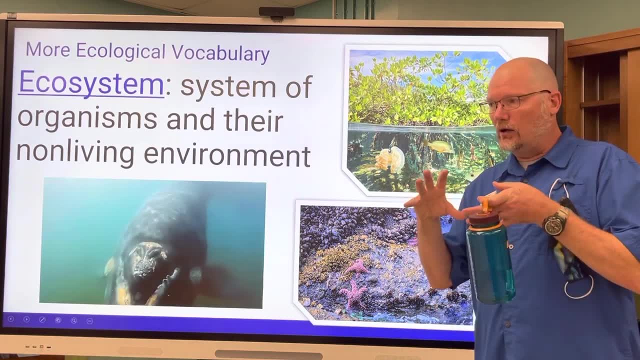 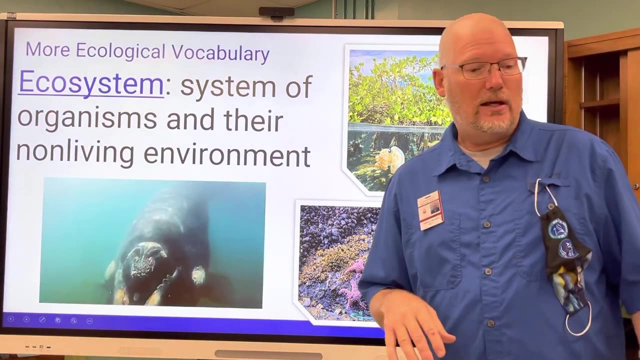 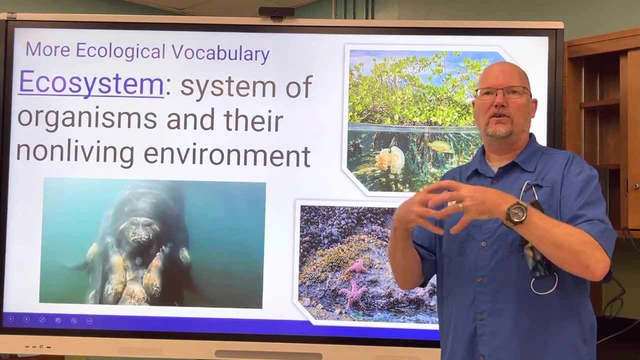 So it's a system of organisms and their non-living environment. Everything that's alive and everything that's not alive that occurs in an environment is an ecosystem. Okay, So ecology is the study of ecosystems. It's a study of how the living and non-living things interrelate. 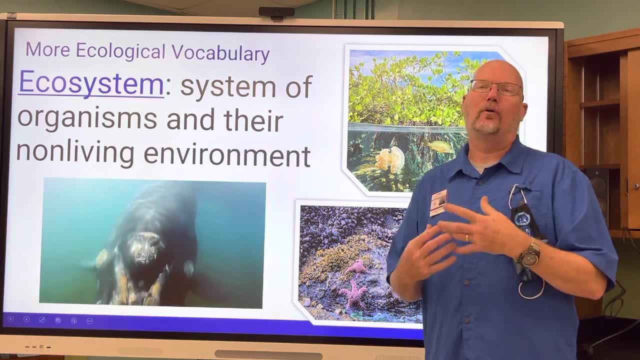 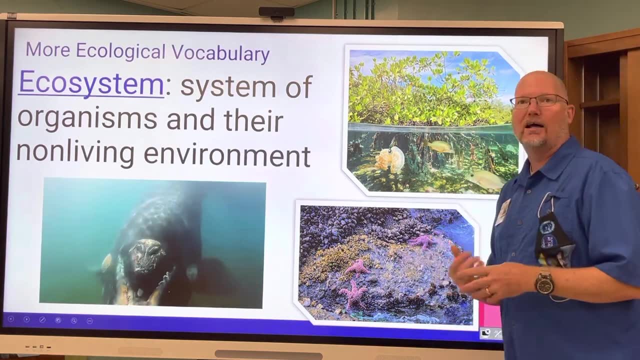 and react to each other and need each other to survive. Well, the non-living things don't need anything, but it's how the living things interact with the non-living things. So let's point out some non-living things here. 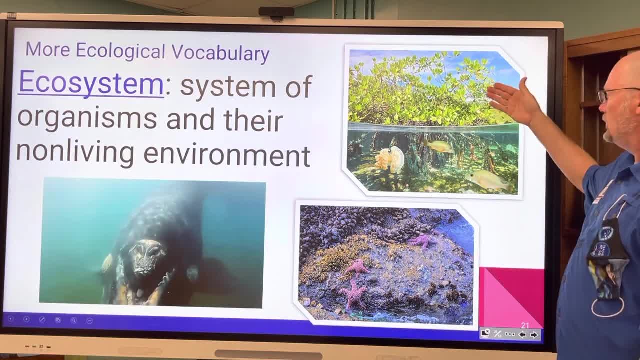 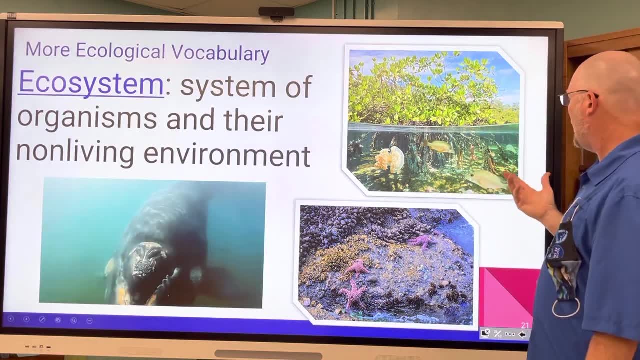 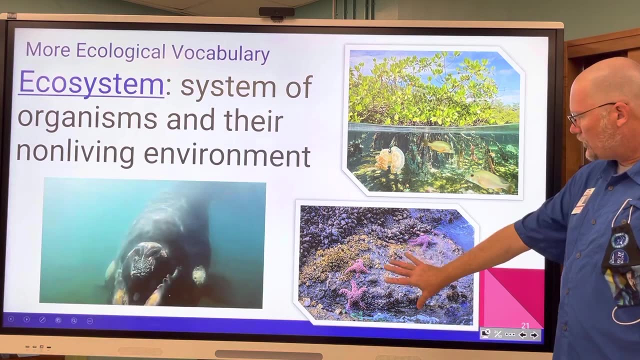 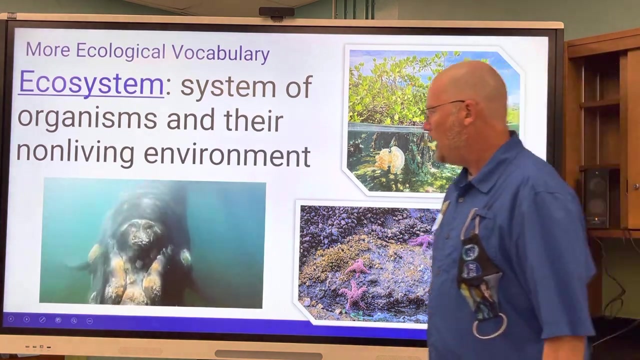 Okay. So what do we have here? What's non-living? Okay, The water, obviously, The air and the clouds, And maybe some sand down here on the bottom. Okay, And that's probably pretty much it. Here we have the water and rocks, because these are all. everything else is alive. 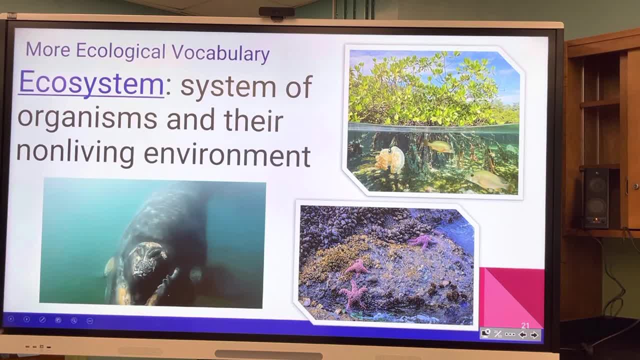 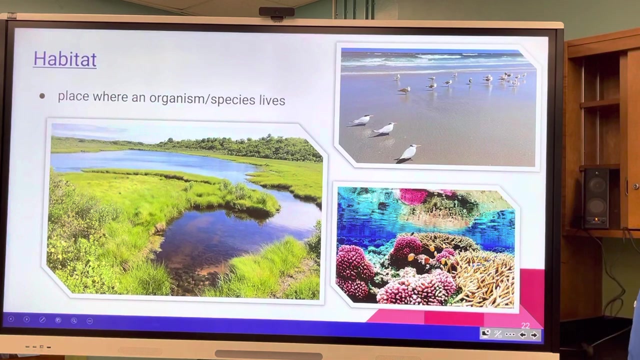 And here, what do you see? here? The water again. obviously Those barnacles on this- I believe this is a right whale- Are are alive. So you can't count those. but the sun dappling on the sunlight is obviously a part of the non-living environment. 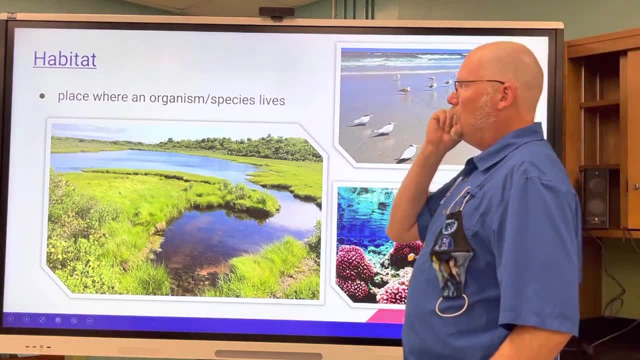 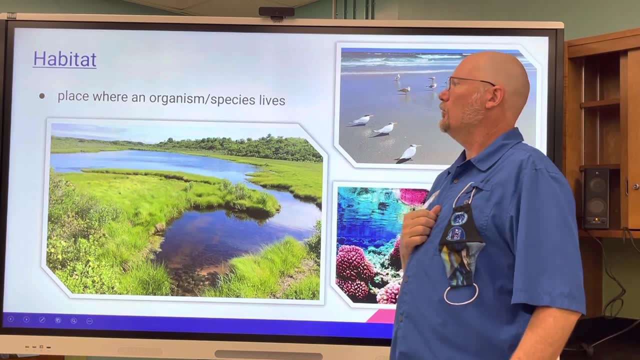 Habitat. What is the? what does it mean to be a habitat? Habitat is a place where things live. That's it, Habitat. Okay, This is a saltwater marsh habitat. This is a saltwater marsh habitat. This is a saltwater marsh habitat. 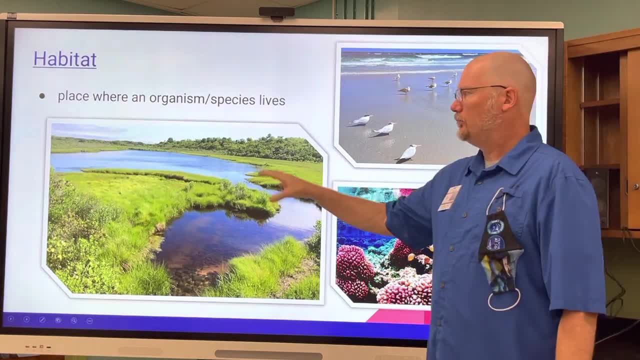 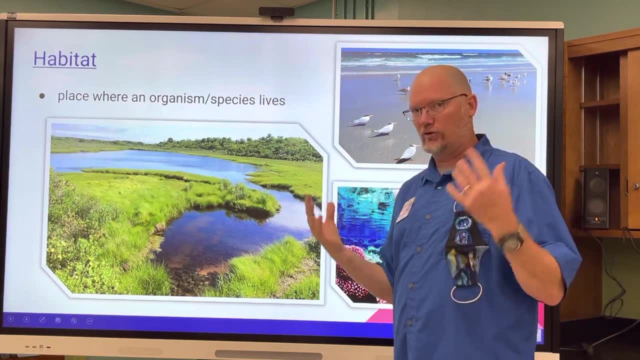 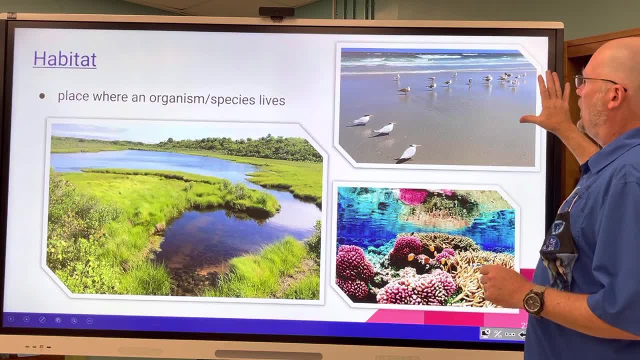 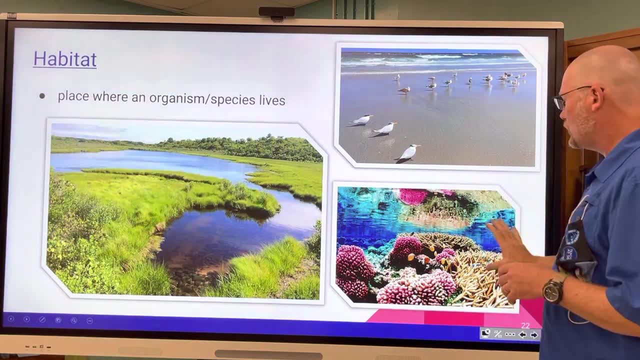 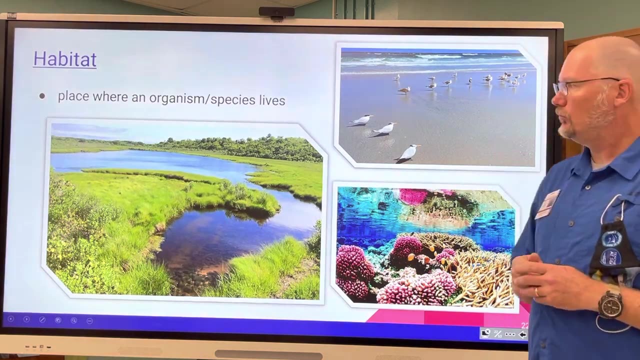 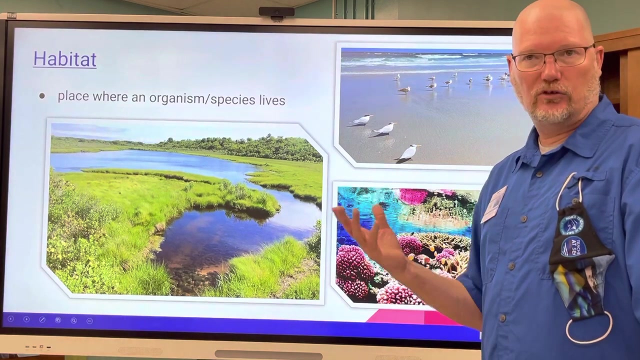 All true stories. by the way, This is a sandishore habitat, which we talked about in the last unit, And this is a coral reef habitat. All very different and with different environmental factors: non-living as well as living, different species of organisms. 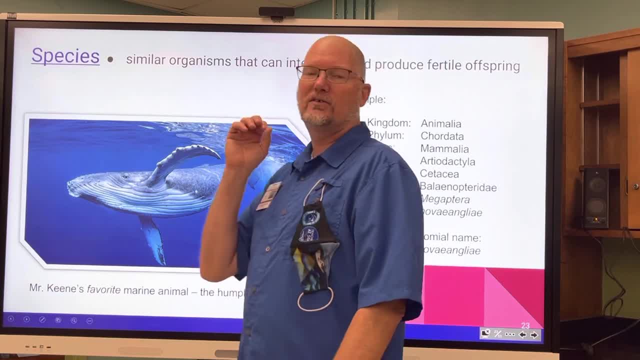 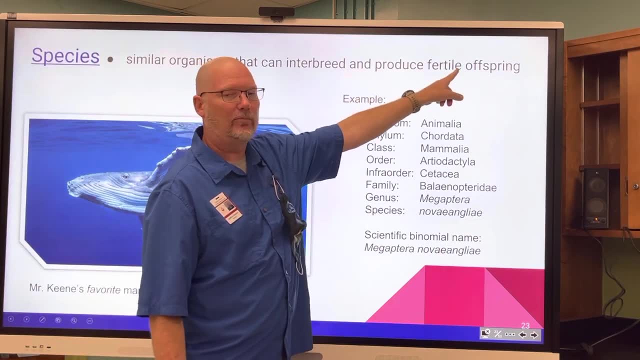 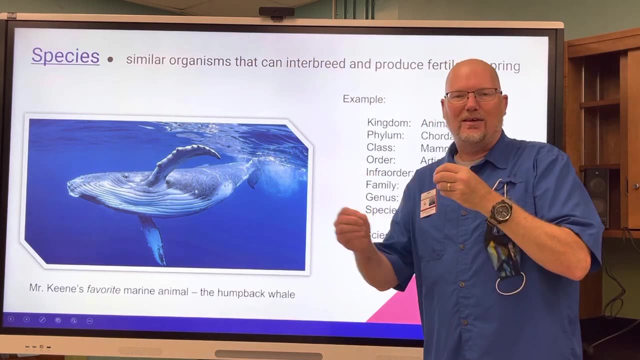 Speaking of species. species is defined as similar organisms that can interbreed and make viable, fertile offspring If two species come together and they're similar, but the babies they make can't make their own babies. that's what defines, that's the line that's drawn. 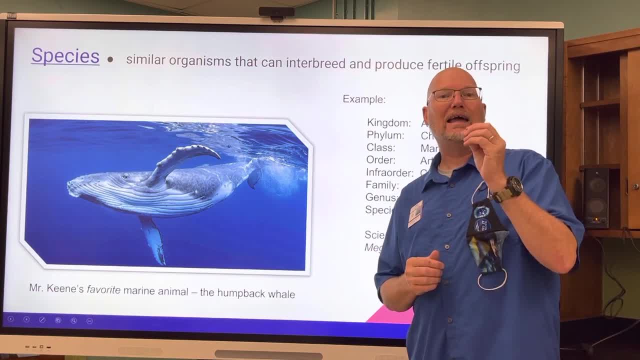 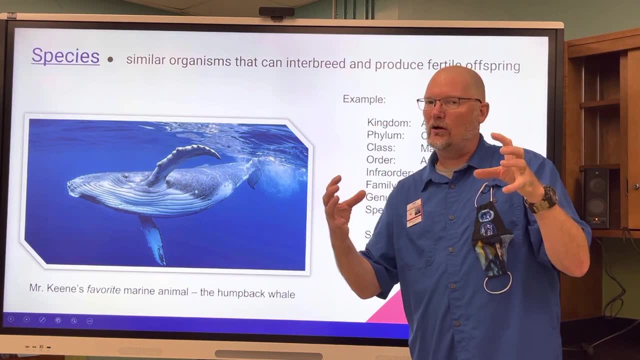 between two different species. okay, You may have heard of a liger, which is like part lion and part tiger, but a lion and a tiger are two different species that are separated far enough where they can have a baby called a liger. 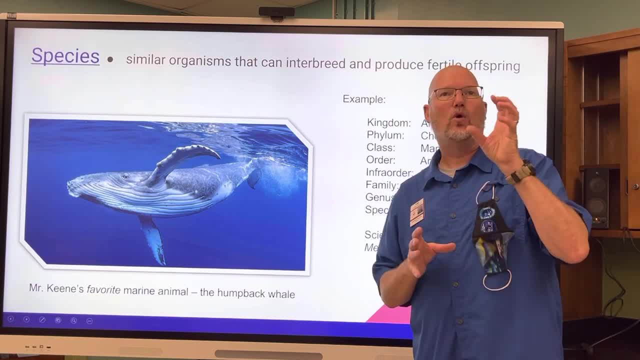 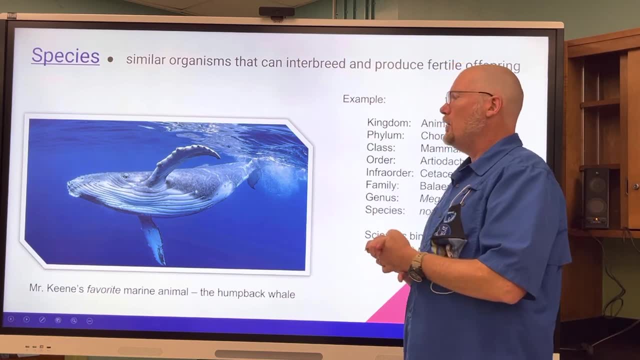 but the liger can't have babies, it's sterile. Same with a horse and a donkey: you get a mule. Mules are sterile, they can't have babies. okay. So an example of a particular species, and my favorite, dearest to my heart, is the humpback whale. 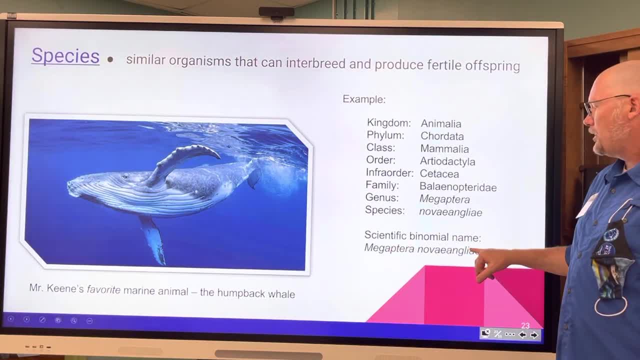 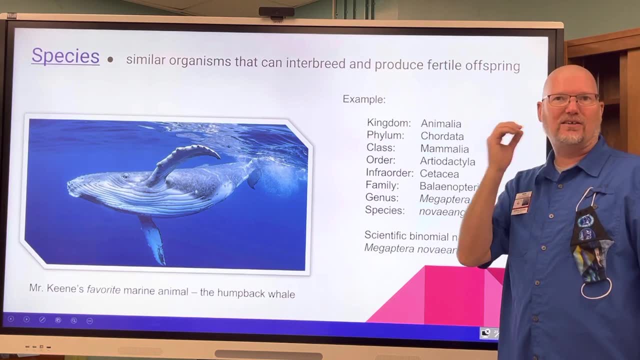 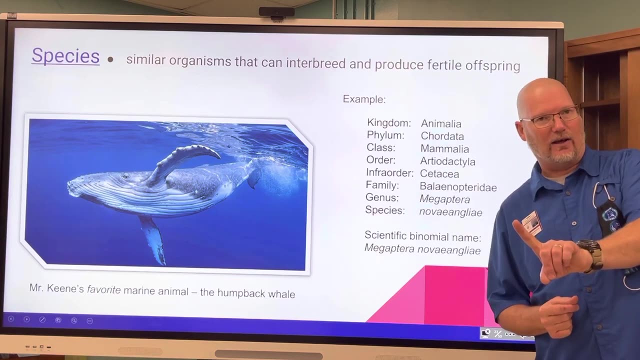 Okay, so your job is to write down the scientific name properly. not all this, that's just the taxonomic classification, but this is a scientific name and a proper way to write it. I know some of you are writing- I'm writing it right now, so be careful. 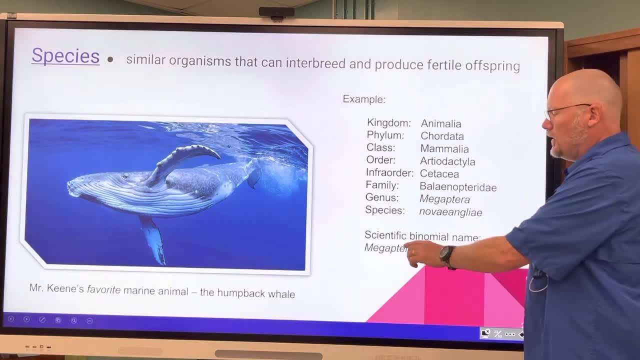 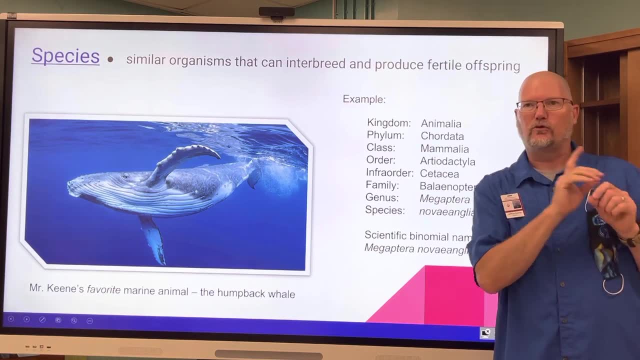 you may have to erase what you just wrote or cross it out. if you're writing in pen, When you write or when you type a scientific name, it must be italicized. So if you're typing this, that's easy. If you're writing it, you can't italicize. 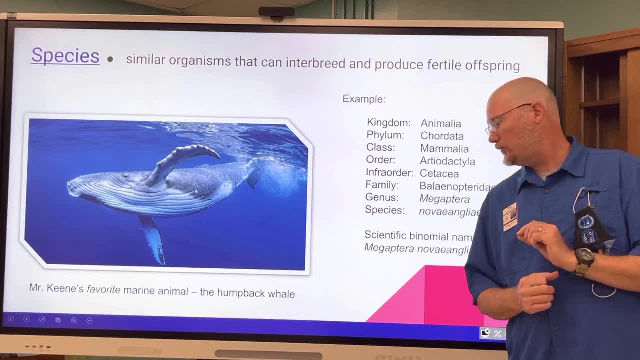 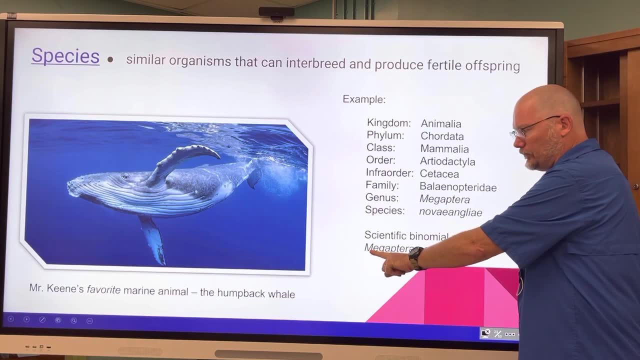 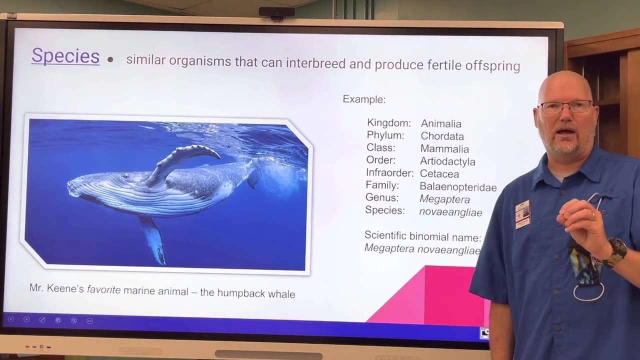 because everything's italicized. The rule for writing a scientific name is to underline it, and both ways, typing or writing the first letter, which is the genus, the first is always, always capitalized, the second one. I see this mistake all the time in movies and books. 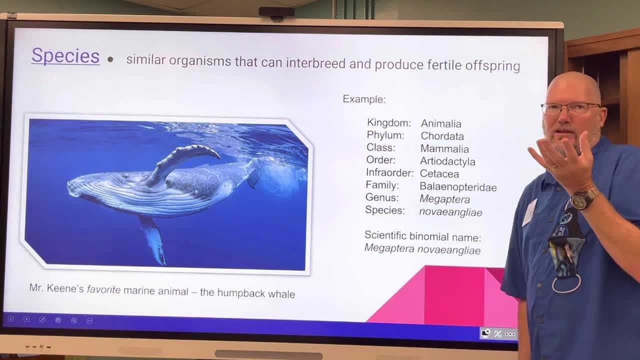 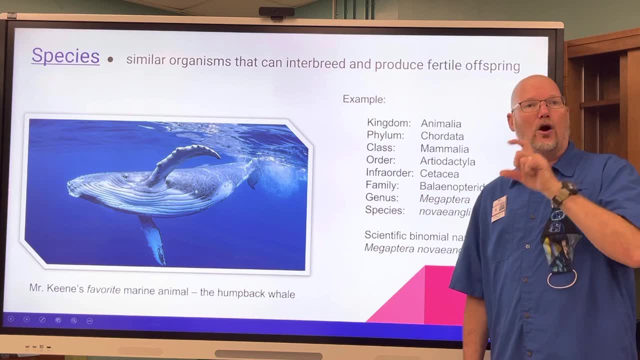 and magazine articles because they're not scientists. right Is lowercase. this is the proper way to write a scientific name. So if you're talking about humans, homo sapiens, the H in homo would be capital, but the S in sapiens would be lowercase. 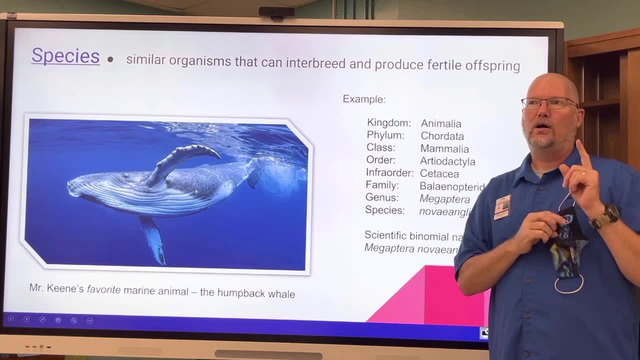 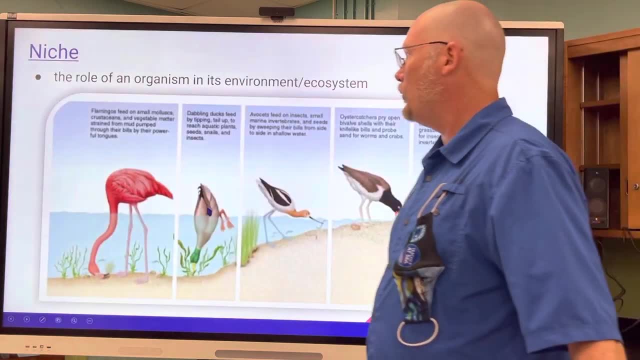 and it would be all italicized. if it was handwritten, it would be underlined. So I'm gonna be checking for that when I check these notes. make sure you do it right, okay. And then, of course, the common name is the humpback whale. 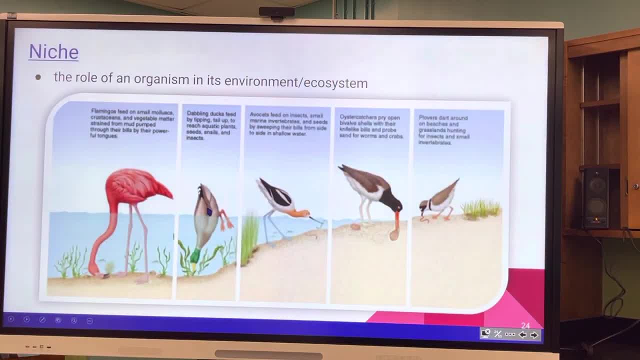 Okay, what's a niche? You could say niche, you could say niche. I prefer the term niche, actually, but a niche is an acceptable way to say it. You may have learned that, So you just have to pick one of these. 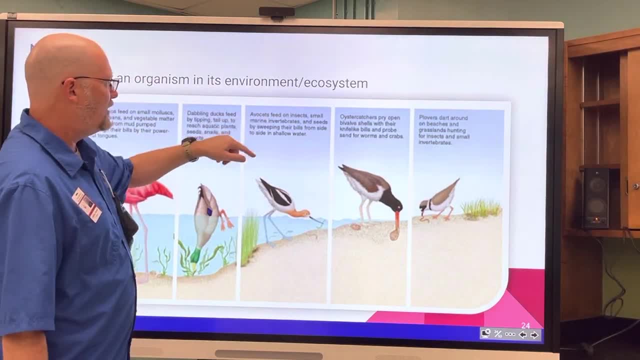 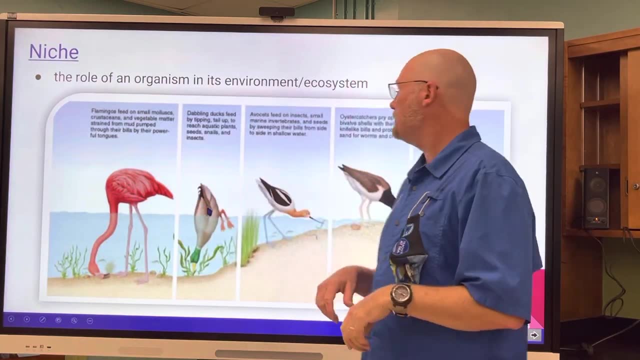 the flamingo, the duck, the avocet- it's hard to read because it's fuzzy up here too. an oyster catcher, one of my favorite birds, okay. Or a plover, those little tiny birds that run around the beach, okay. 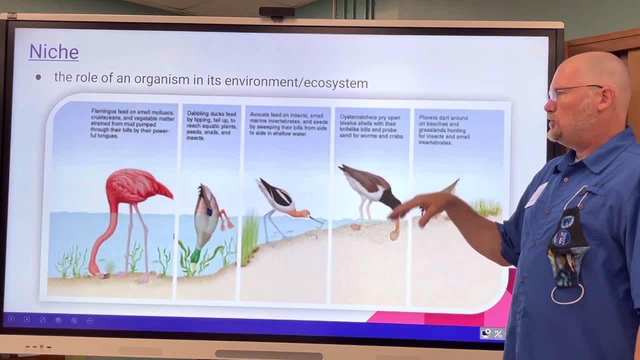 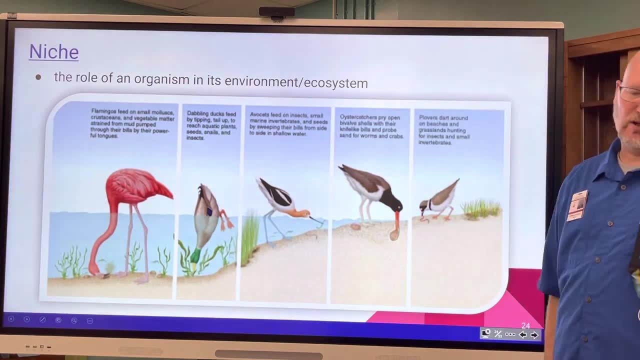 Oyster catchers. you might not typically see on the beach, you might see those further like more inland, like in the estuary. okay, Anyway, pick one of these as your example And they all occupy a role, a particular role, in. 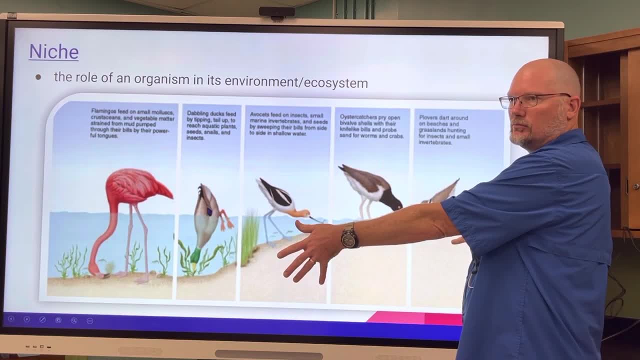 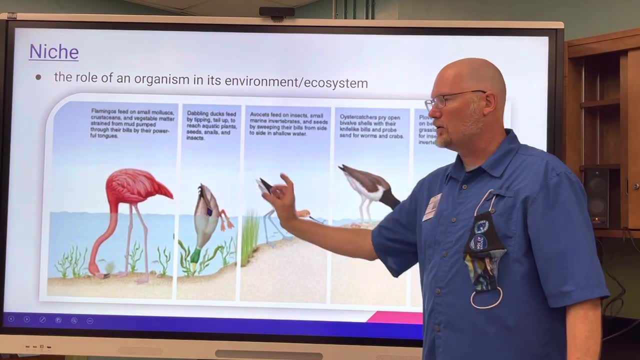 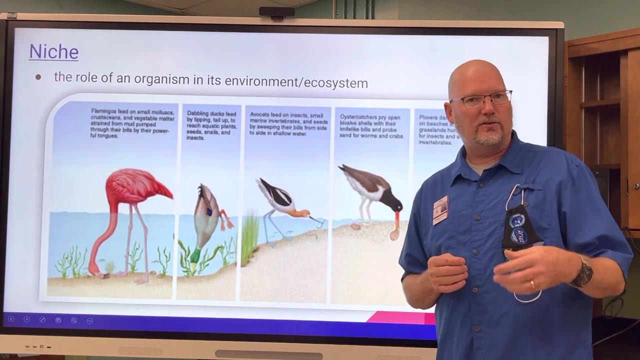 so these are all in the littoral zone right Of a shoreline, but they all occupy. they all occupy a role in the littoral zone, So they're not competing with each other, And that's what a niche is. You may have heard of niche as a niche market in business. 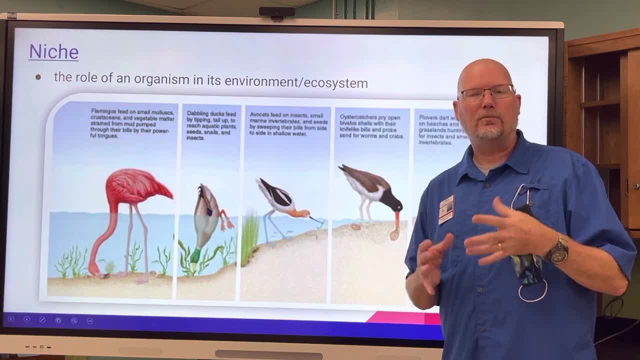 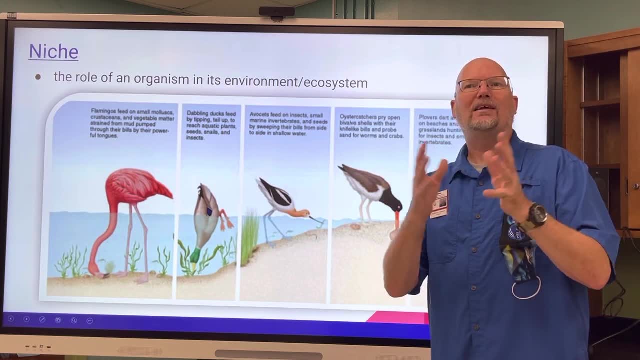 or a niche business concept where, if you're gonna open up a business somewhere, make sure that you are able to provide what nobody else can provide. so there's no competition, And that's what's happening here. There's no competition in those different areas. 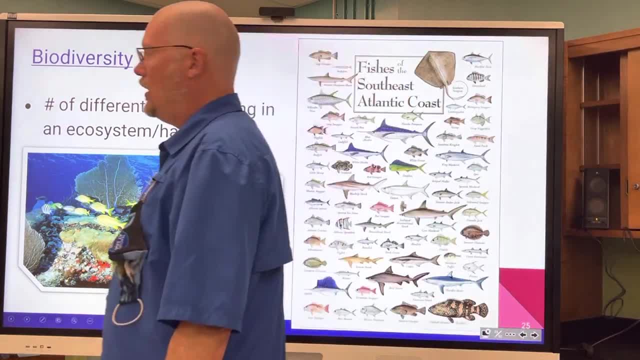 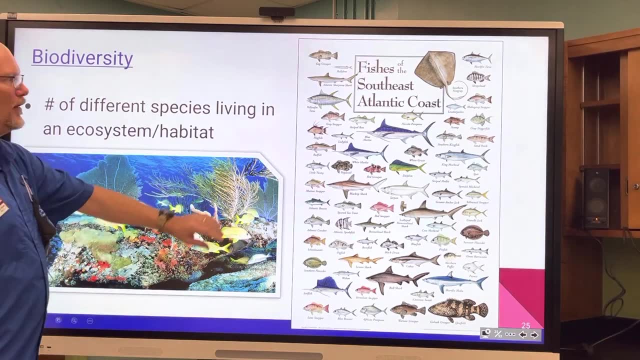 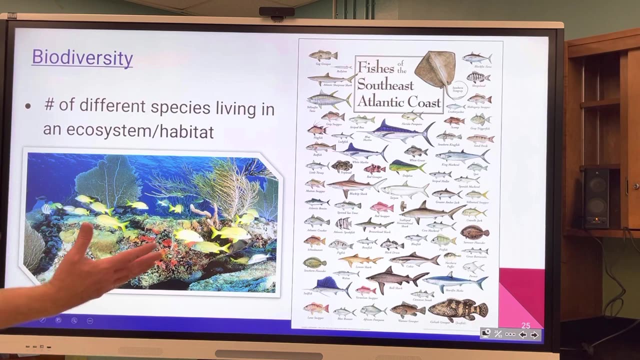 or little competition. Biodiversity. Biodiversity is the number of living things in an ecosystem or a habitat. So these are the fishes of the southeast Atlantic coast When you go out in the water, in the ocean, and off of Florida, off of Boca Raton. 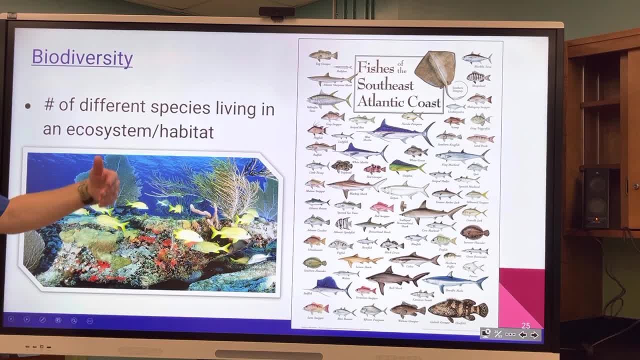 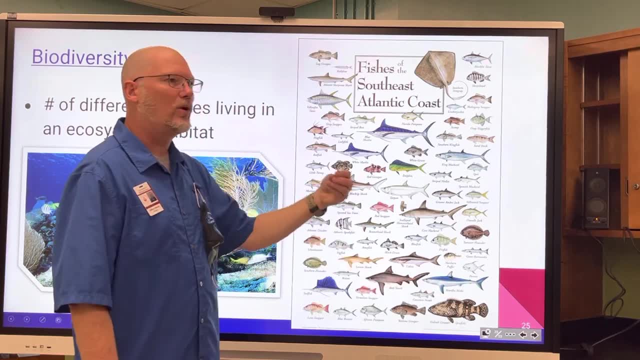 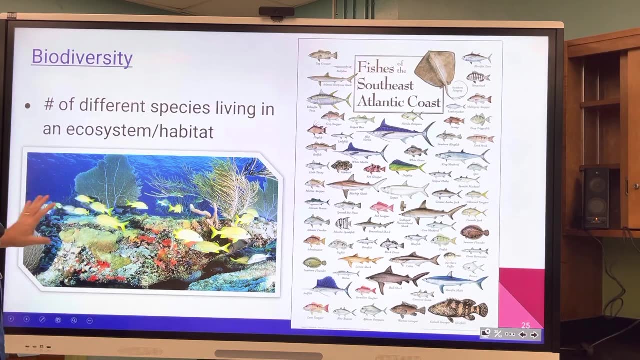 these are the fish that you would probably be able to find, plus a lot of others. okay, So the more there are, the more different species there are, the more biodiverse a region is, a habitat, an ecosystem is, And, of course, a coral reef is known to be. 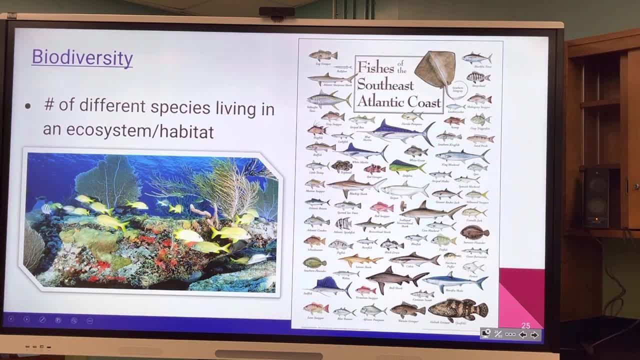 one of the most biodiverse ecosystems in the world, as well as, like perhaps, the Amazon rainforest or even estuaries, are extremely biodiverse. Okay, population. we're gonna go really quick now because we only have a couple minutes left. 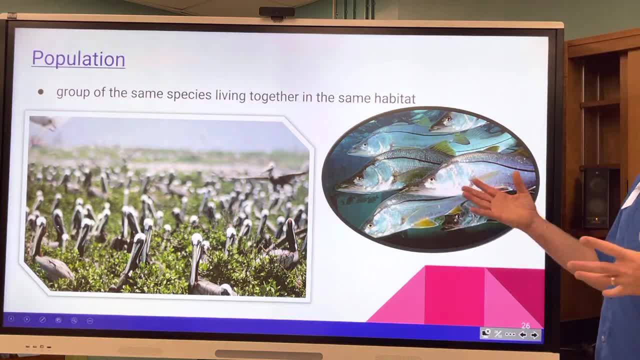 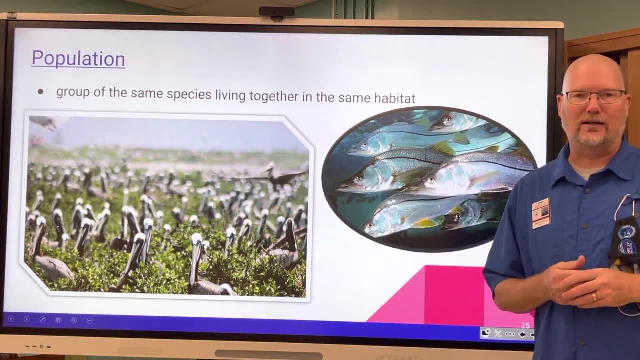 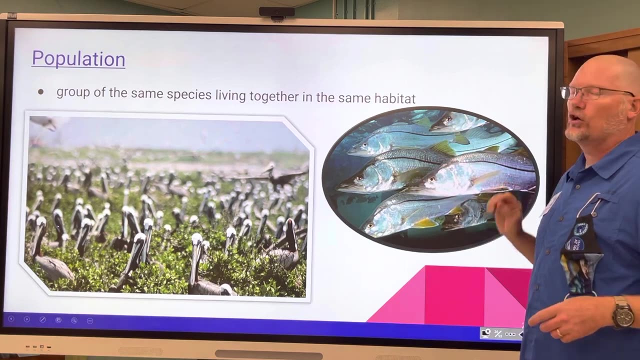 before class is over. A population is a group of the same species living together in the same habitat. So here we have a population population of brown pelicans. Yes, only the front is focused, the rest is out of focus. Here you have a population of snook. 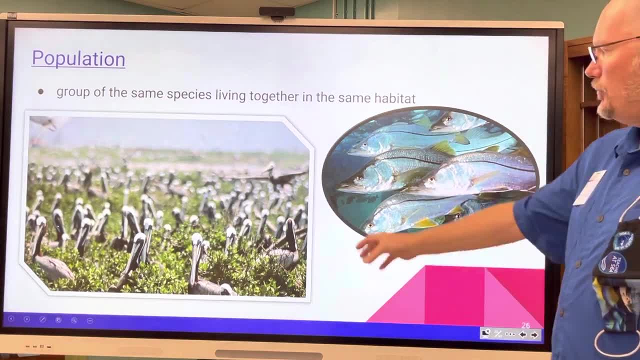 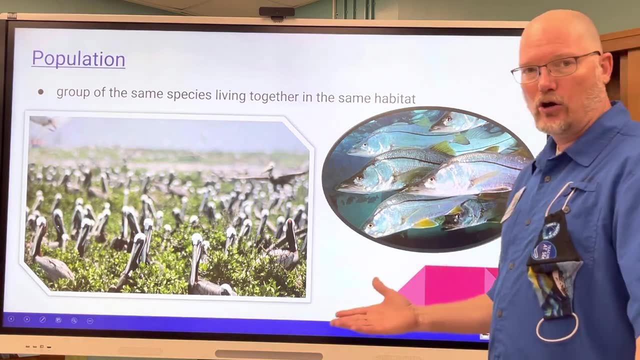 maybe right off the coast here, okay, The pelicans would be breeding inland. There's quite a few parks around here that have bird breeding- marine bird breeding habitats right around here, within a few minutes drive. I've been to them. 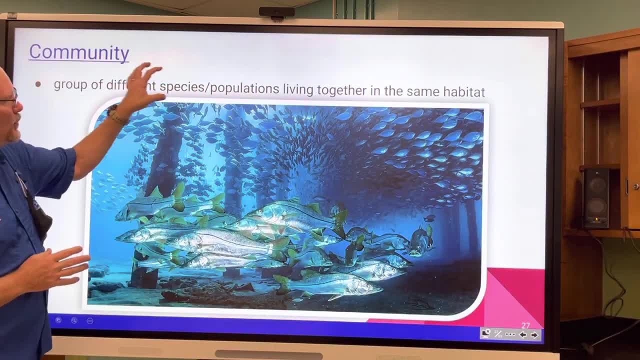 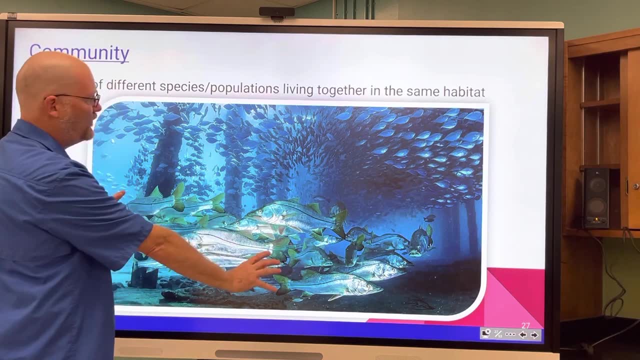 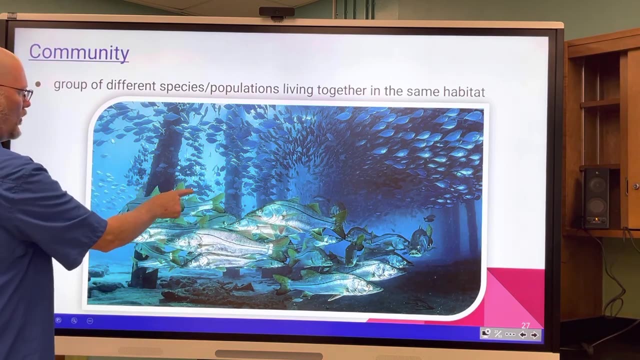 And then a community is. you take groups of different populations and you put them in the same habitat. So here you have those snook that I showed you before, but then you pull out and you see the other populations of other fish. So you've got different species of fish over here. 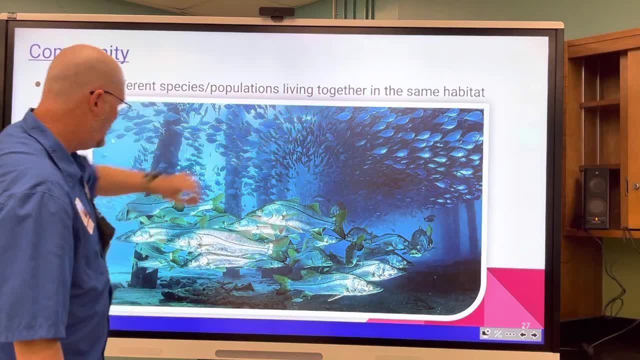 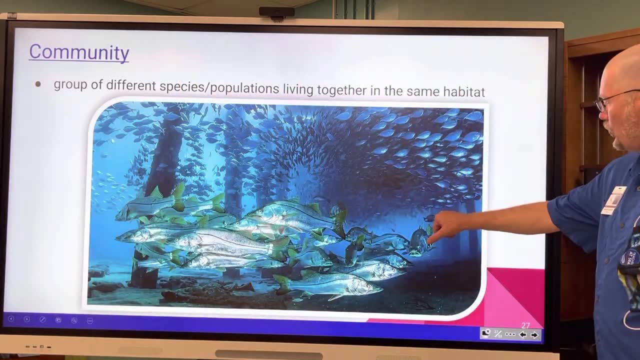 going around the poles and different species of fish in this bait ball, And then, if you look closely, you might actually see some other species wandering around somewhere that don't quite fit in with the other ones. okay, So different populations is a community. 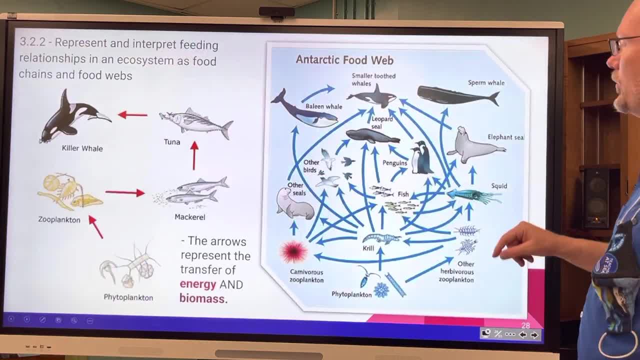 And then let's see. that's our last slide. So good, we're almost done. So the arrows again represent the energy transfer and something called biomass, which we're gonna talk about in the next part of this notes. So you have to know how to interpret a picture like this. 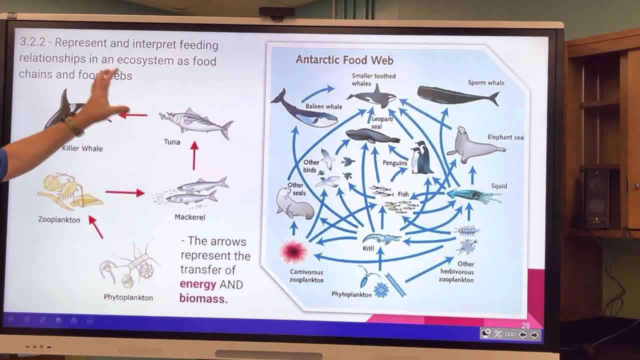 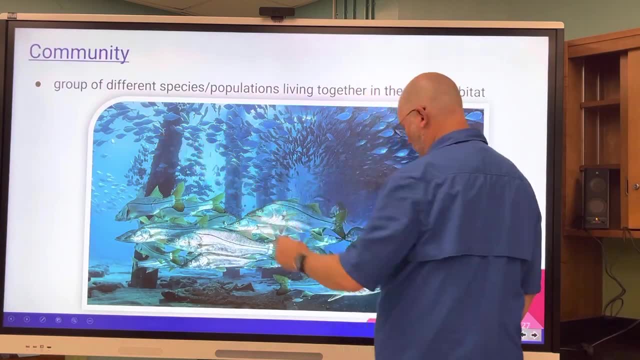 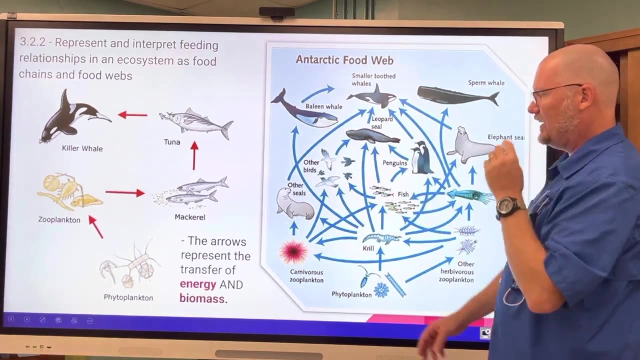 okay, What's eating? what? Where's the energy going? You would have to be able to trace a food chain- sorry, a food chain- in a food web, So I could pick. I could you know I pulled this out of this. 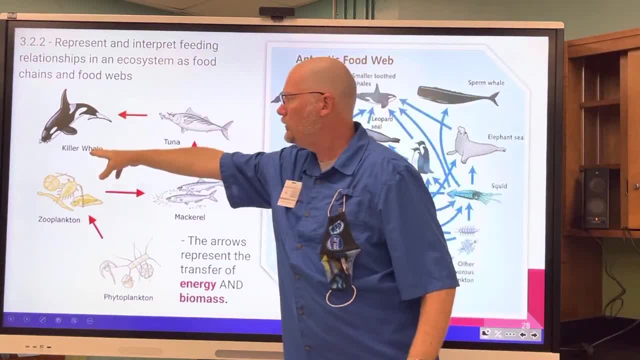 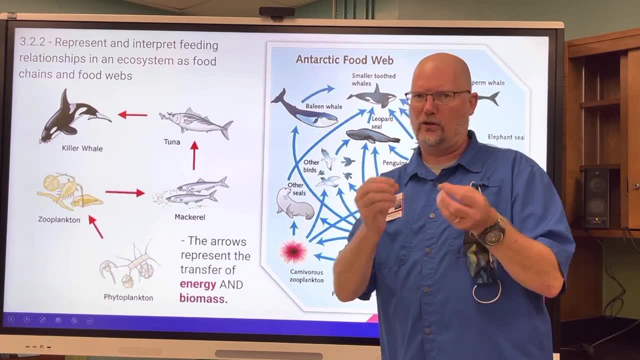 cause. you see the orca whale. it's not really a killer whale- People call it that, but it's an orca whale. You don't call a lion a killer cat or a wolf a killer dog or us killer humans, cause we eat meat, right. 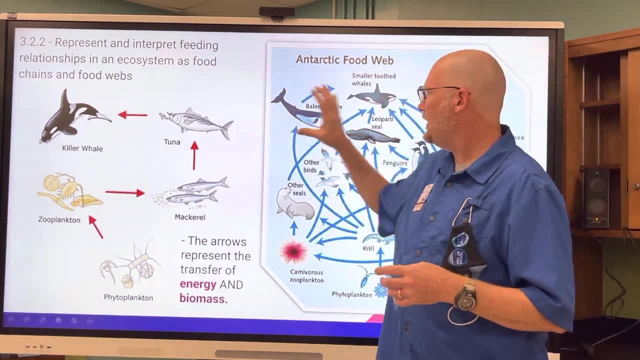 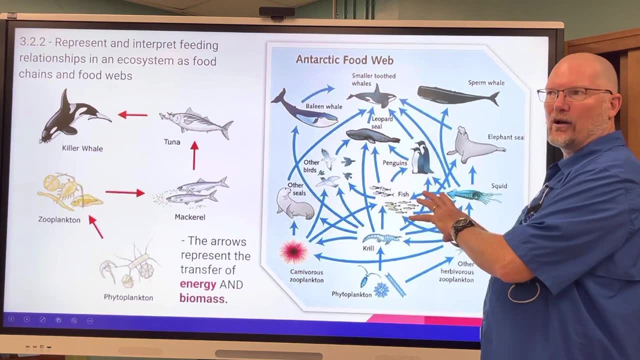 So it's an orca whale Anyway. so you can pull it out and you can make into. you can make multiple different food chains from a food web, And so you just have to know how to draw one, how to pull one out like trace it up. 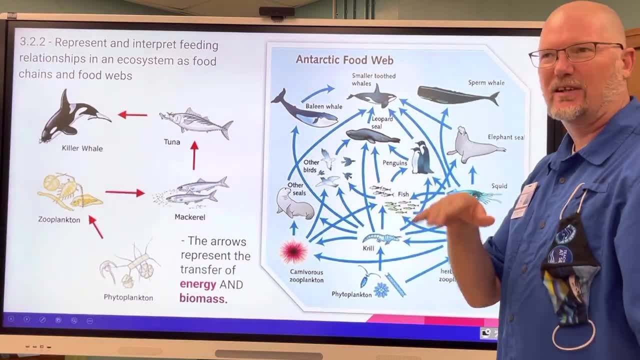 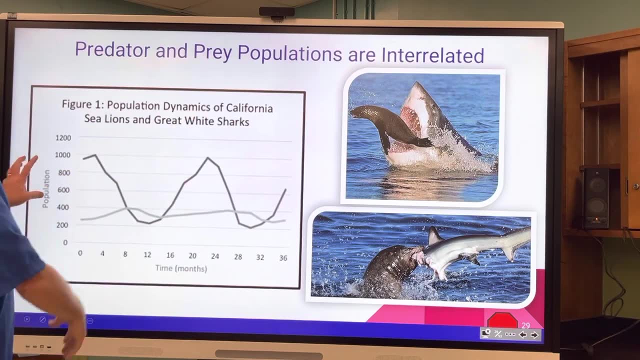 and know how to read one, okay, And we're gonna have a little bit of practice on that in the future. And then, finally, predator and prey populations are interrelated. So this is in your notes. All you have to do is answer a couple of questions about this.